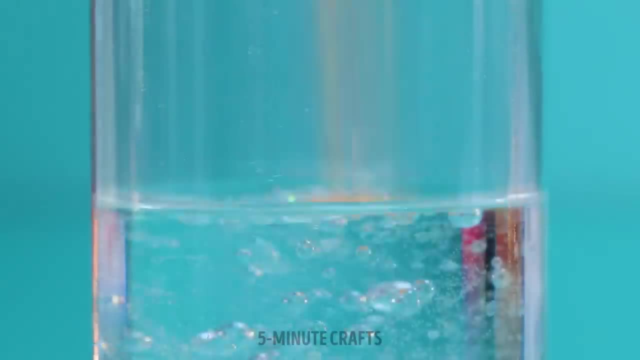 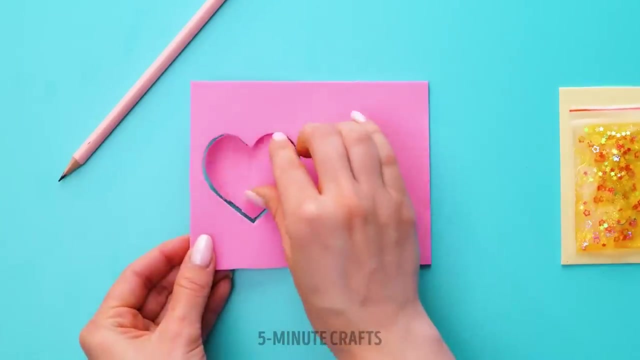 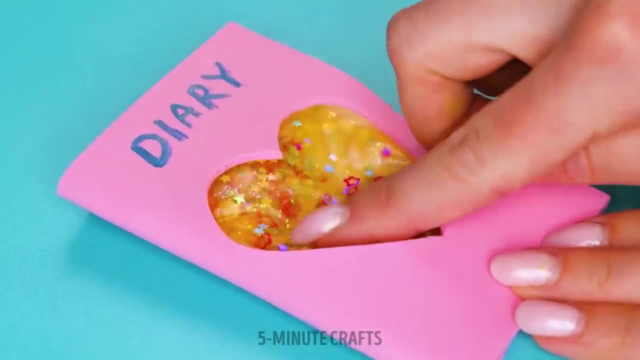 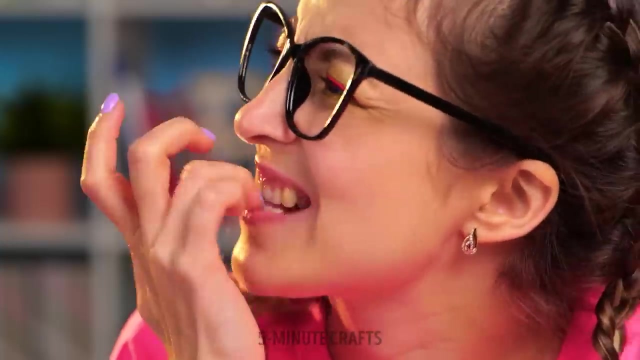 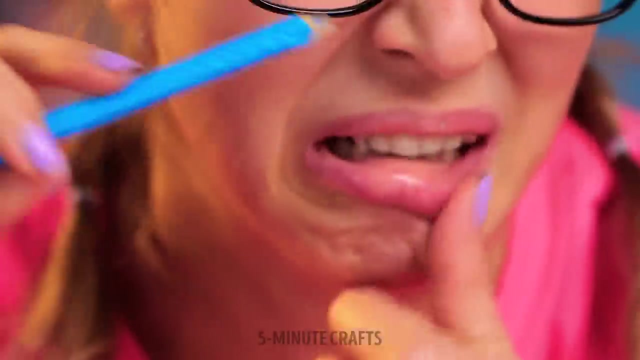 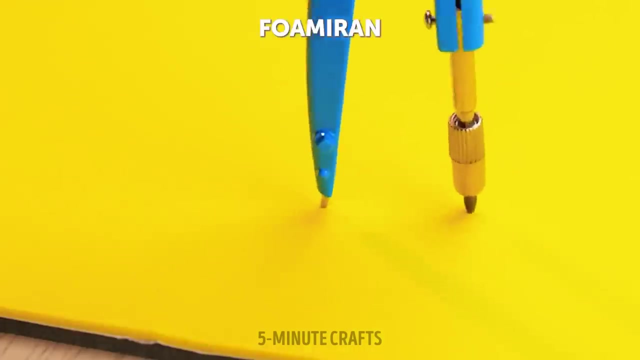 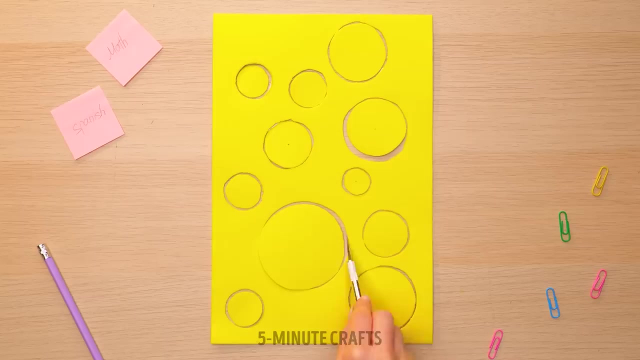 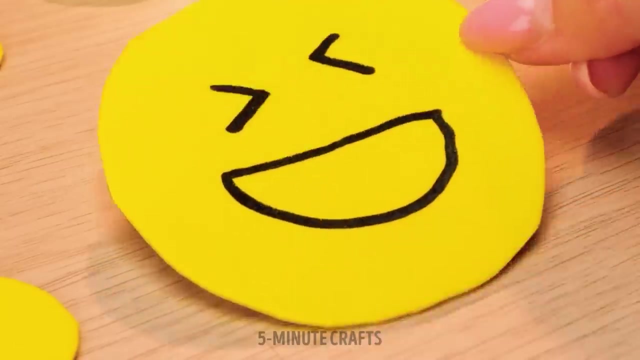 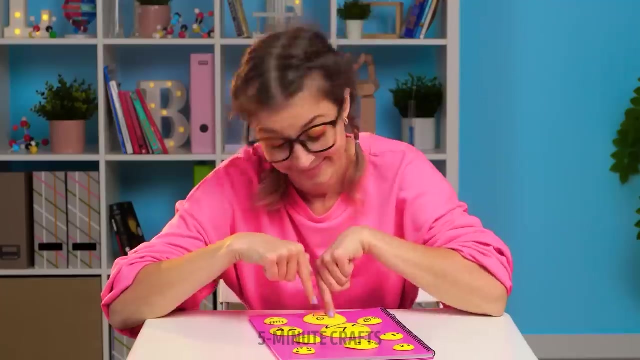 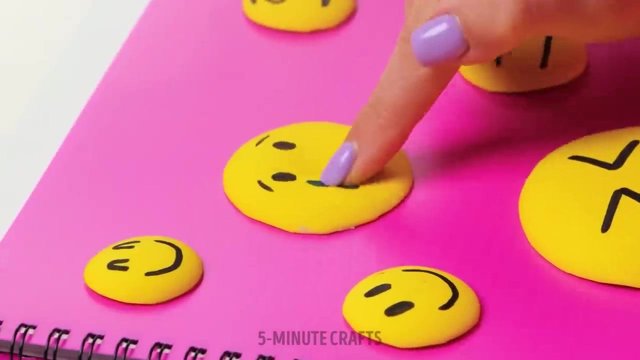 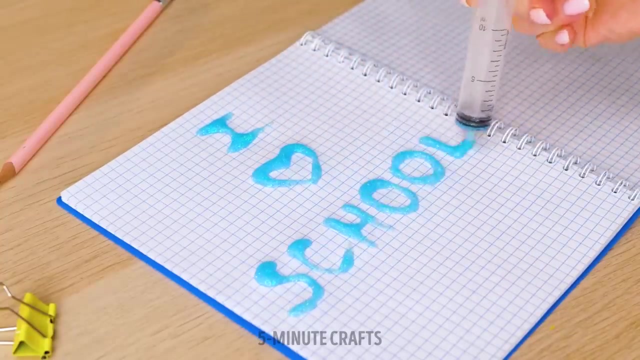 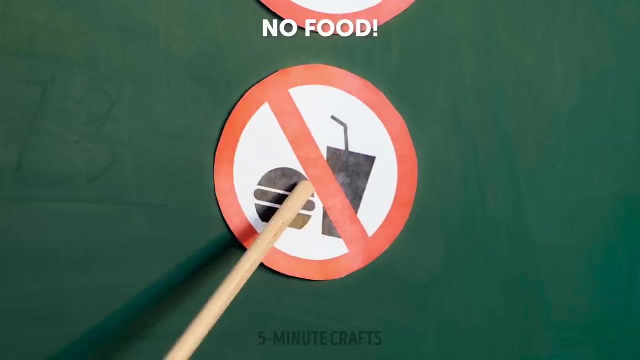 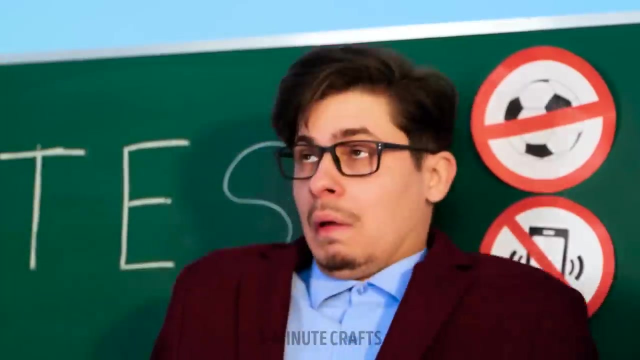 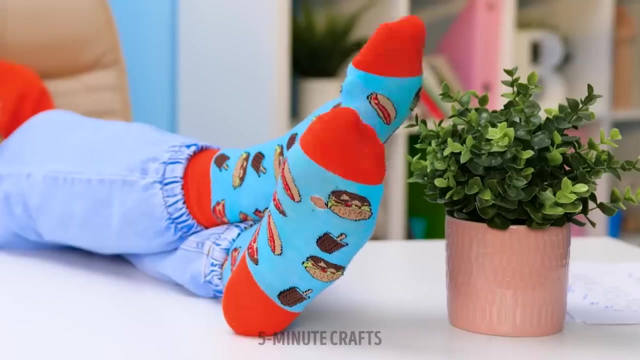 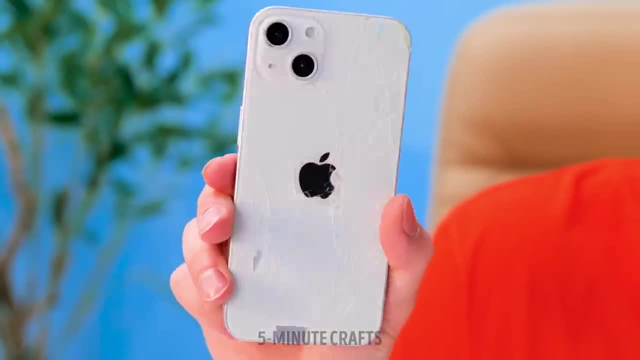 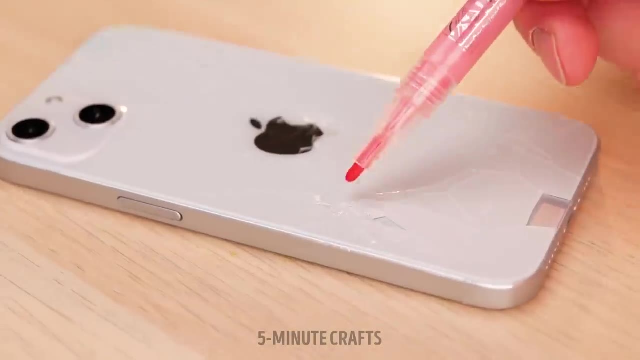 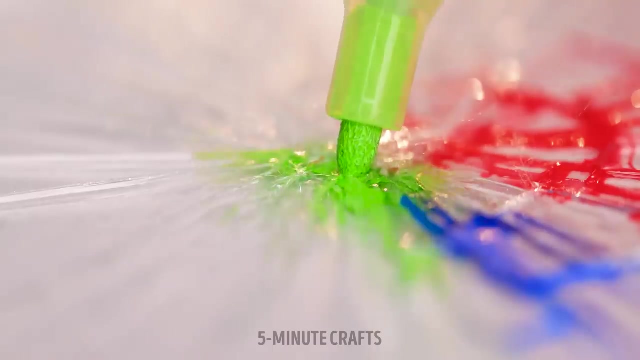 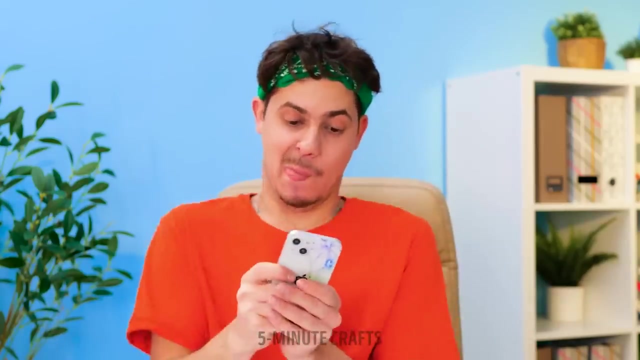 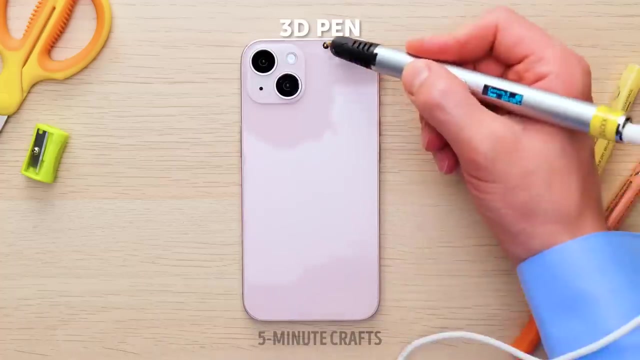 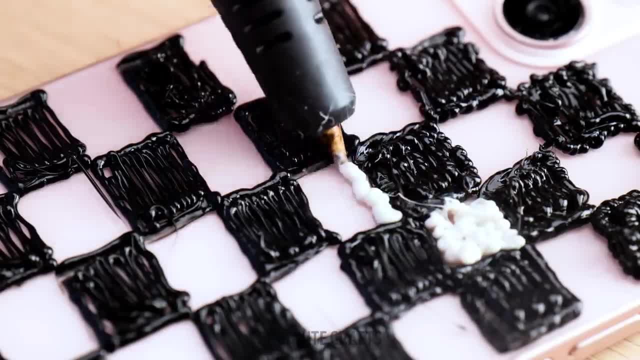 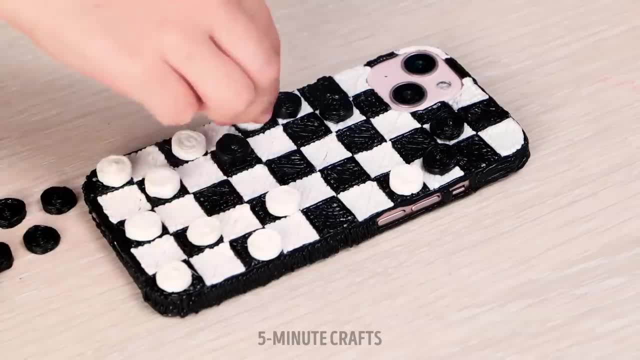 Maybe you're not too afraid, Maybe you're not too afraid, Maybe you're not too afraid. Yeah, yeah, yeah. Oh baby, here's one. Oh, yeah, here's one. Oh, baby, here's one. Oh, yeah, here's one. 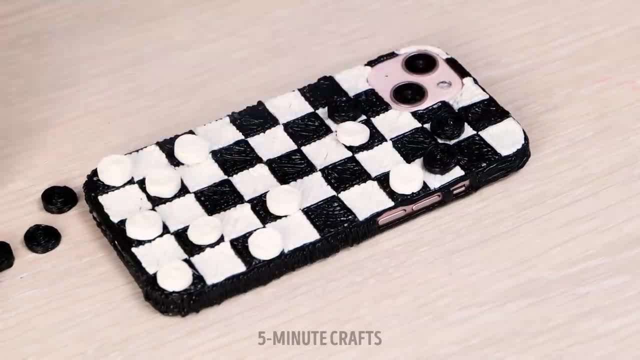 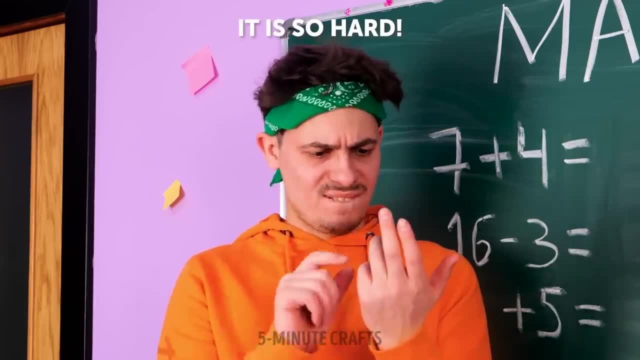 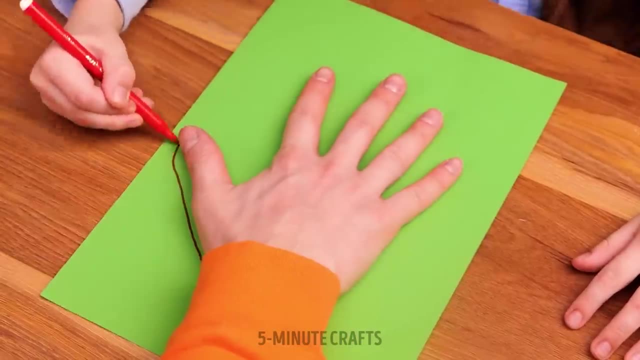 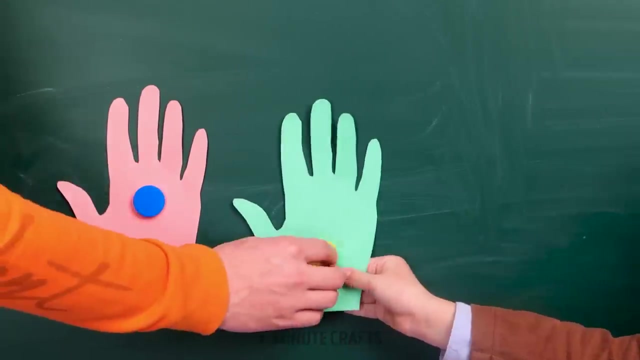 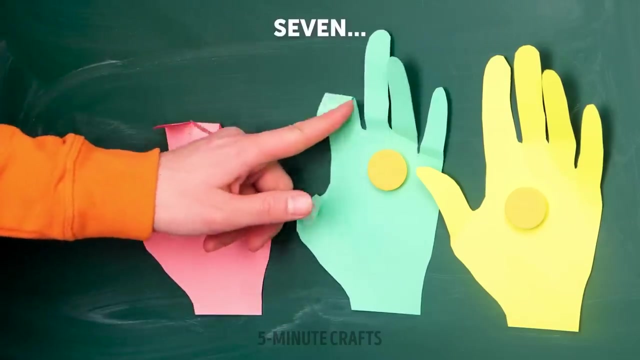 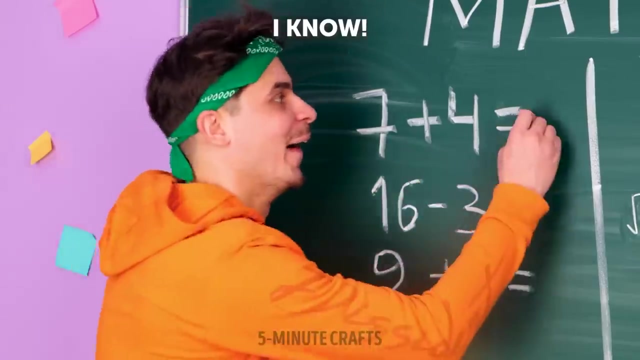 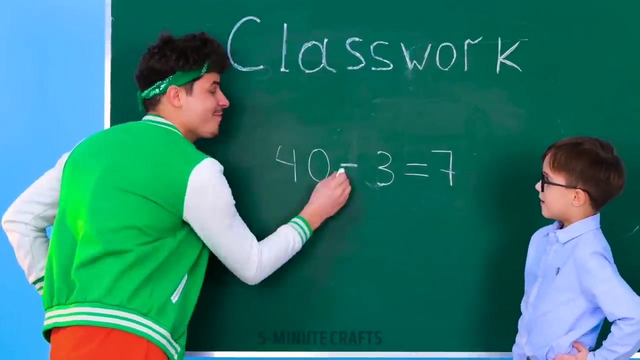 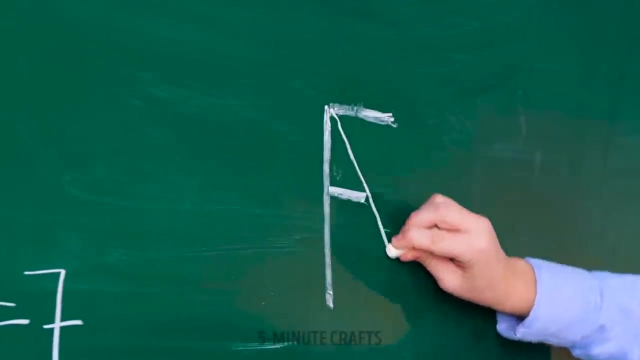 Oh baby, here's one. Oh, Oh baby, here's one. Oh, Don't look back. Oh baby, here's one, Don't look back, Come on tonight, Come on tonight. Mama always used to say: you'll find another. Endless love is coming. I'll be sure of that. 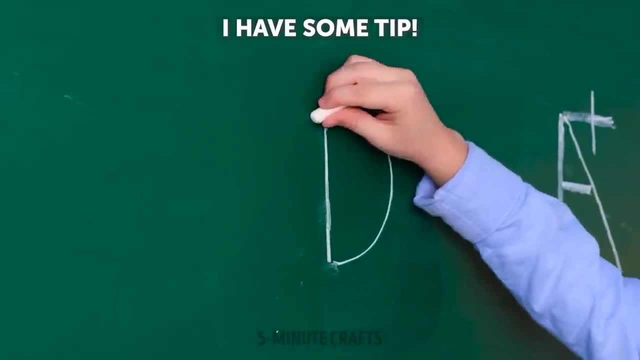 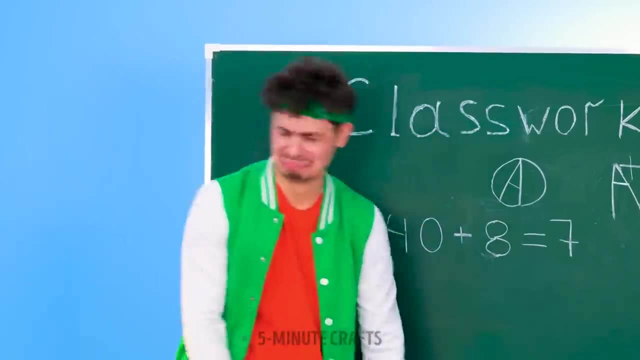 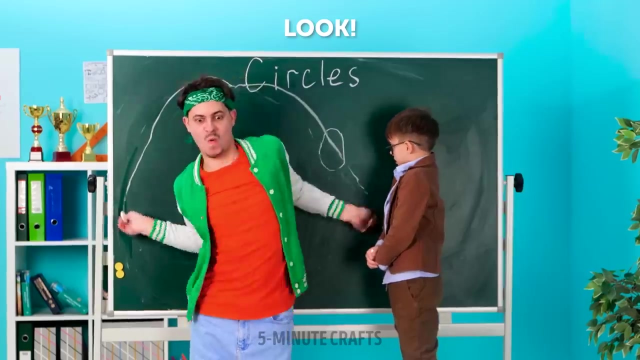 But it's so hard Cause it's you. it's you always on my mind. Yeah, it's you. it's you taking all my time. Let it sink in. haven't you been hurting enough? I give you all of my love, but you don't seem to care. 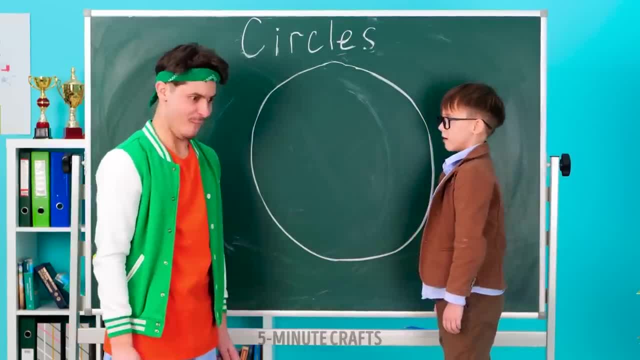 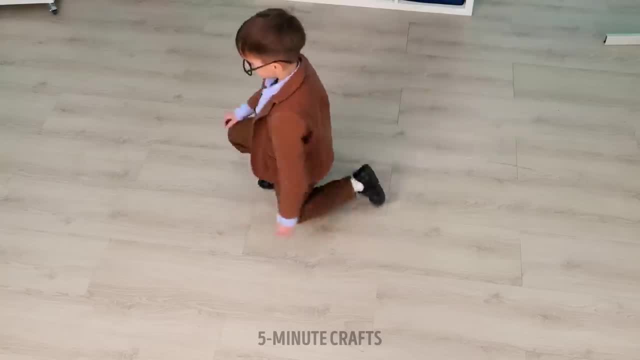 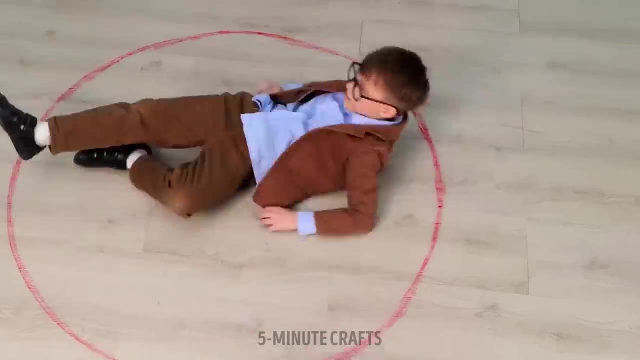 But my heart's around you, but your heart isn't there. Don't tell me, we're fine lying to yourself. It's so late to meet up, we are too far apart. It's so late, can't you see? I can't trust you no more. 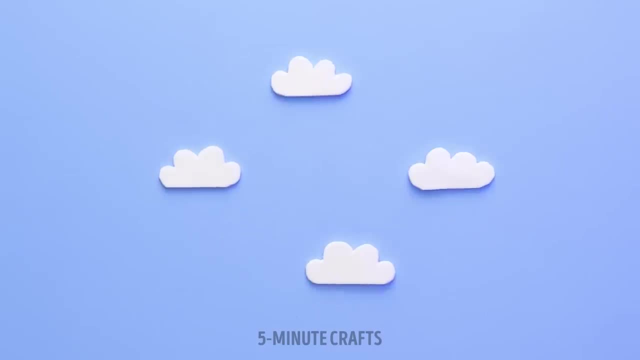 Gotta get over you, cause I'm more than the dark. It's so late, can't you see? I can't trust you no more. It's so late, can't you see? I can't trust you no more. It's so late to meet up. 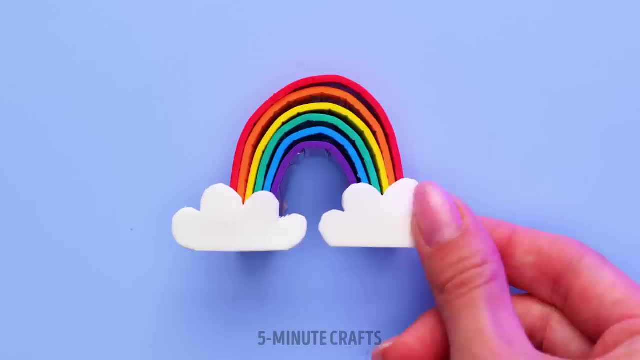 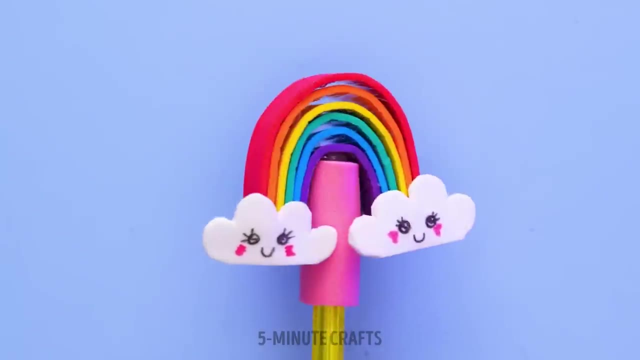 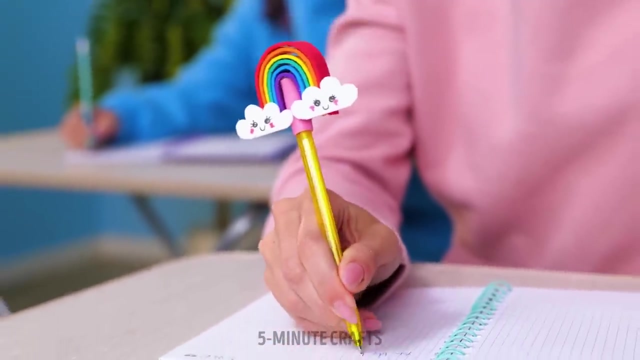 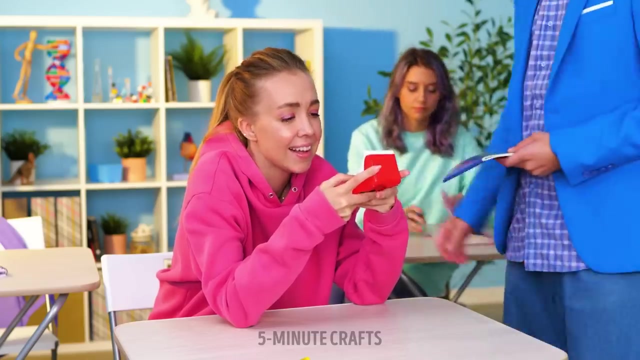 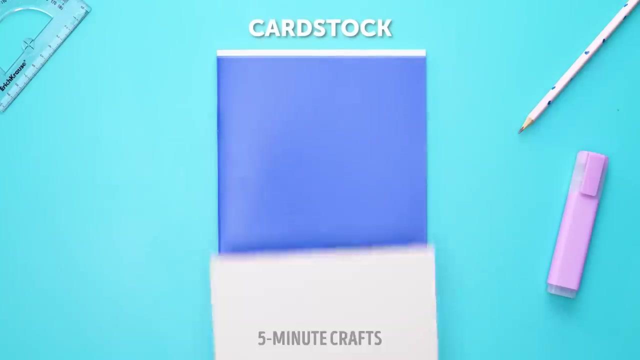 Don't go there, cause you can't finish what you start. I can't keep up. You're holding back and then you let go. Don't let it go too far, just stay away, Cause it's you. it's you always on my mind. 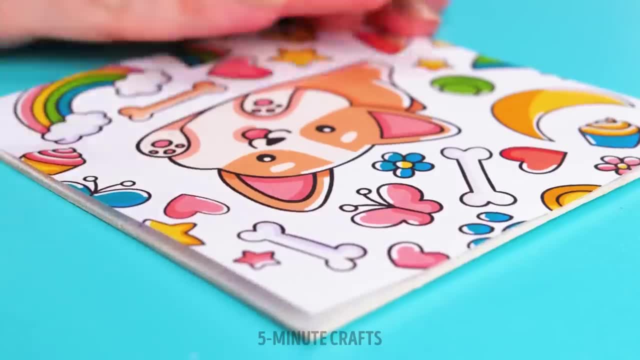 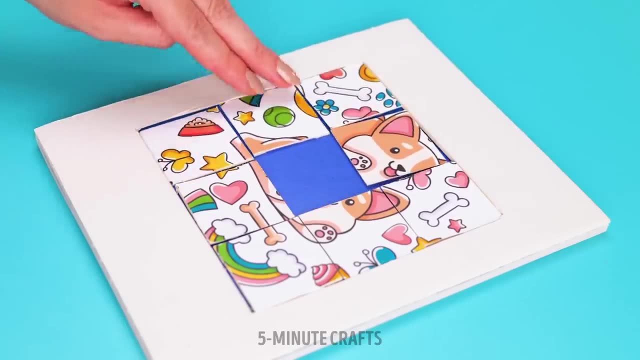 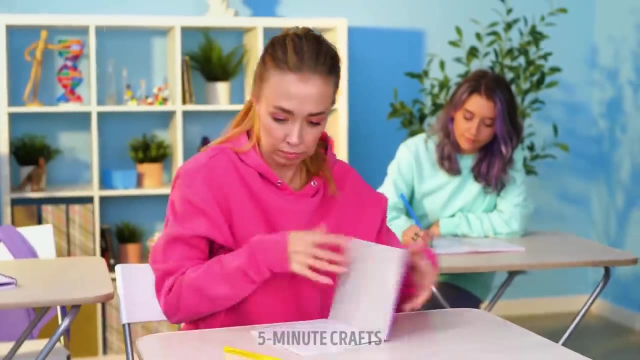 Yeah, it's you. it's you taking all my time. Let it sink in. haven't you been hurting enough? I give you all of my love, but you don't seem to care. But my heart's around you, but your heart isn't there. 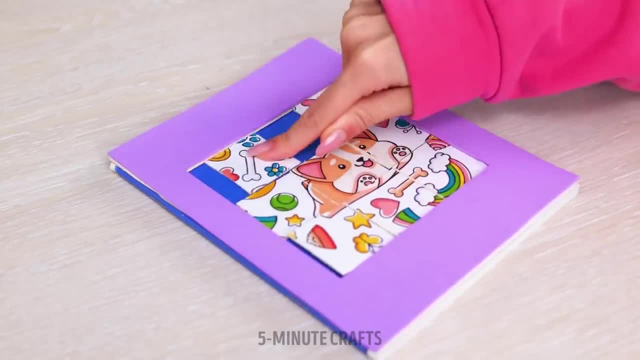 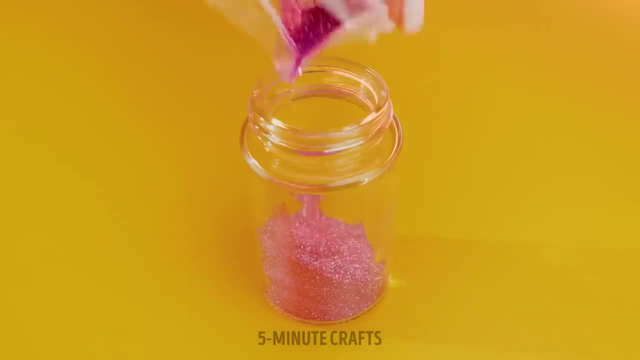 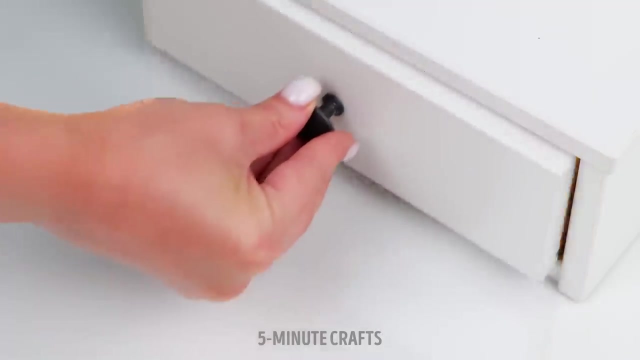 Don't tell me we're fine Lying to yourself. It's so late to meet up. we are too far apart. It's so late, can't you see? I can't trust you no more. Gotta get over you, cause I'm more than the dark. 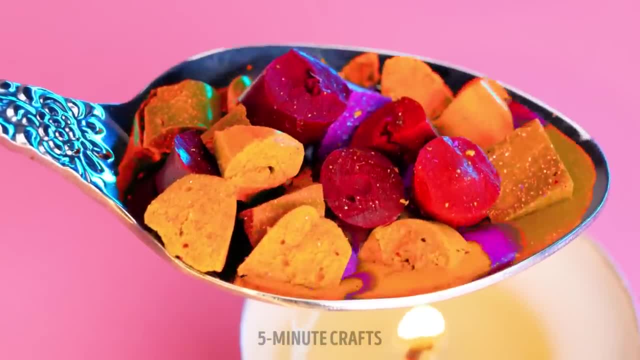 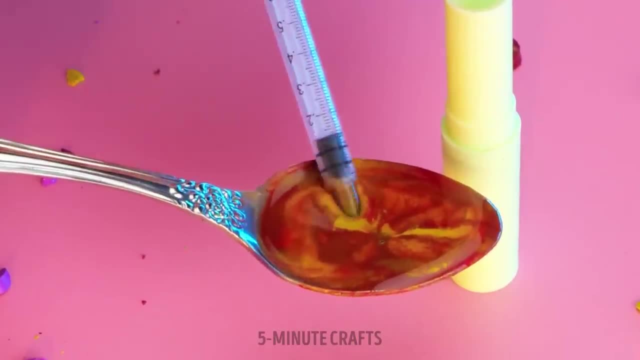 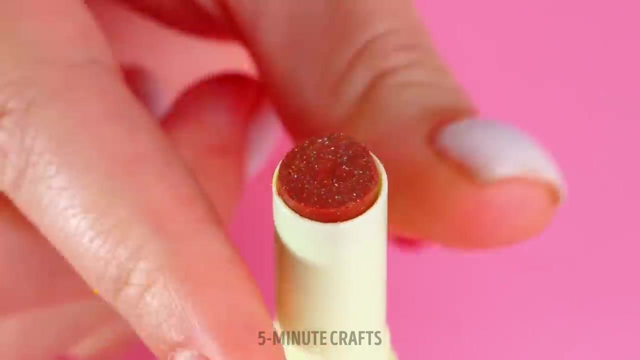 It's so late to meet up, Too late to meet up, Too late to meet up, Too late to meet up. Oh, gotta get over you, cause I'm more than the dark. It's so late to meet up, Too late to meet up, Too late to meet up. 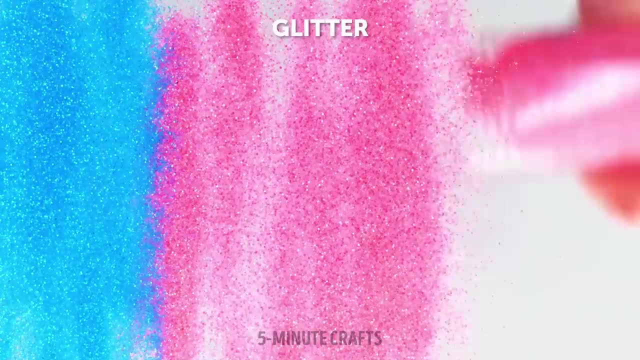 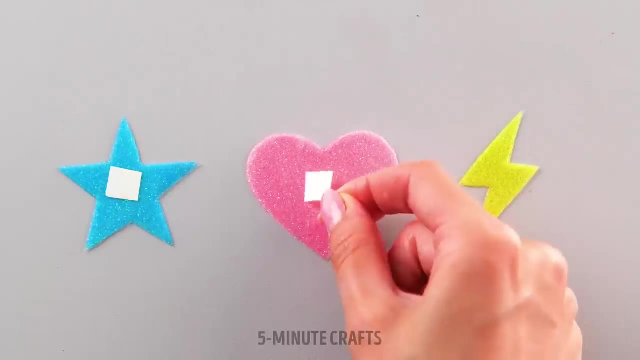 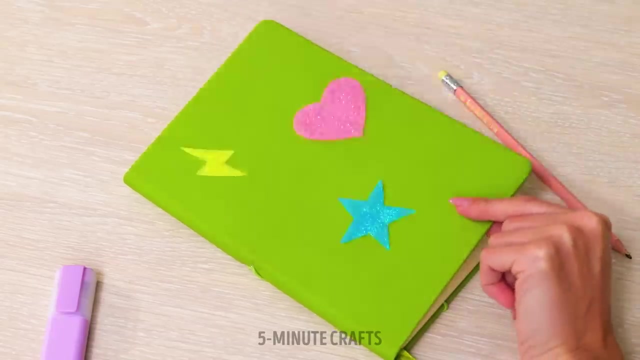 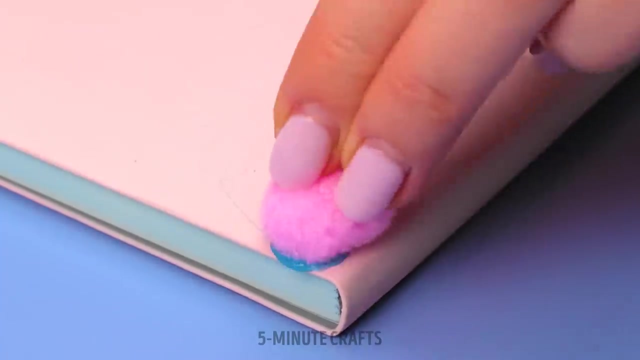 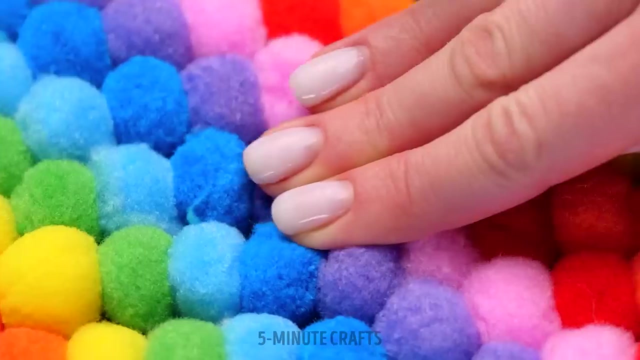 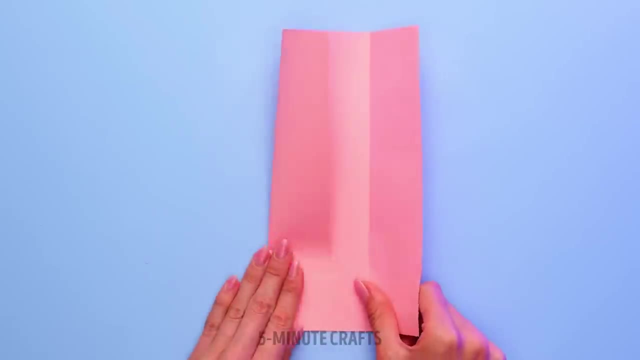 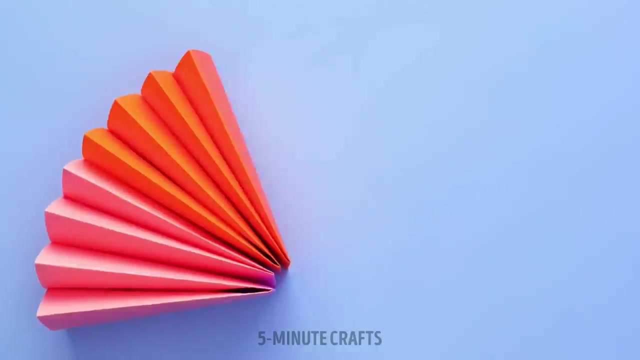 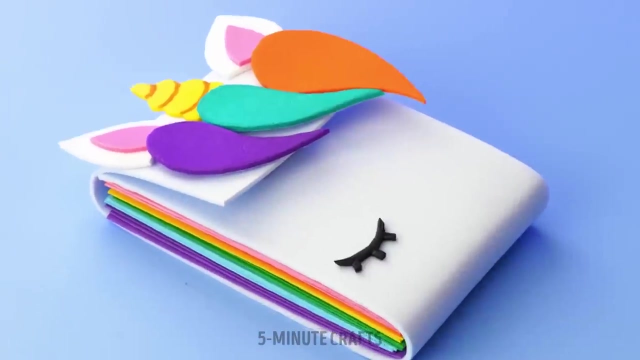 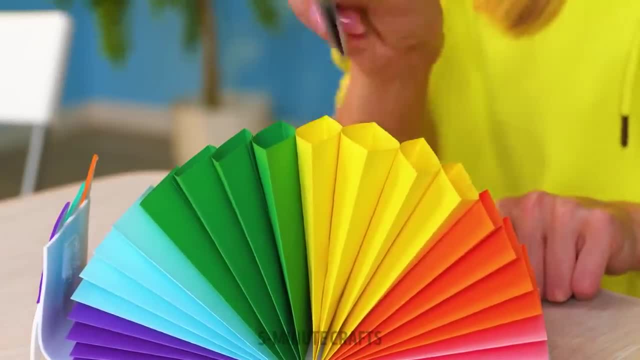 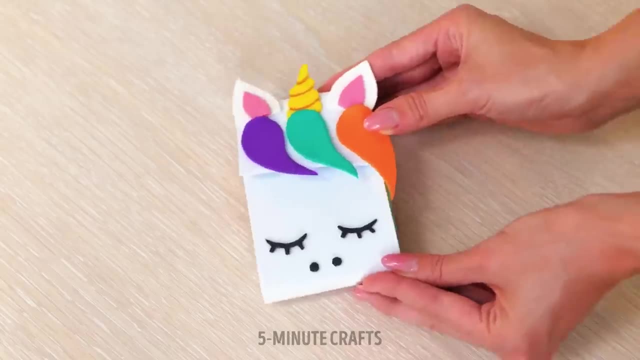 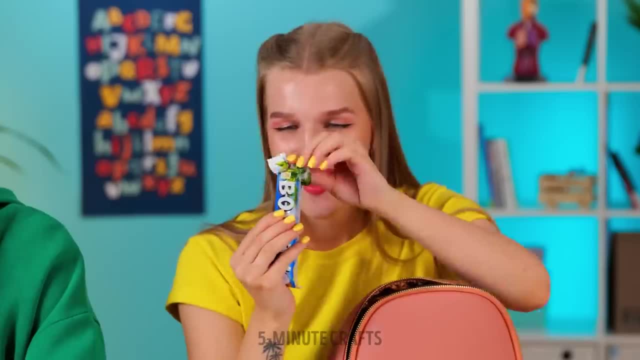 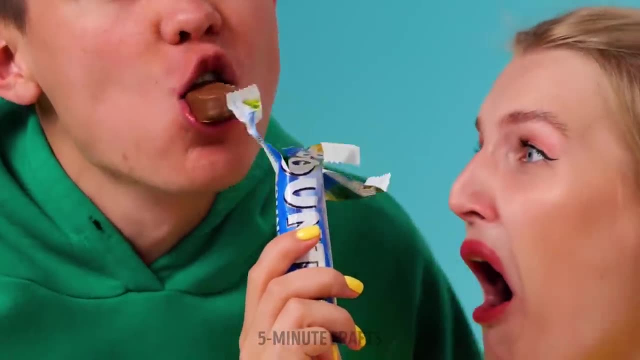 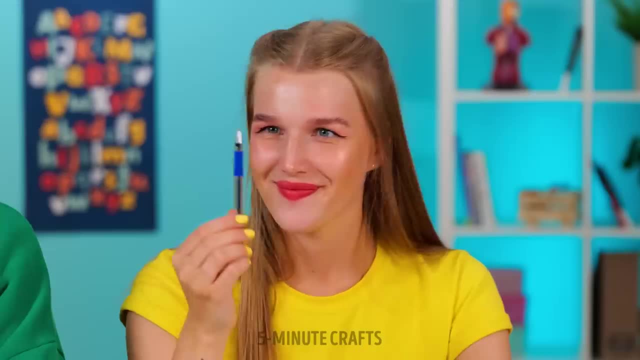 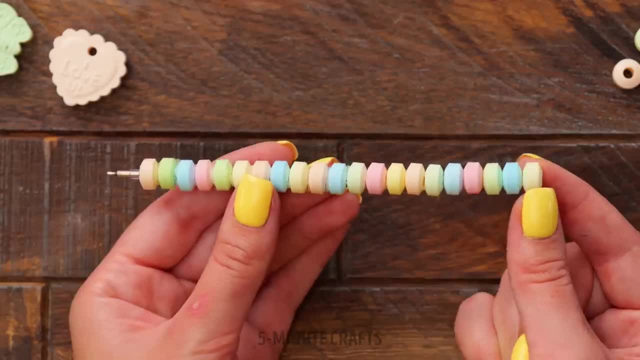 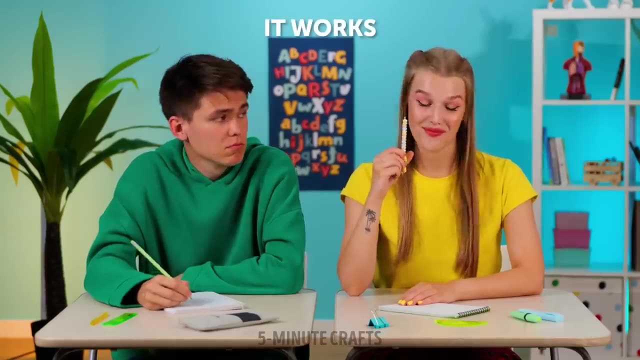 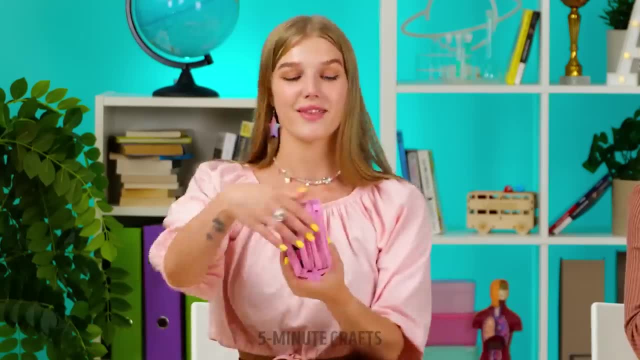 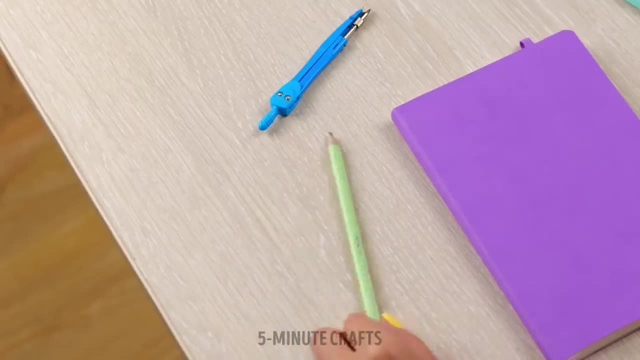 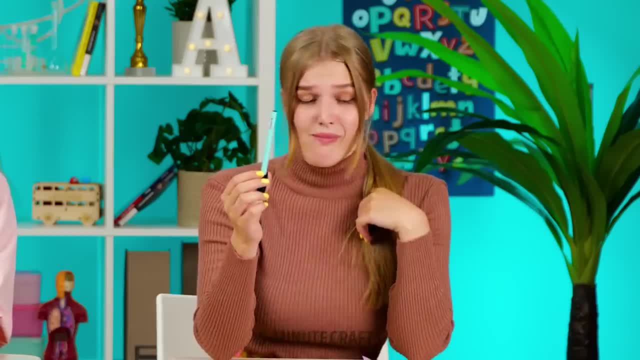 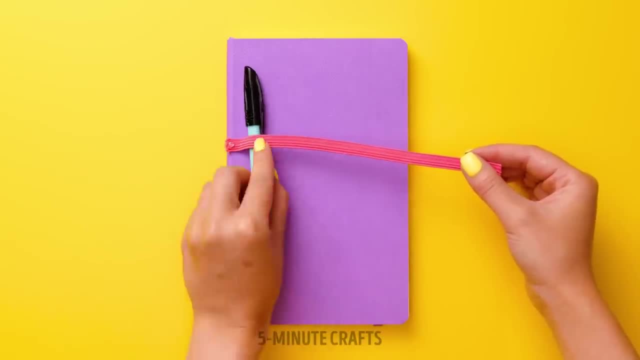 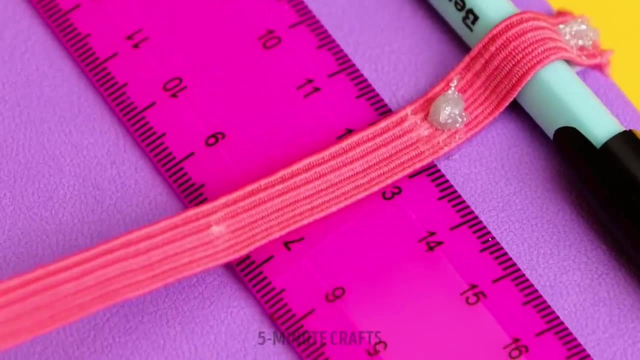 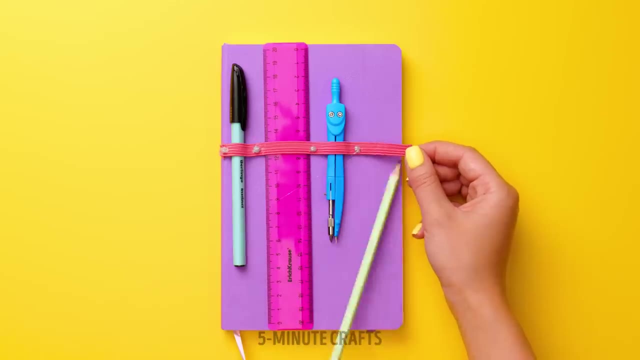 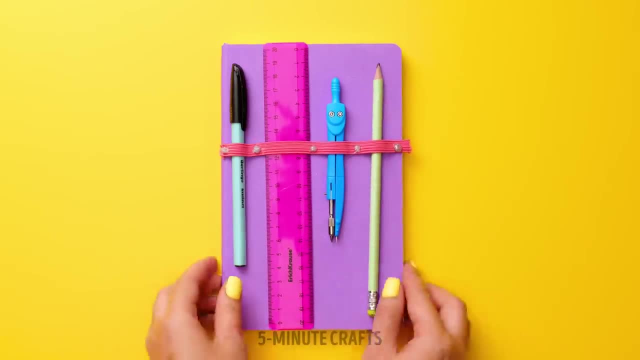 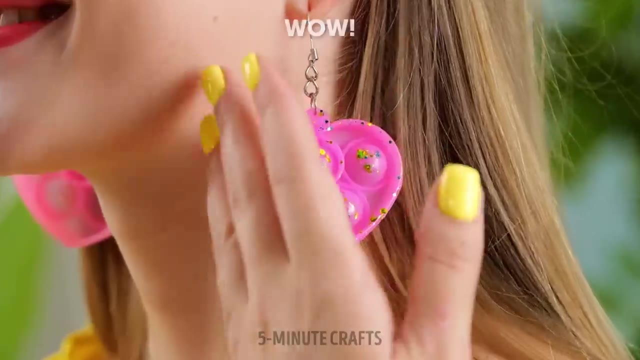 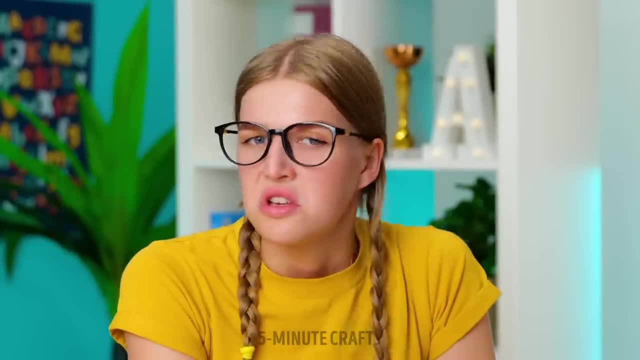 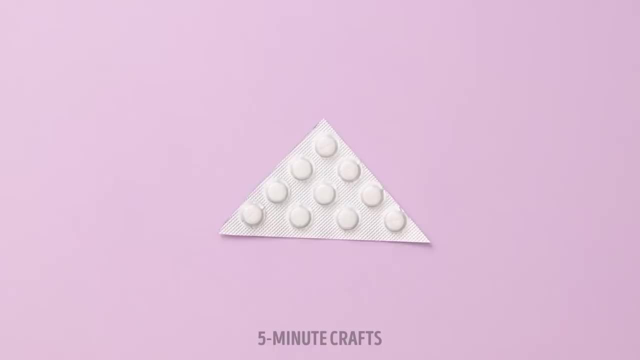 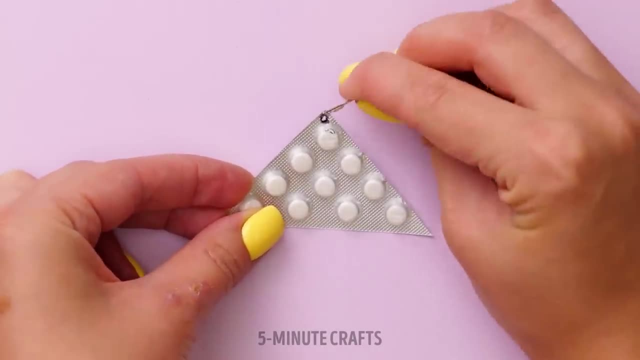 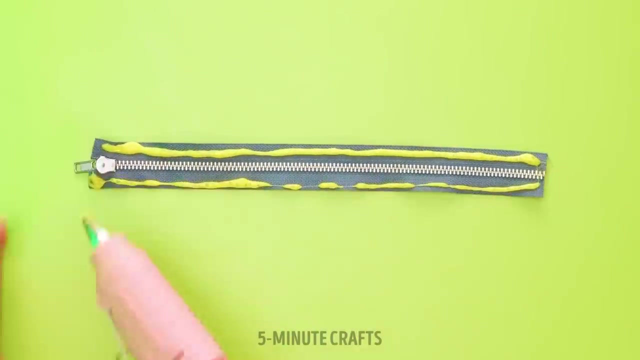 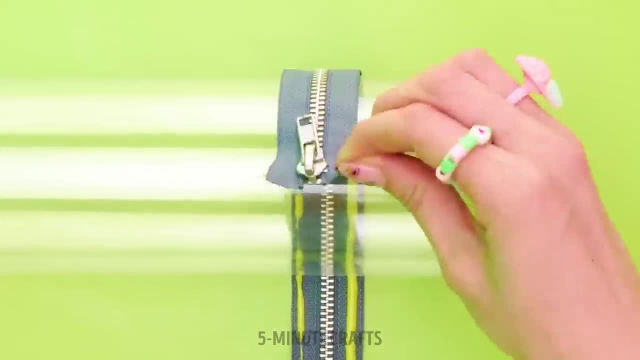 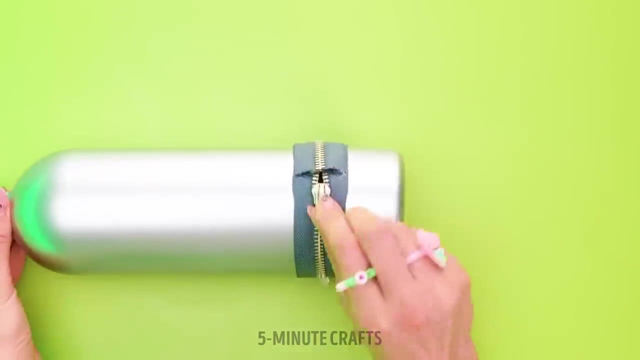 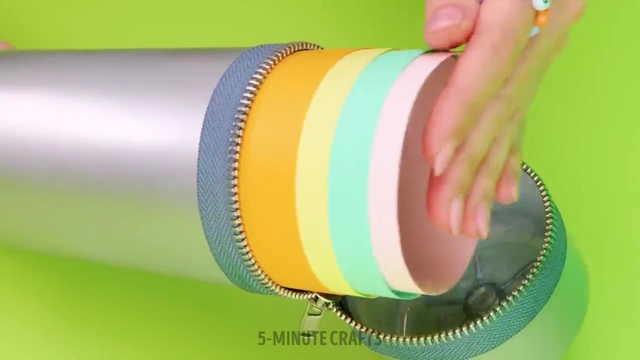 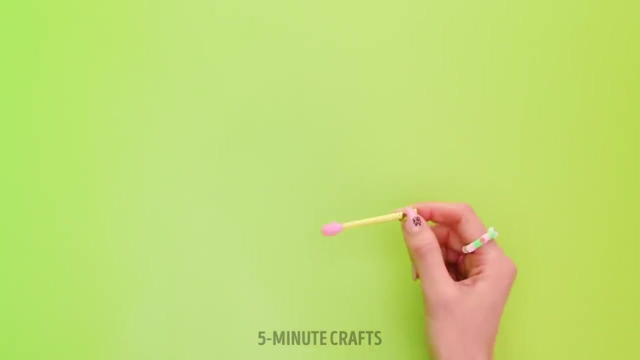 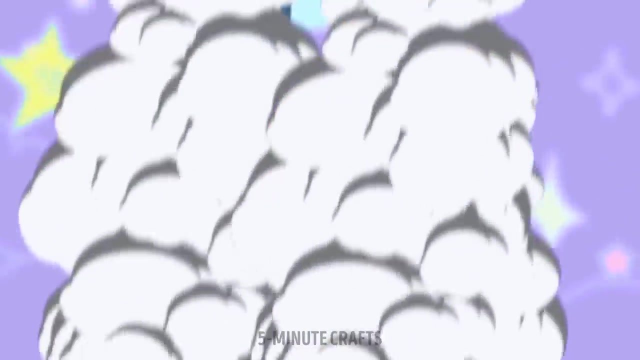 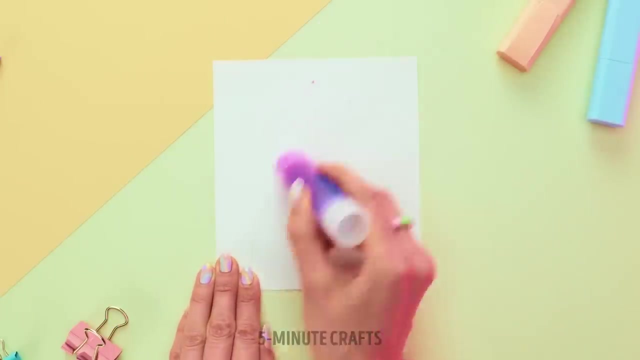 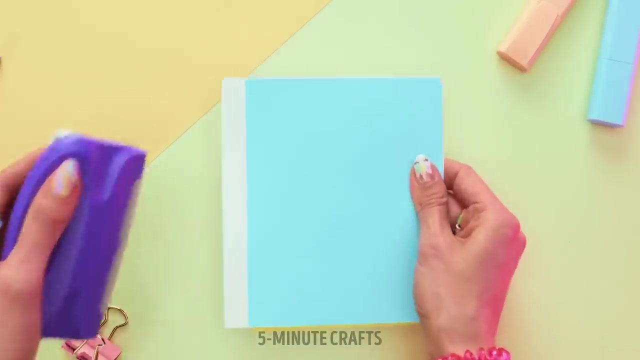 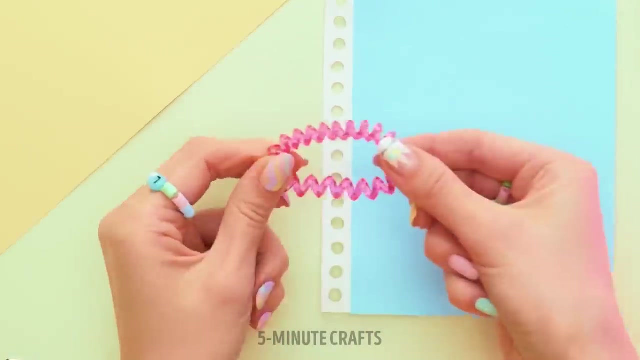 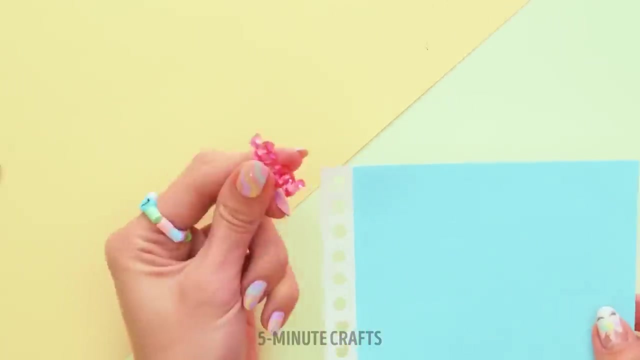 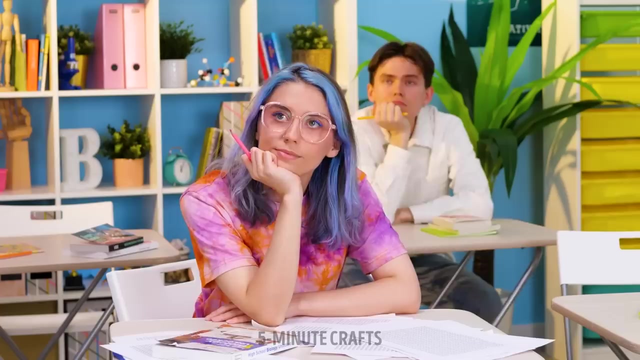 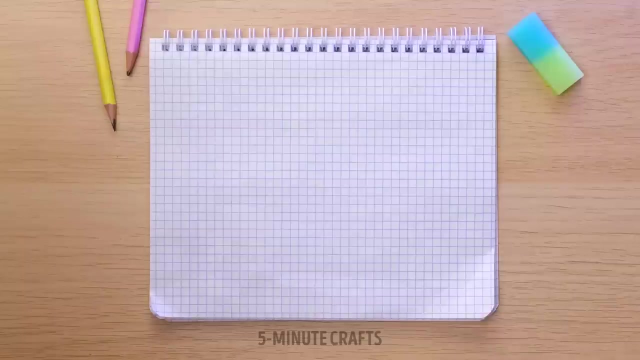 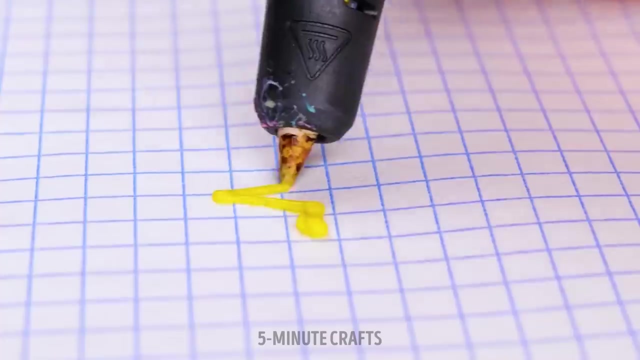 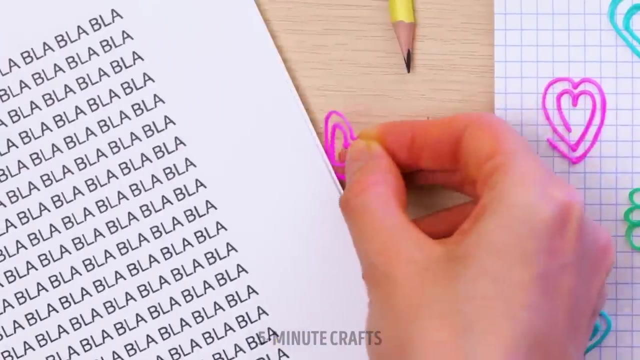 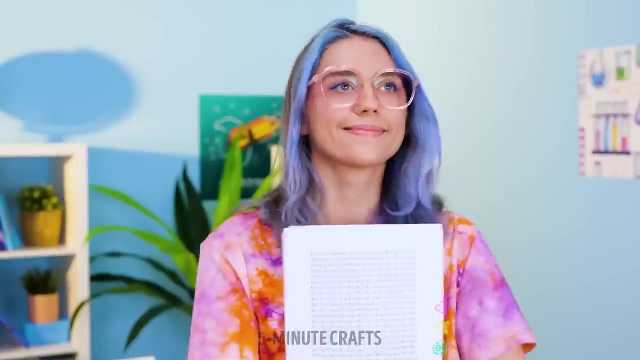 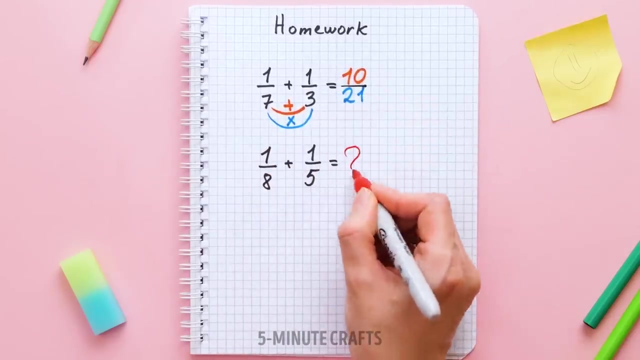 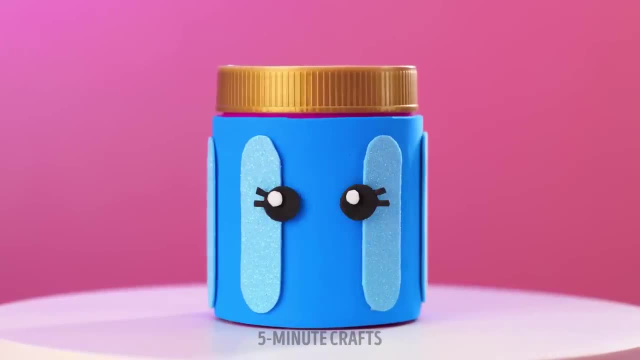 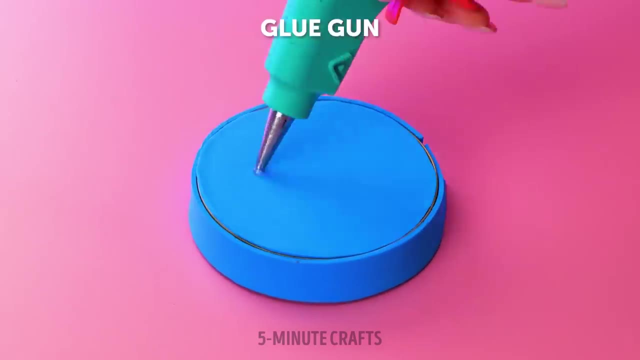 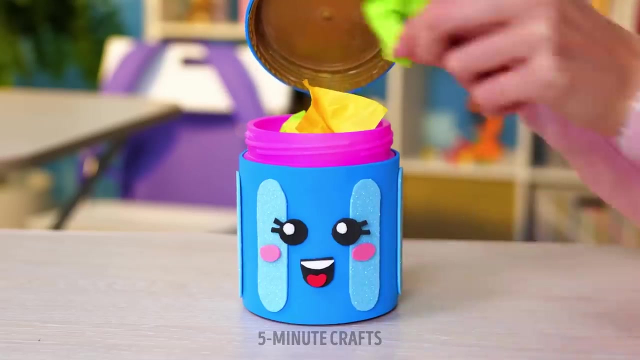 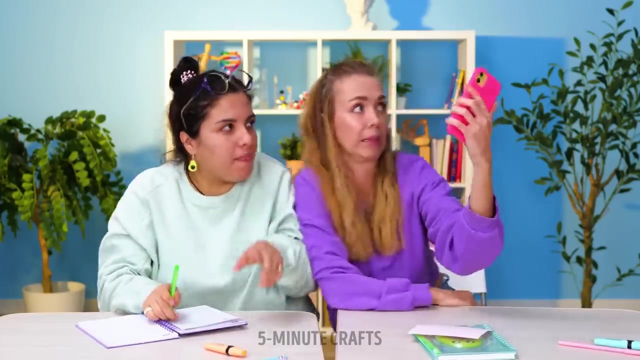 Thank you for watching. Thank you for watching. Thank you for watching. Don't look back. My Mama always used to say: You'll find another Endless love. It's coming, I'll be sure of that, But its so hard Cause its you. its you, Always on my mind. Yeah, its you. its you. Take it all by time, Let it sink in. haven't you been hurting enough? Give you all of my love, but you don't seem to care. Put my arms around you, but your heart isn't there. Don't tell me we're fine lying to yourself. 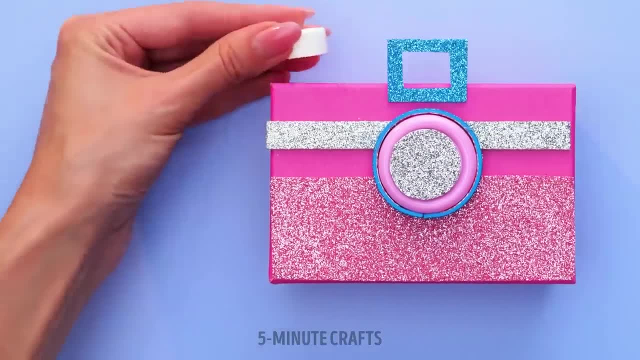 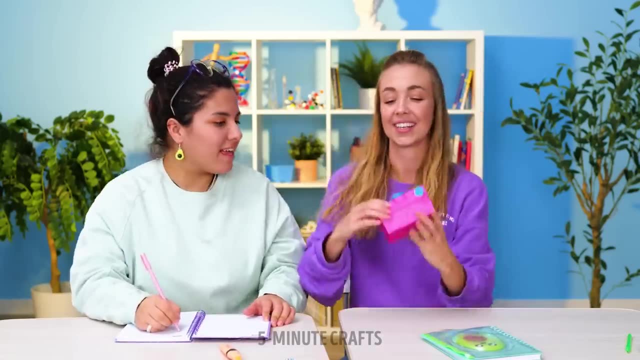 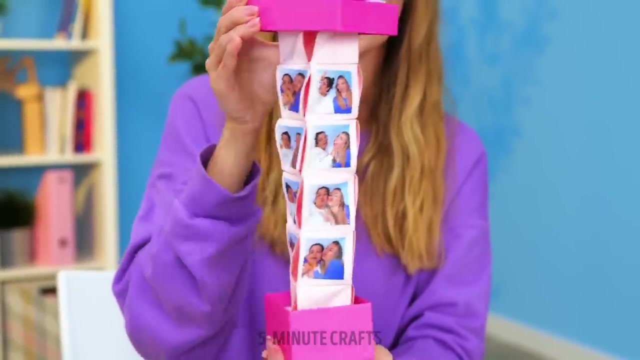 It's so late to meet up. we are too far apart. It's so late, can't you see? I can't trust you no more. Gotta get over you, cause I'm more than the dark. It's so late to meet up. too late to meet up. 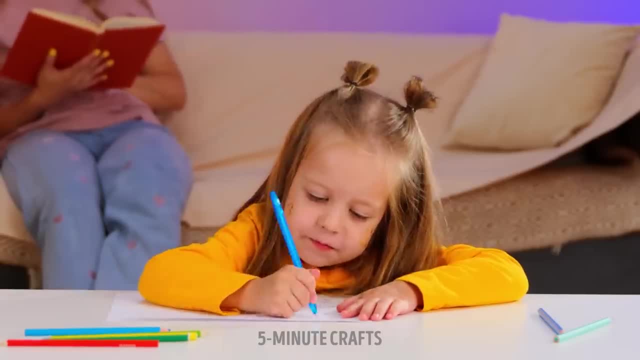 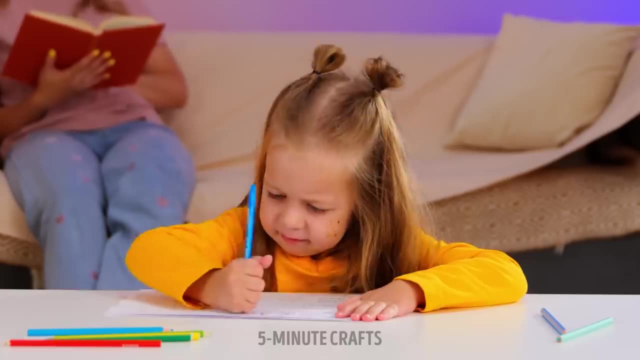 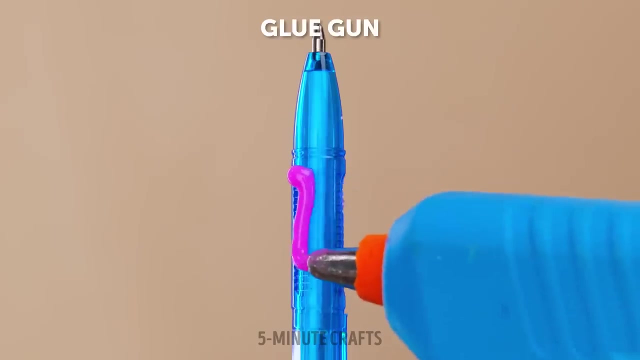 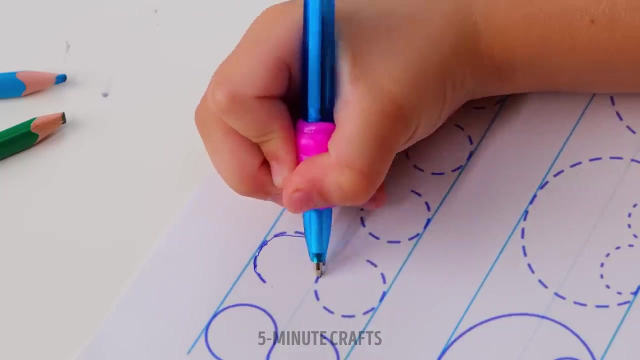 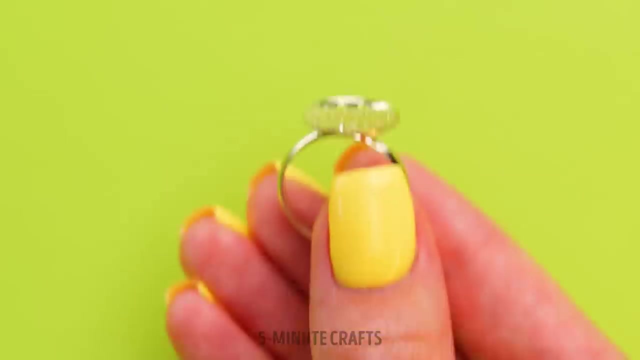 Too late to meet up. Don't go there. Don't go there. If you can't, If you can't, If you can't finish what you start, I can't keep up. You're holding back, And then you let it go too far. Just stay away. But it's you, it's you. 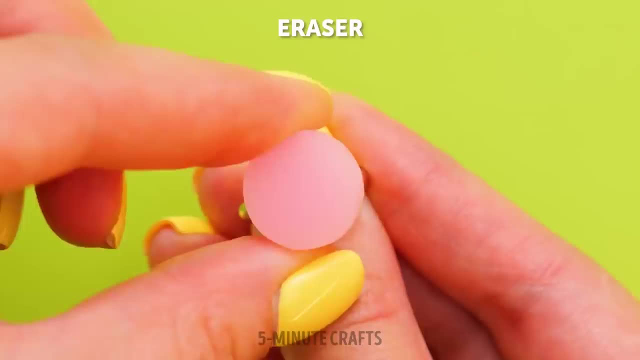 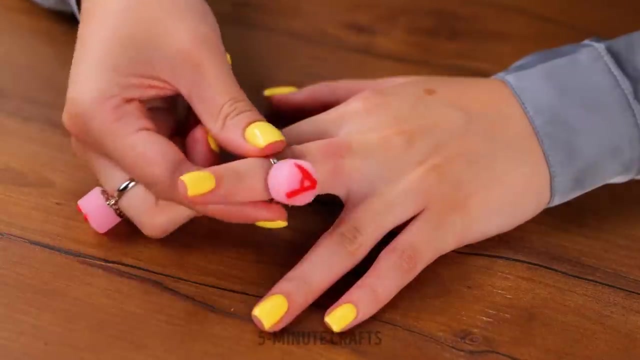 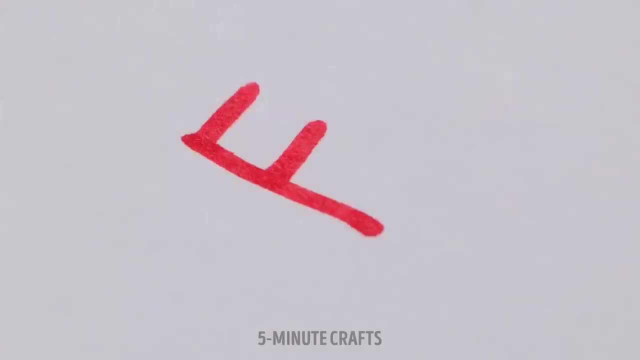 Always on my mind. Yeah, it's you. it's you Taking up a time and let it sink in? Haven't I been hurting enough? Oh, oh. Give you all of my love, But you don't seem to care. Put my arms around you, but your heart isn't there. 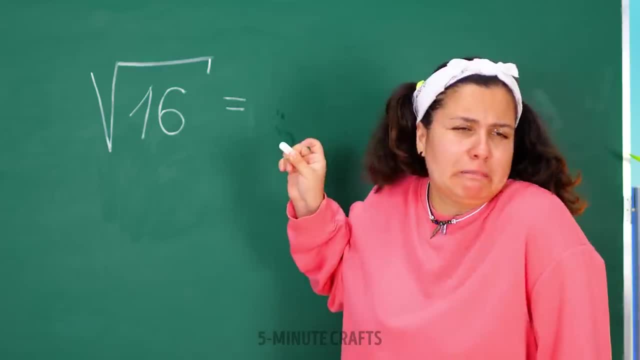 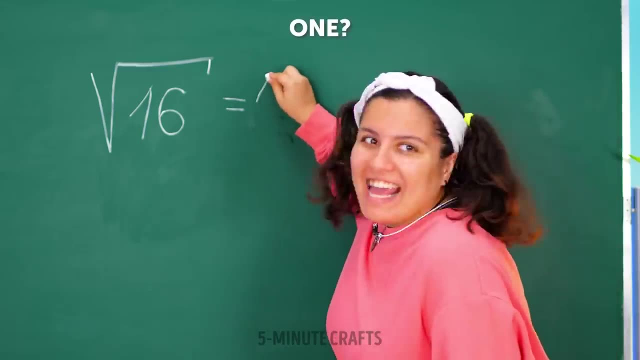 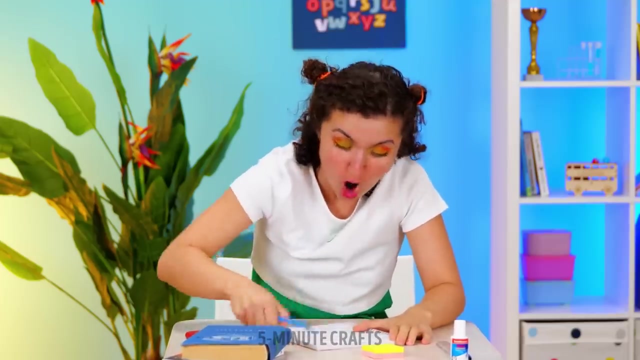 Don't tell me we're fine, lying to yourself. It's too late to meet up. we are too far apart, Too late, can't you see? I can't trust you no more. Gotta get over you, cause I'm more than the dark. It's too late to meet up. 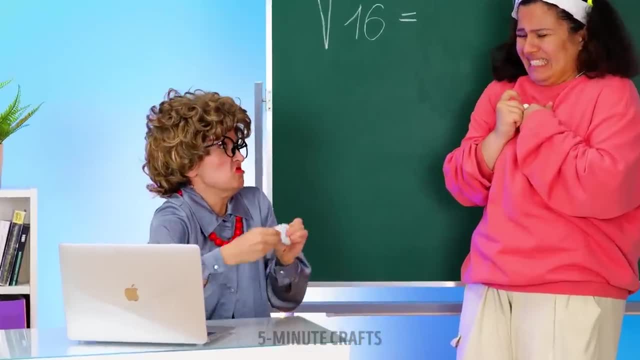 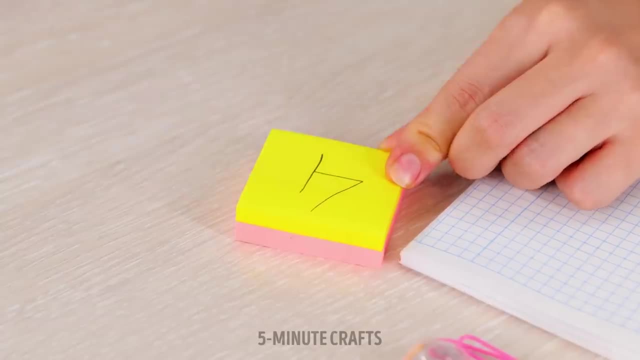 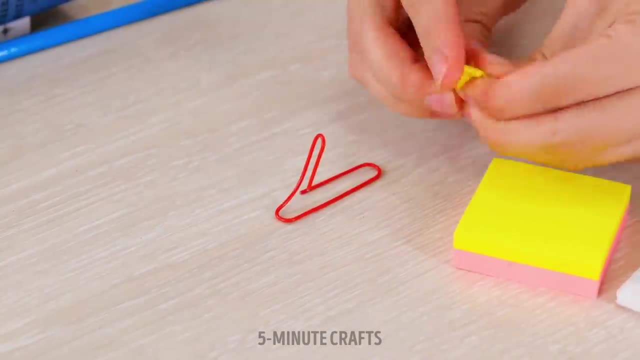 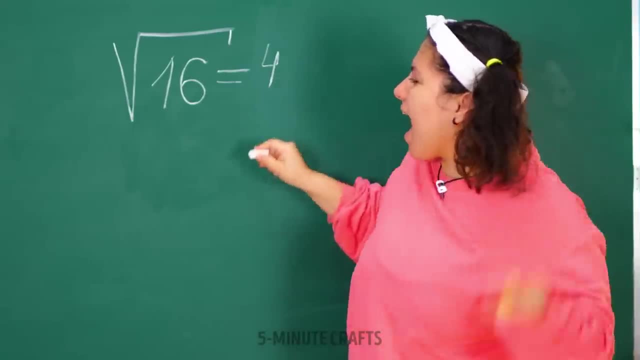 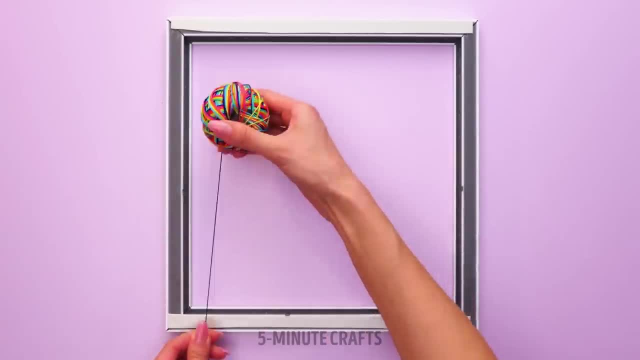 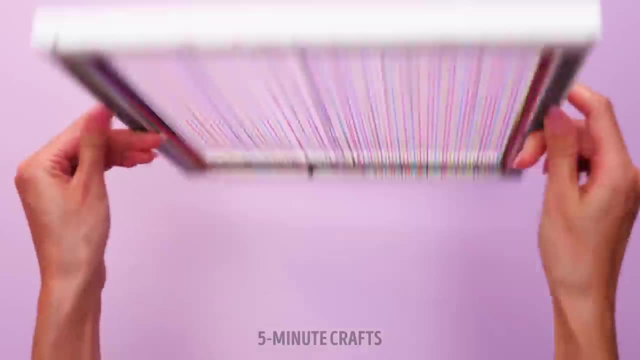 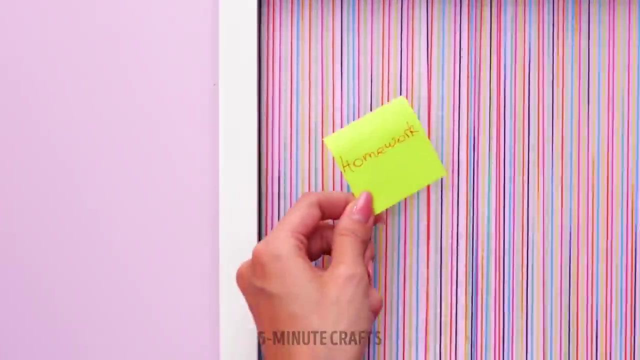 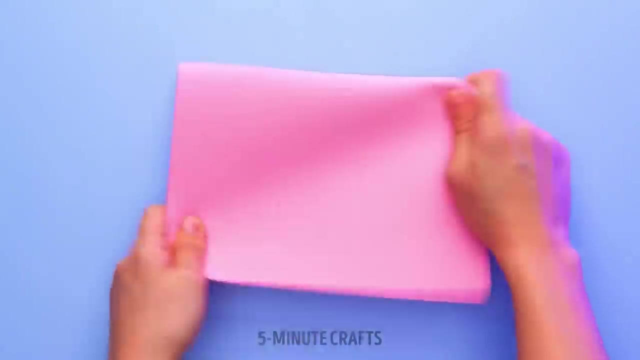 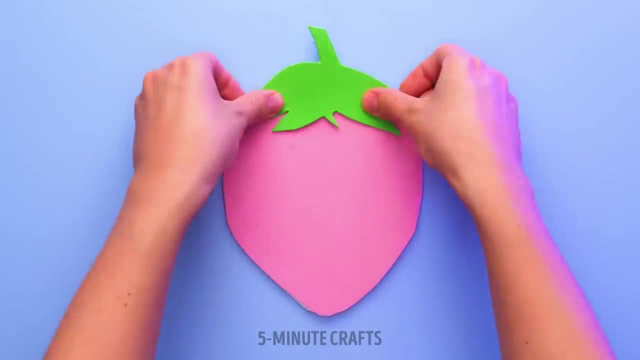 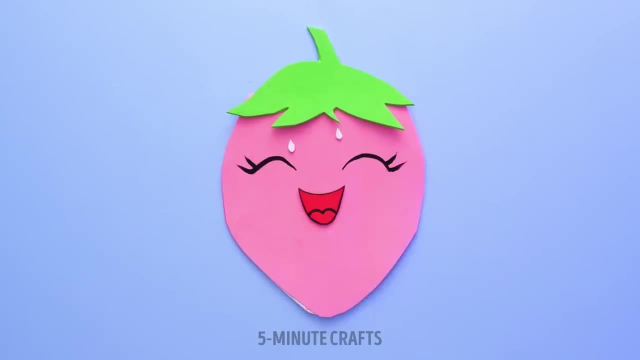 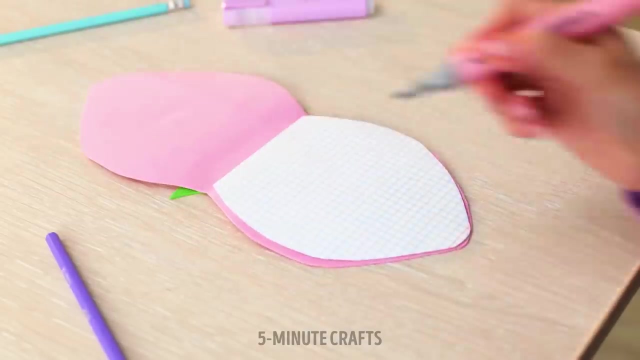 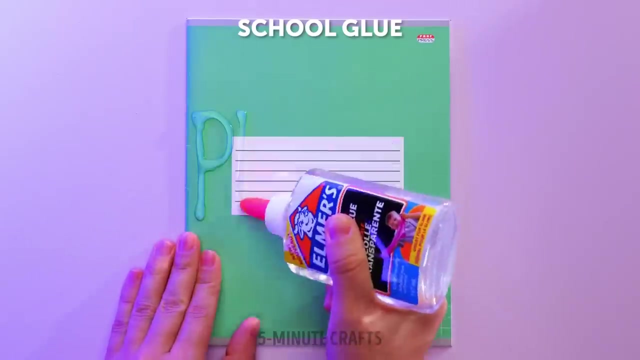 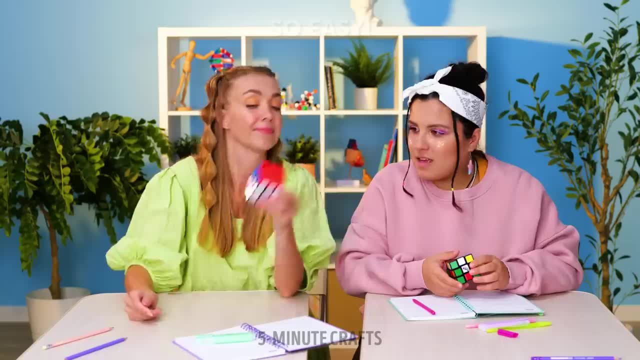 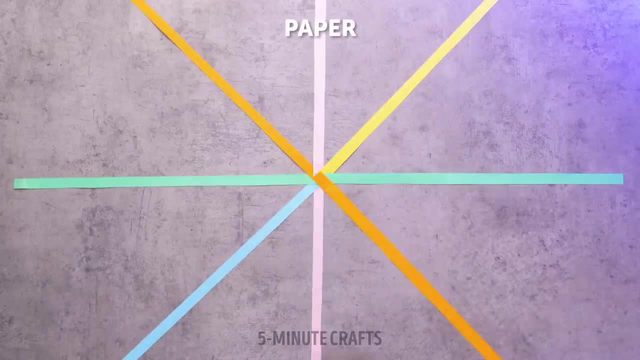 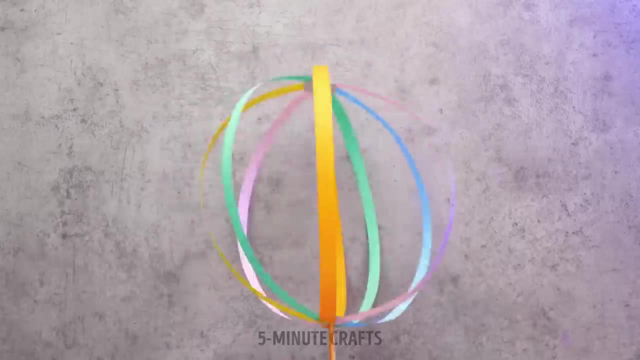 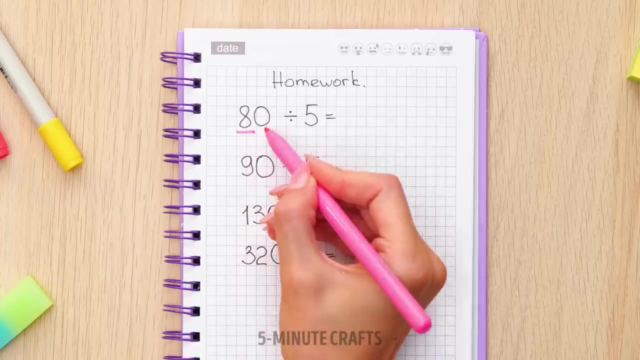 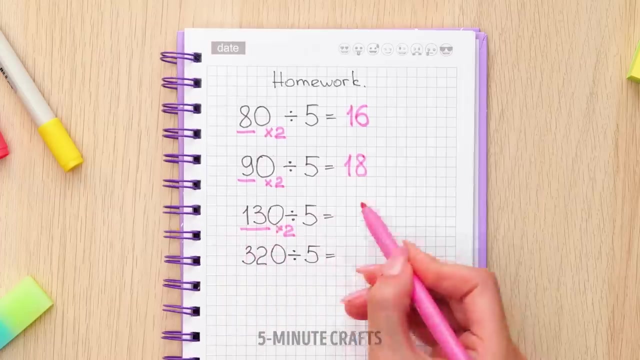 I feel the love. Baby, what's your number? I wanna go under Making you a memory. that's really all I need, All I need, all I need. I'm alive and breathing, living my best life. Love is on my mind and it's taking me high. 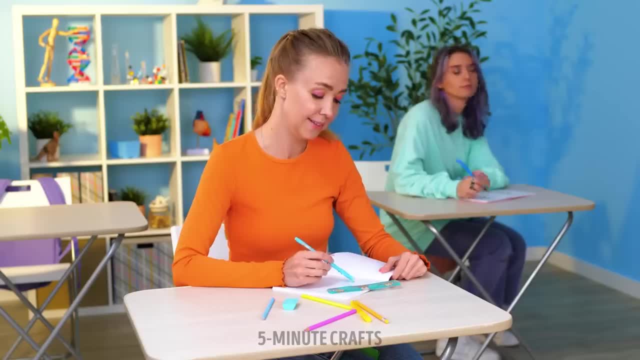 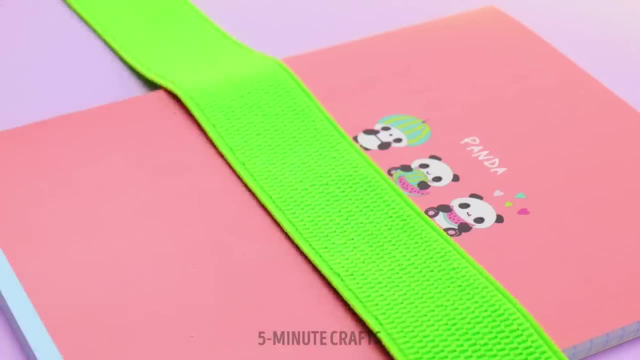 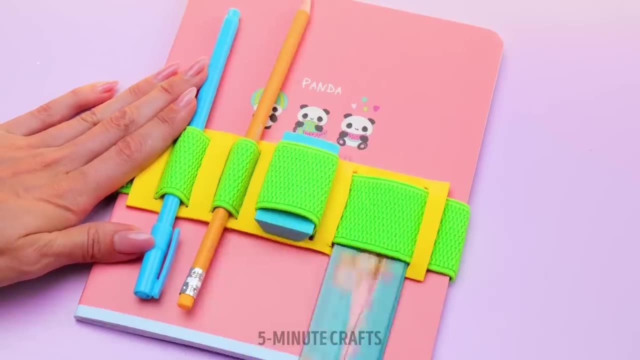 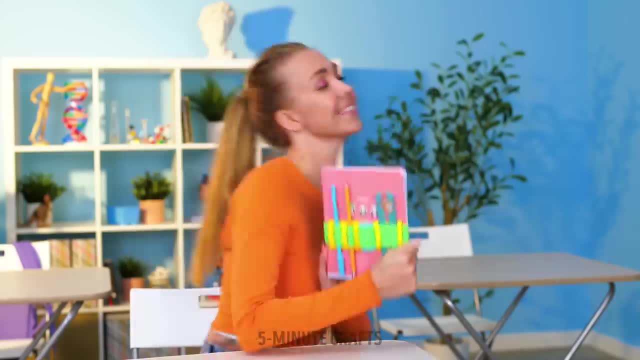 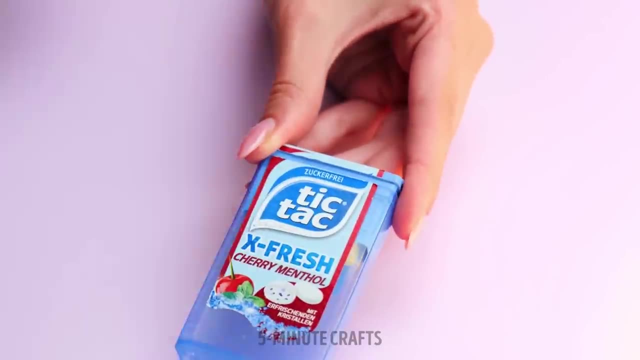 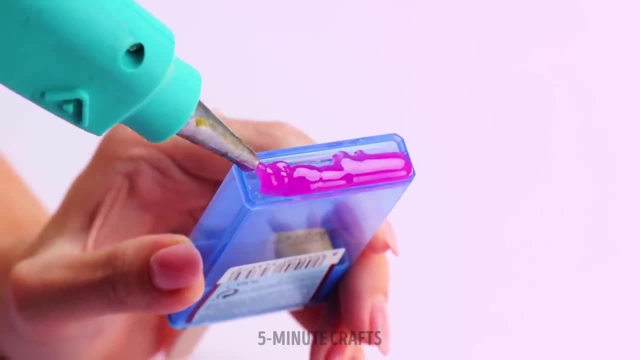 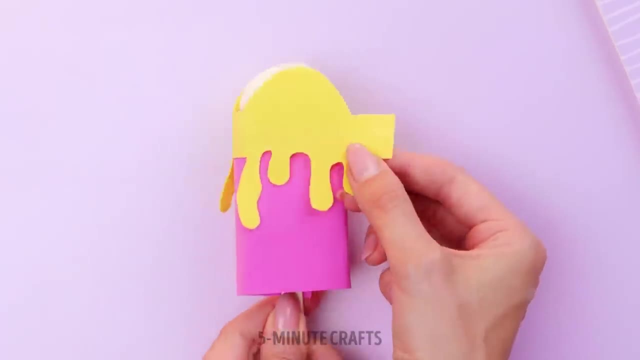 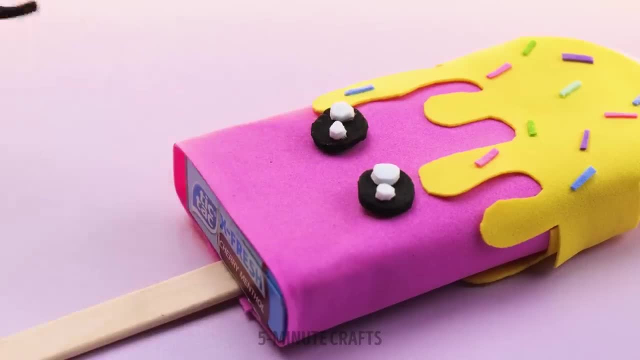 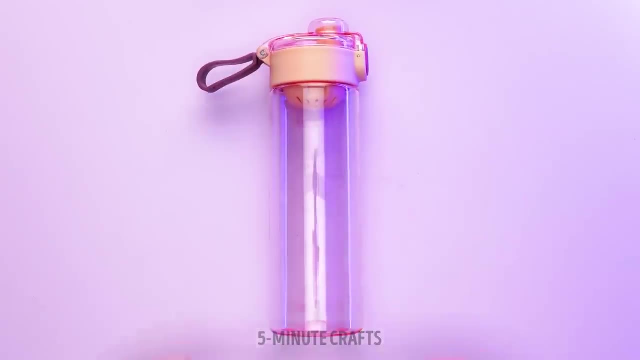 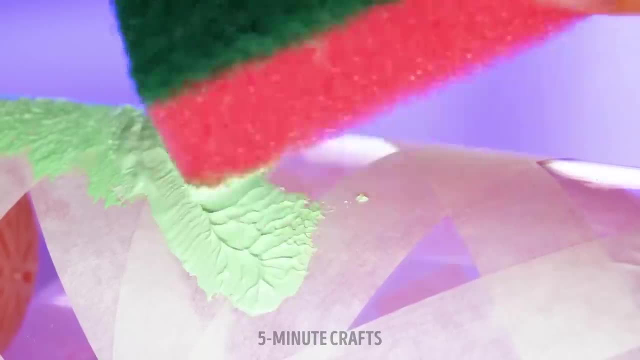 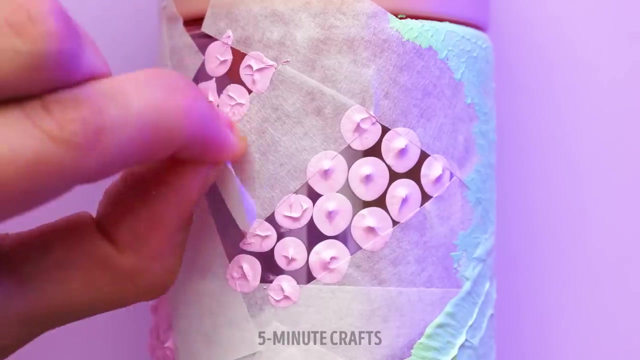 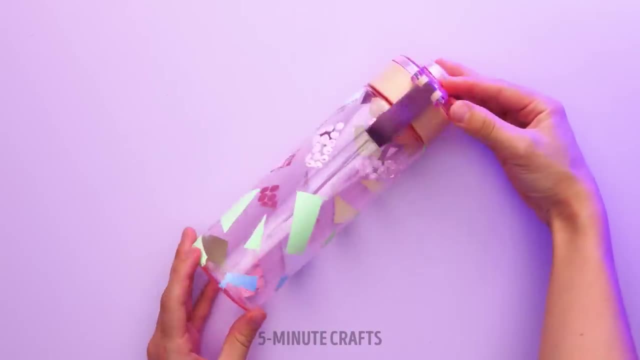 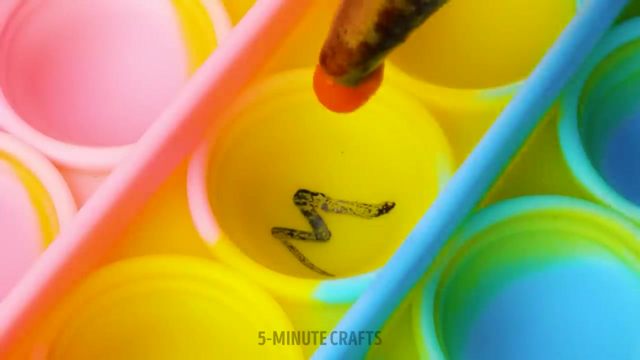 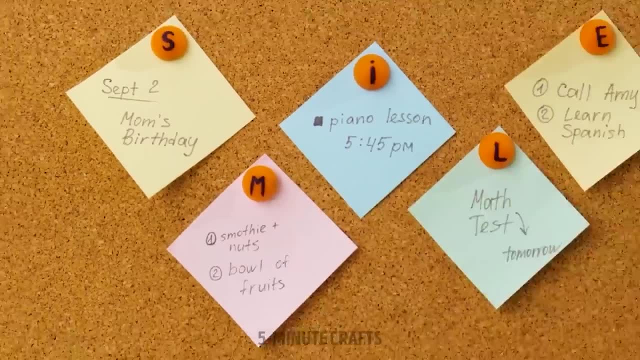 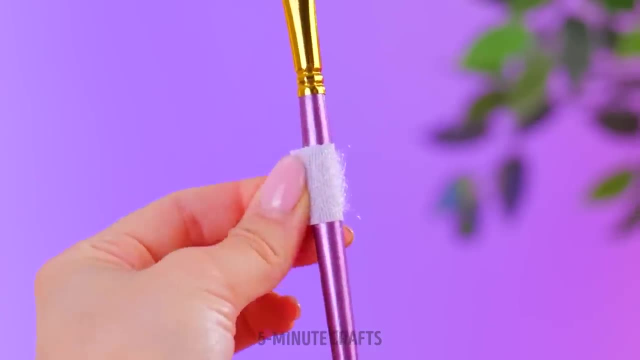 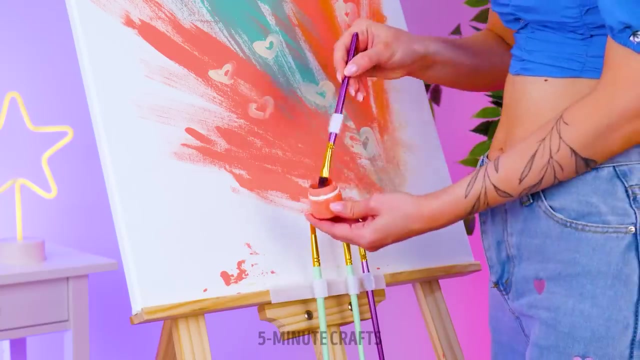 I used to think that you were only mine, But I was blinded by a shallow lie. I'll call your friends. I'll let them know That I'm so done with the tragic boys. Tonight. I'll get into my zone. I'll dance until the tears are gone. 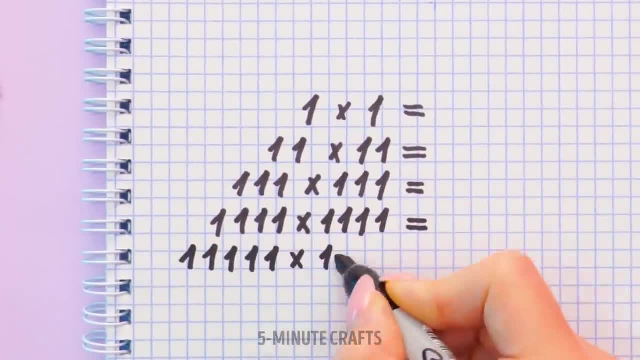 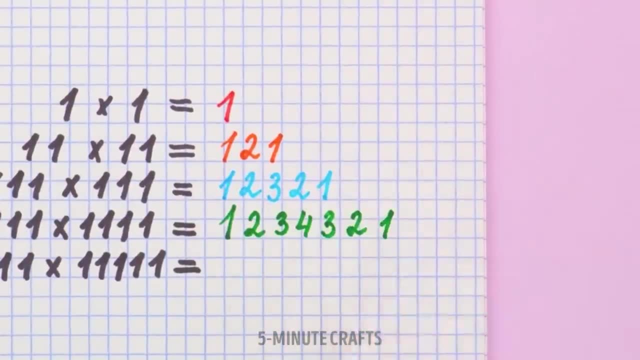 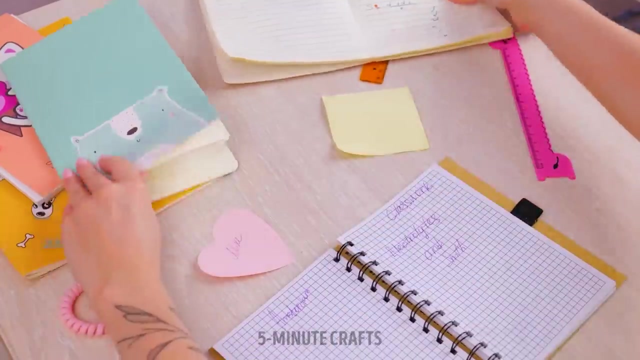 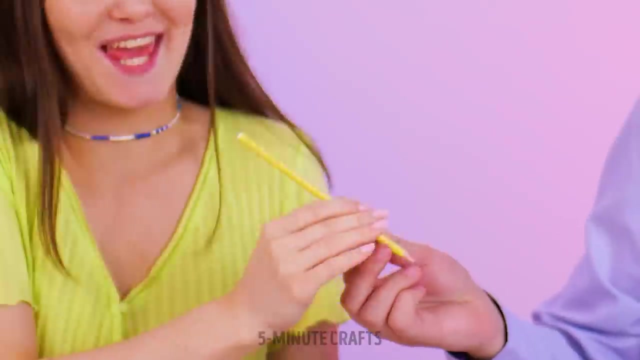 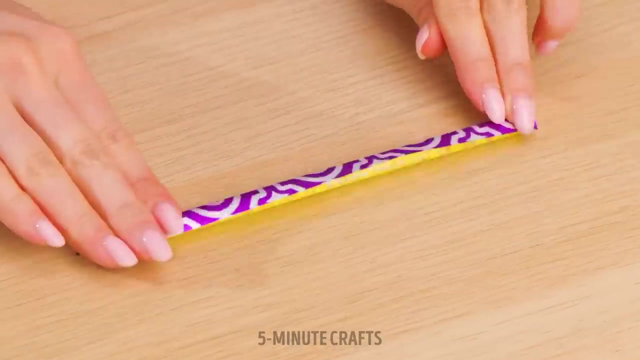 No time for bad love. bad love, bad love. I'm dancing all these tears away. No time for bad love. bad love, bad love. I'm dancing all these tears away. Don't need ya, Don't need ya. Even you just made me realize All the things I used to sacrifice. 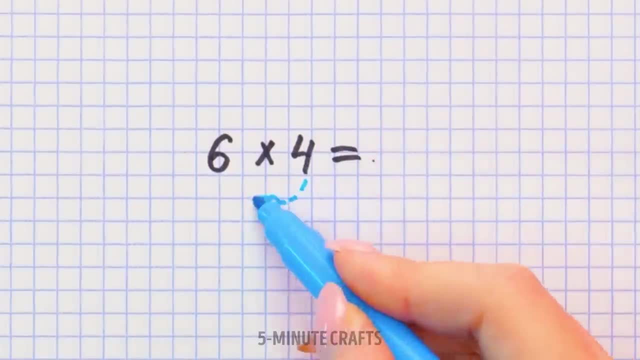 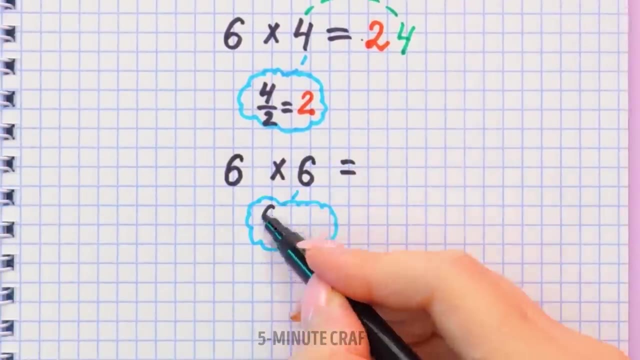 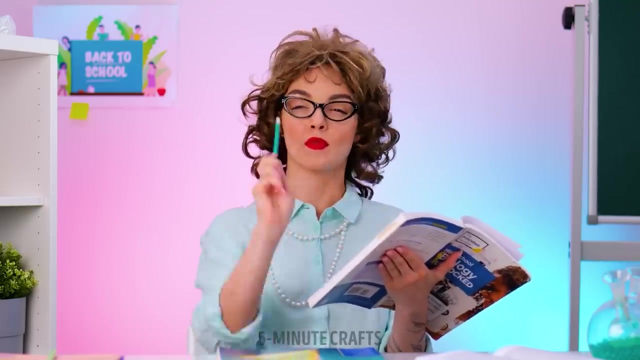 Just to please you, just to call you mine. But look at me. now I have the time of my life. I'll call your friends. I'll let them know That I'm so done with the tragic boys. Tonight I'll get into my zone. I'll dance until the tears are gone. 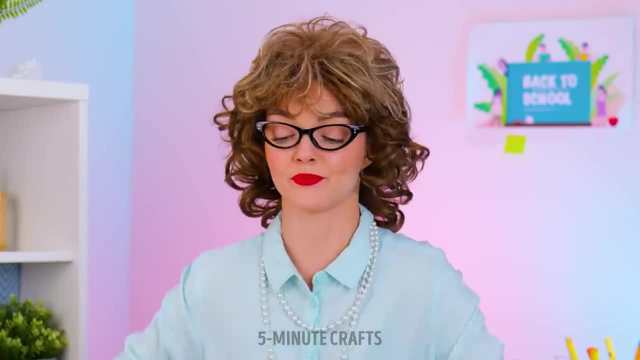 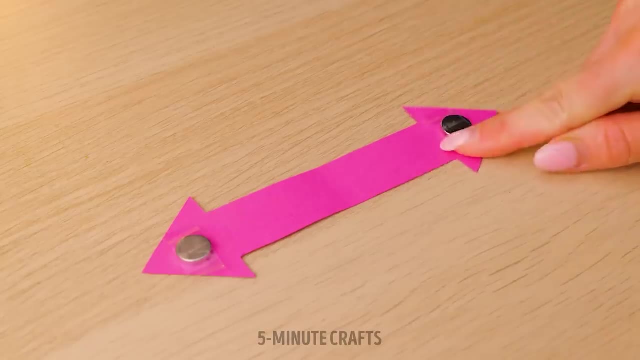 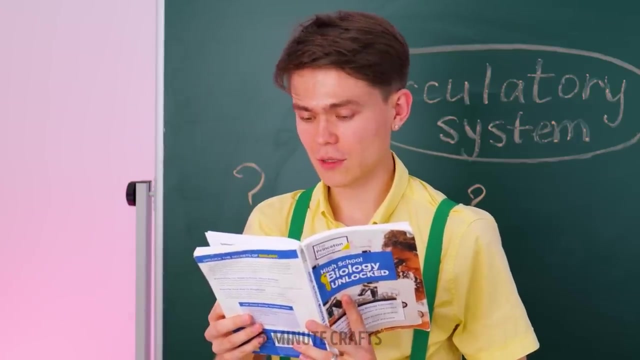 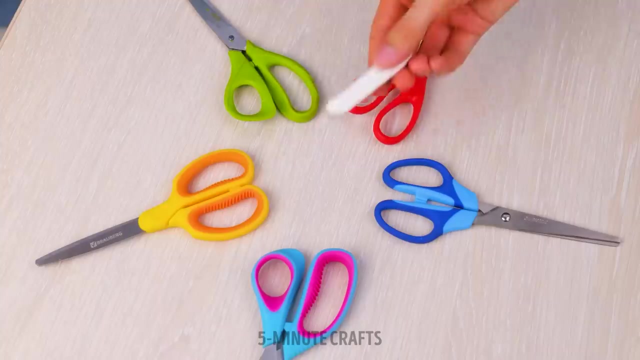 No time for bad love. bad love, bad love. I'm dancing all these tears away. No time for bad love. bad love, bad love. I'm dancing all these tears away. Don't need ya. I've got you now. I've shown you now. 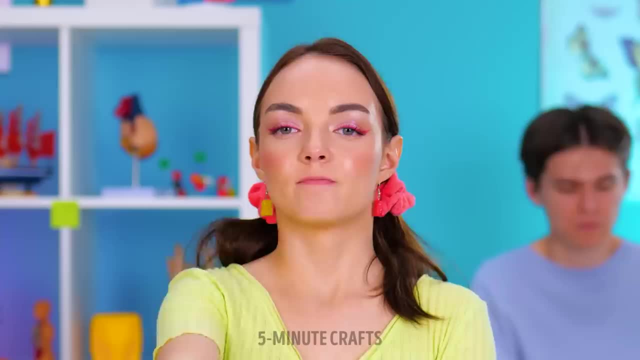 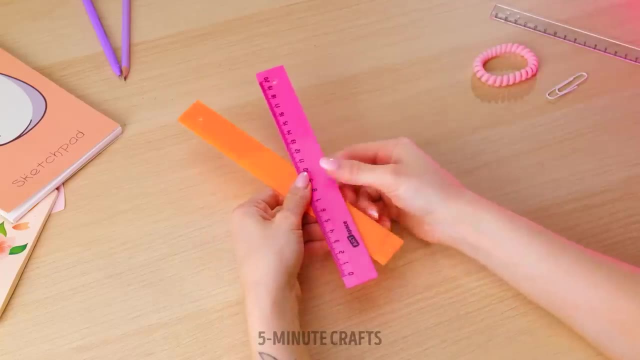 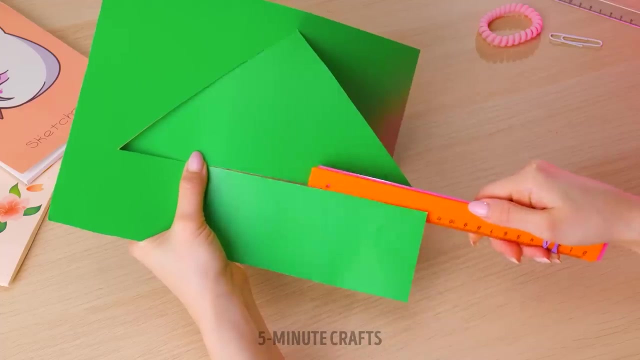 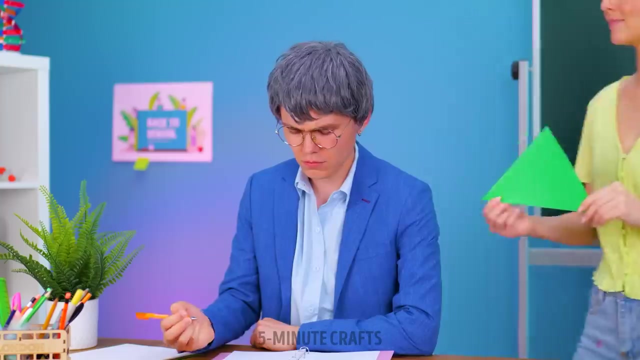 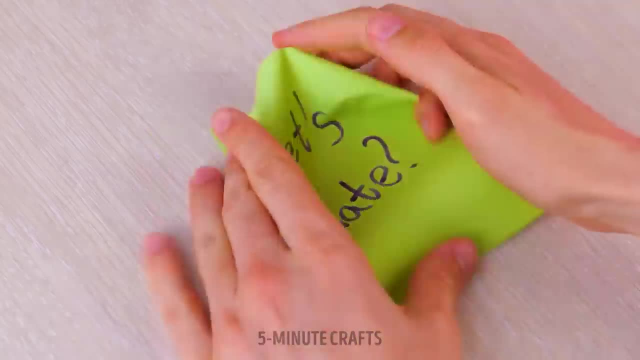 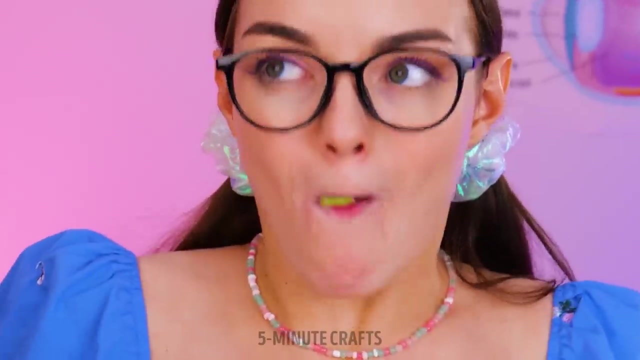 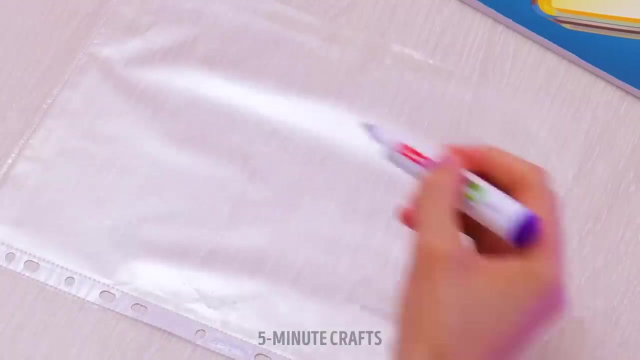 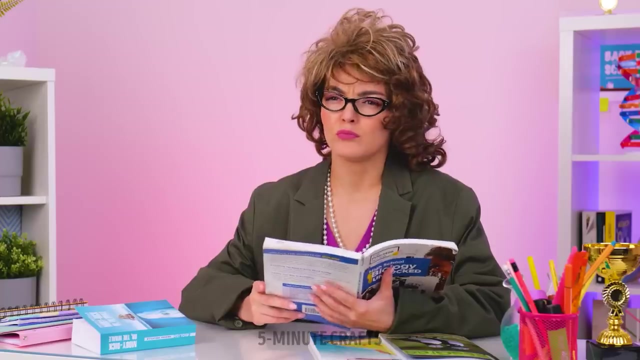 Dancing all these tears away. Dancing all these tears away, Dancing all these tears away. No time for bad love, bad love, bad love. I'm dancing all these tears away. No time for bad love, bad love, bad love. I'm dancing all these tears away. 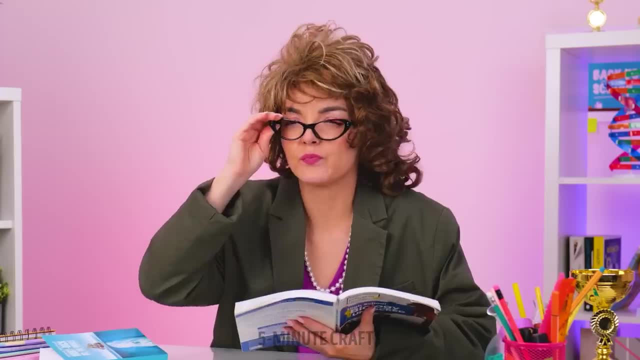 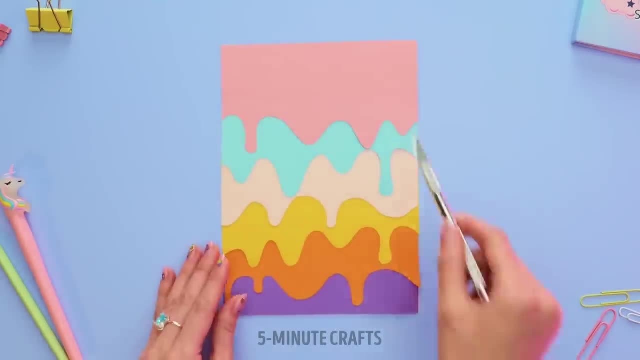 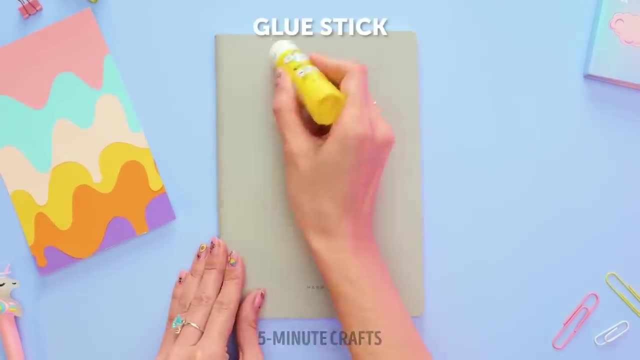 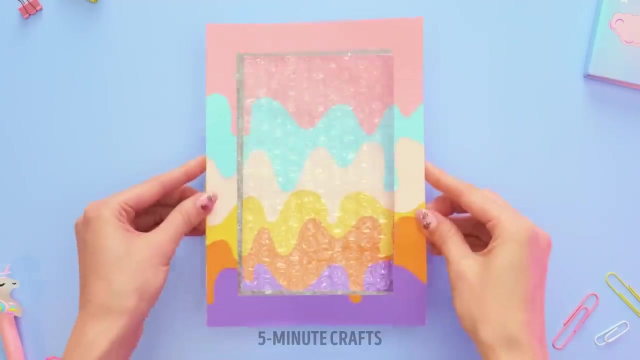 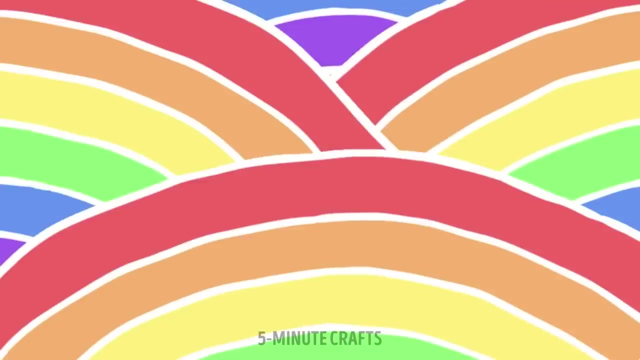 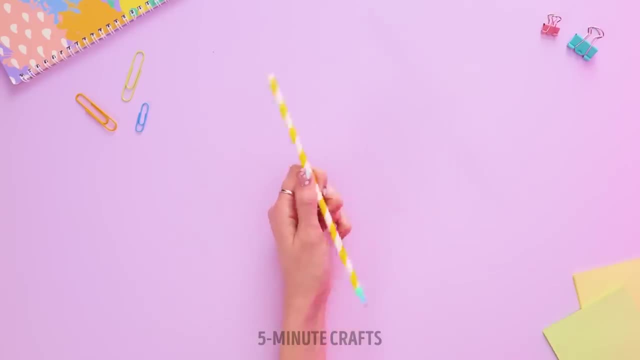 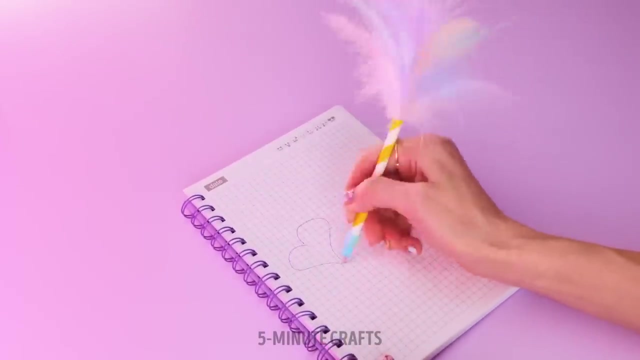 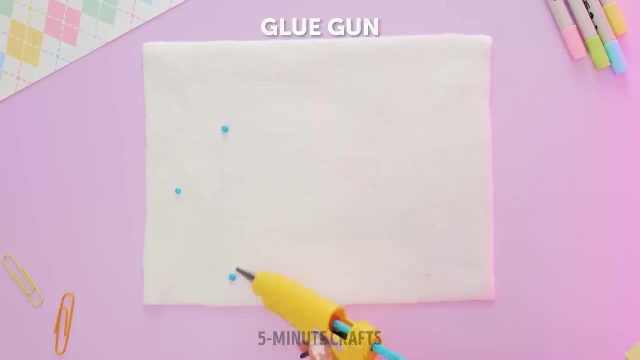 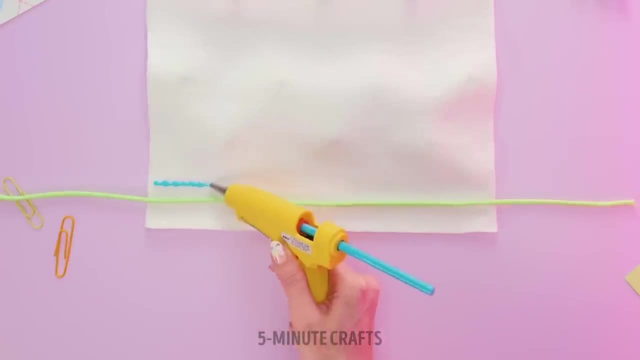 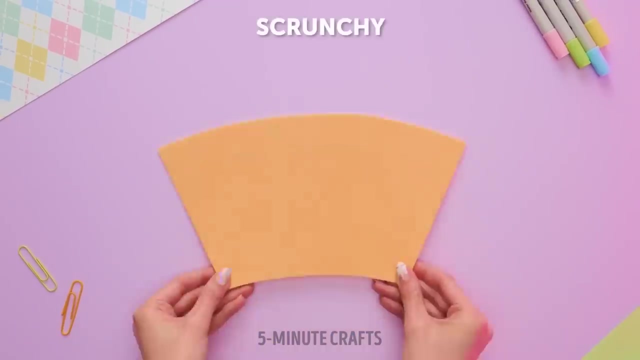 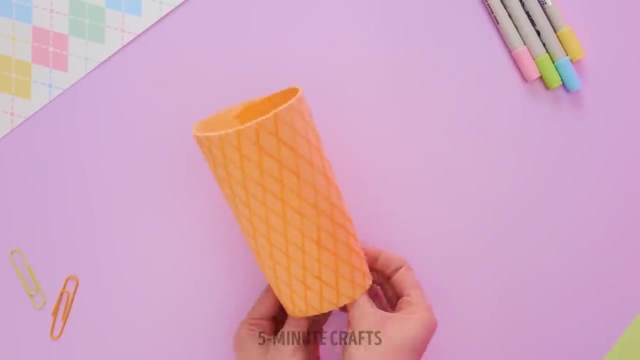 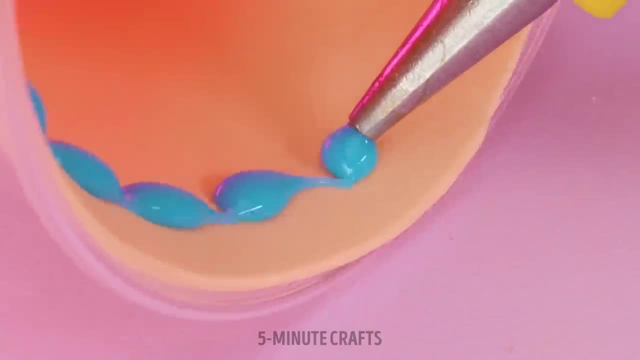 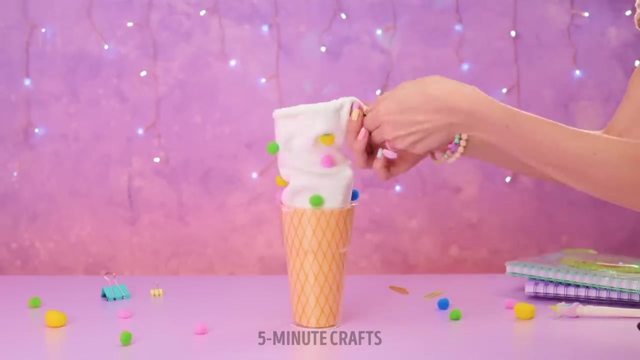 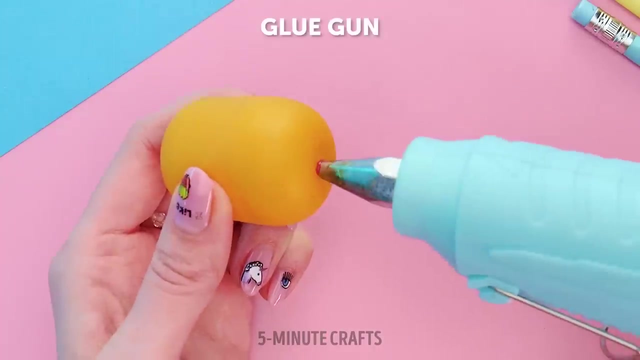 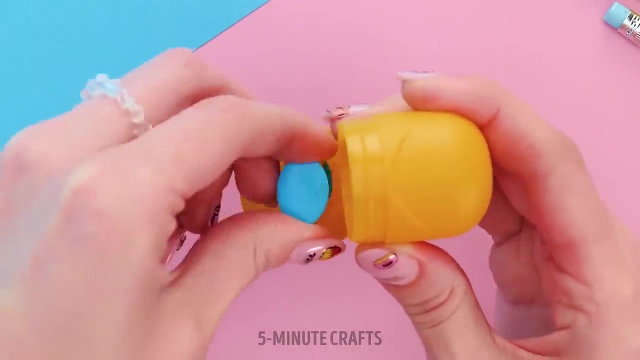 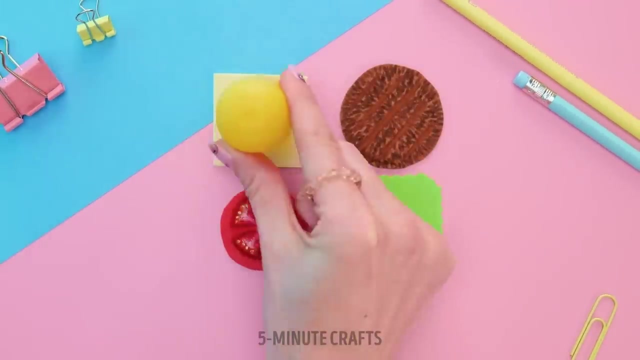 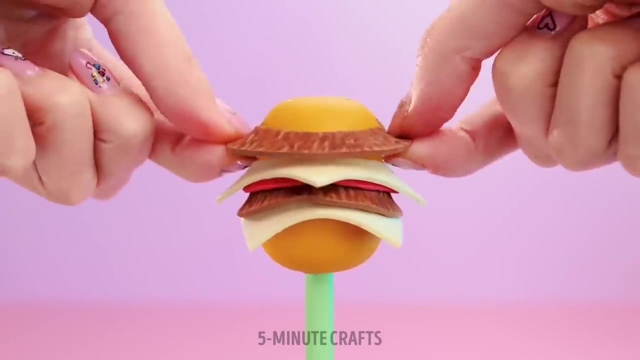 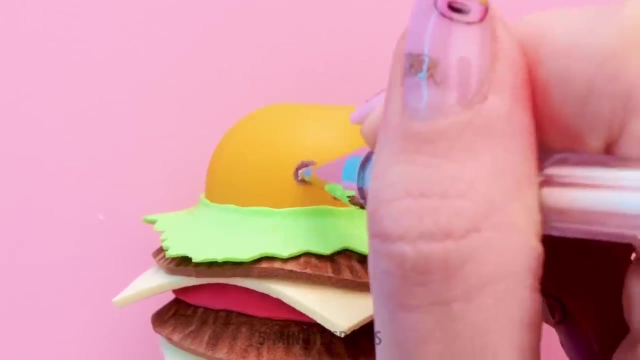 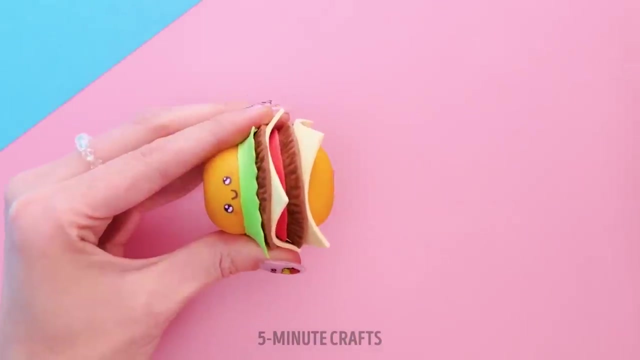 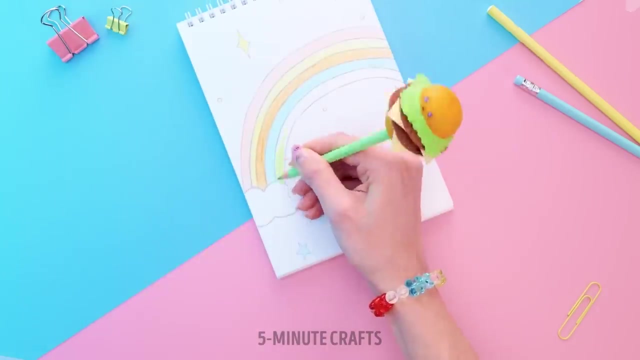 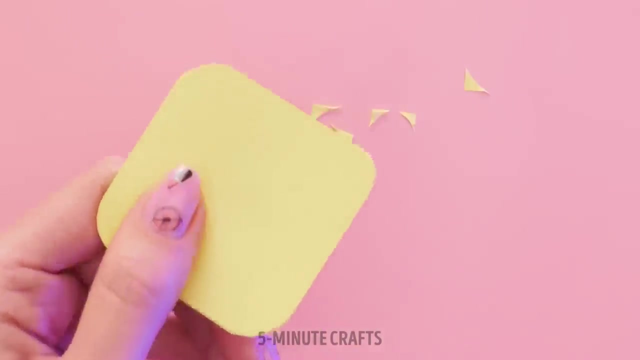 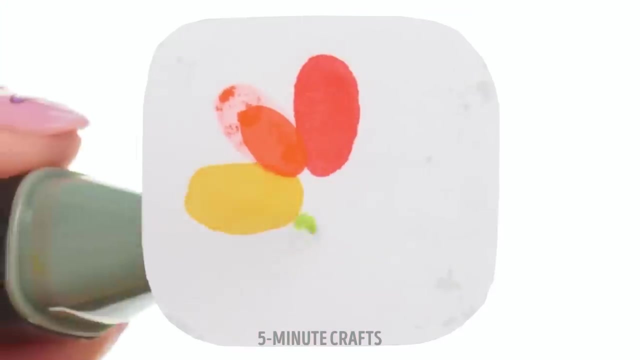 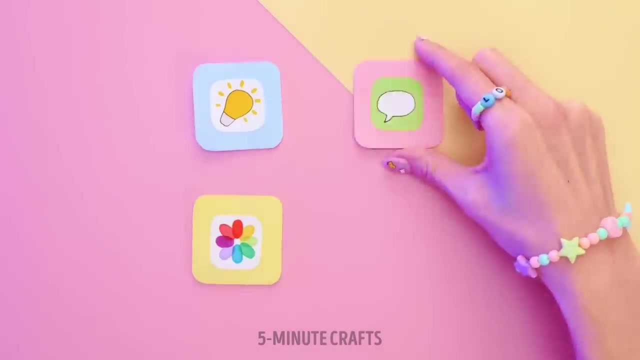 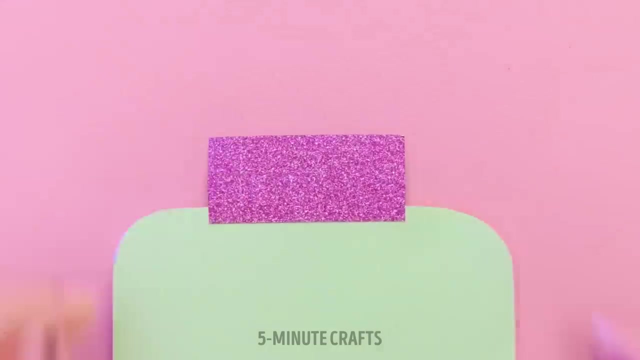 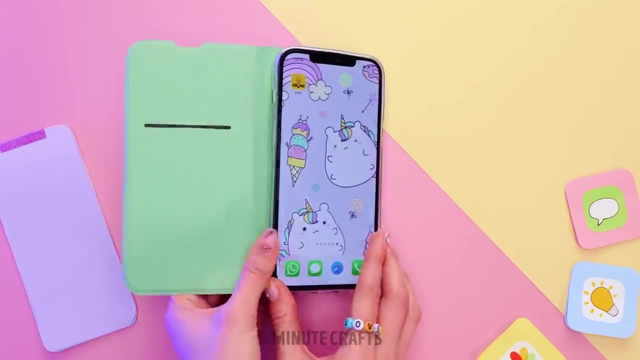 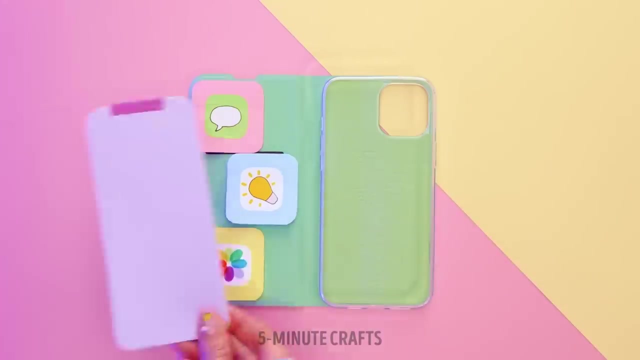 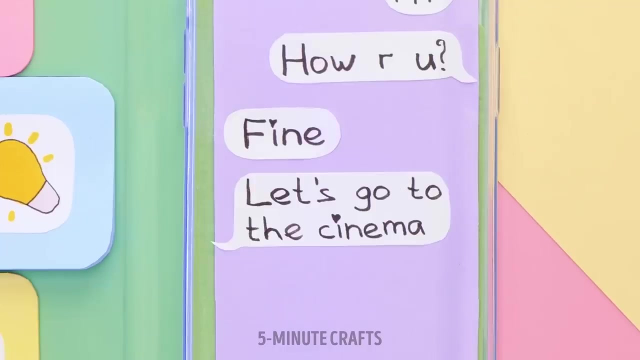 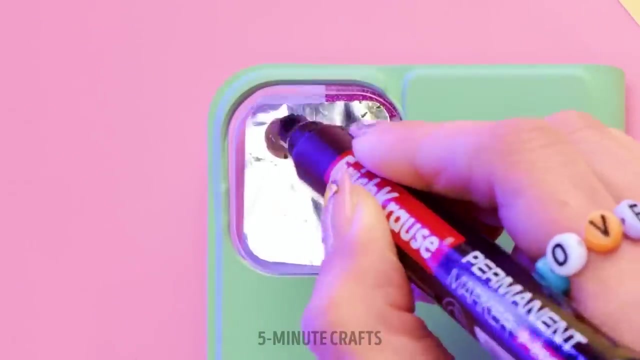 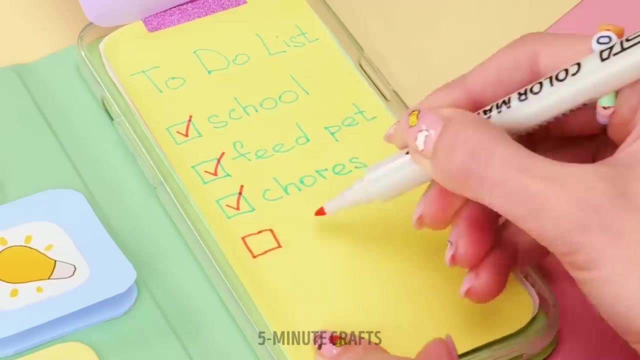 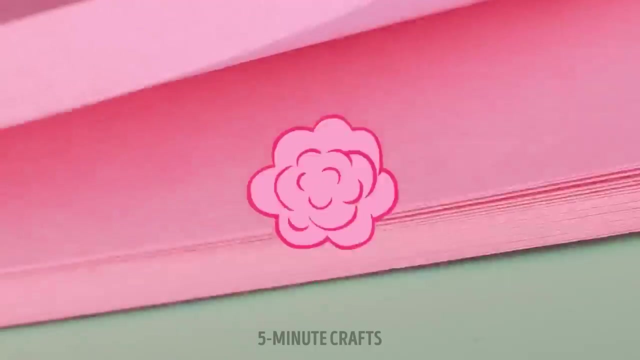 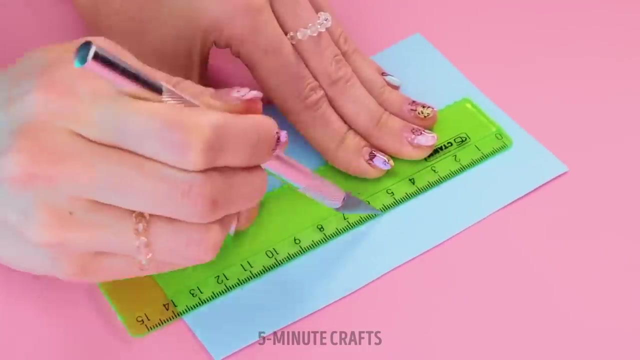 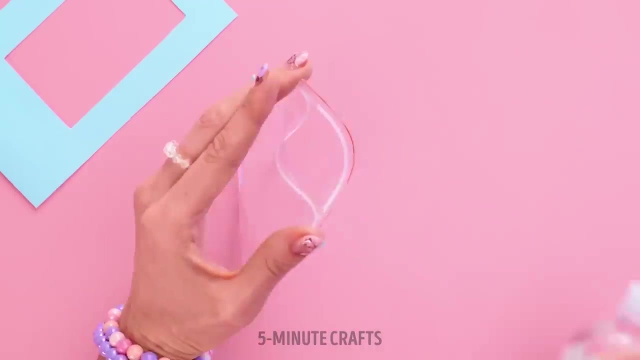 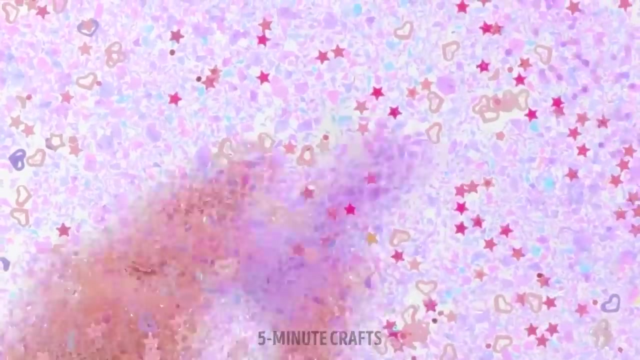 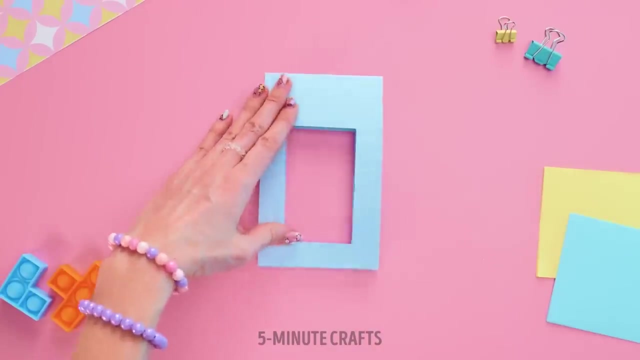 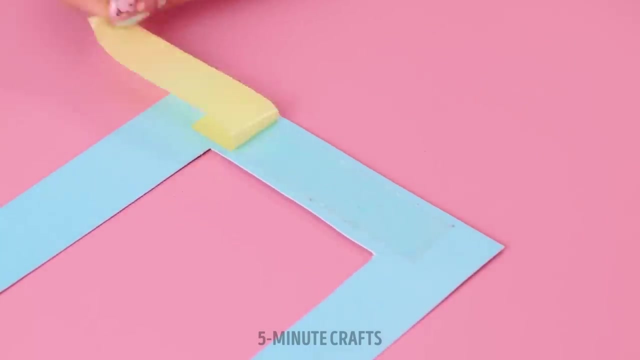 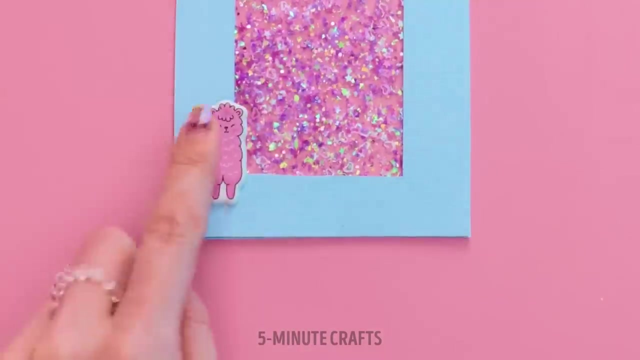 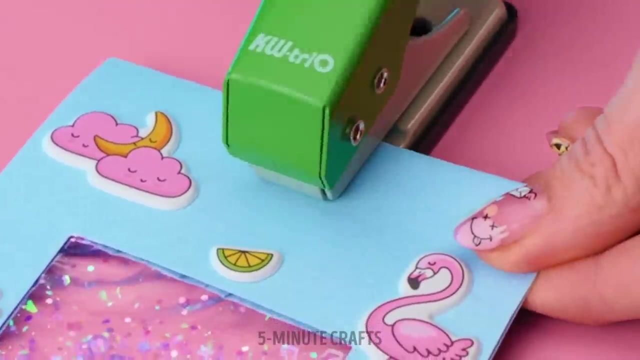 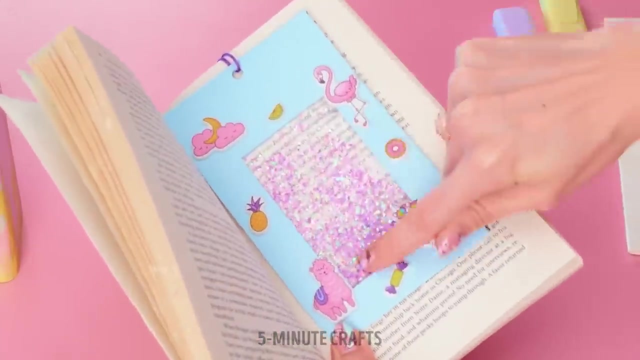 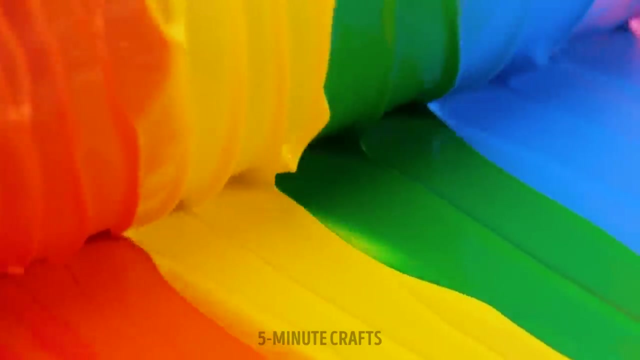 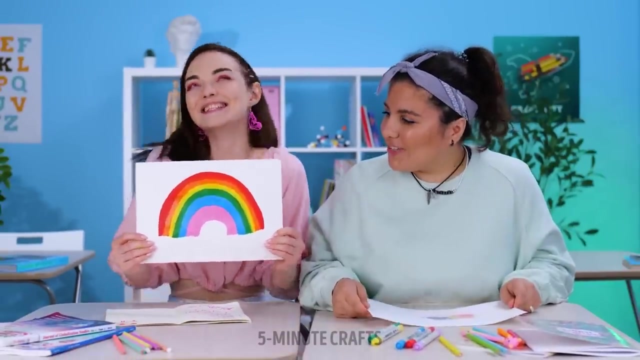 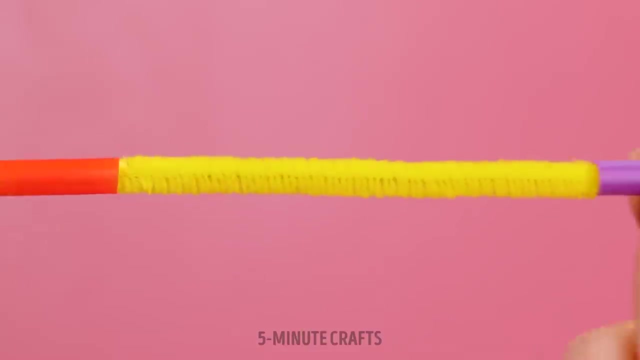 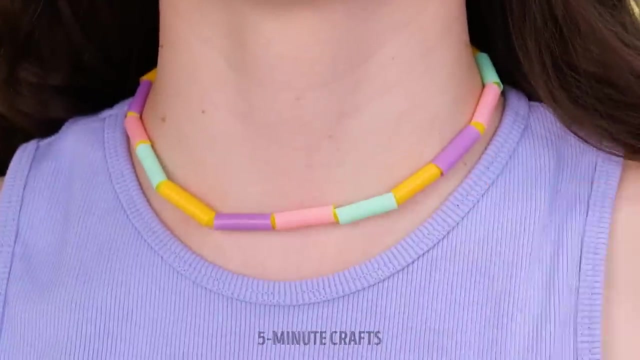 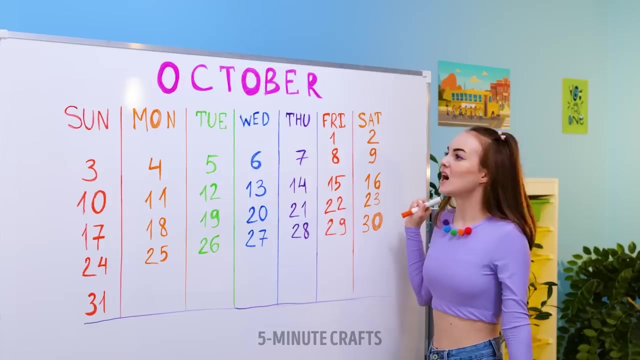 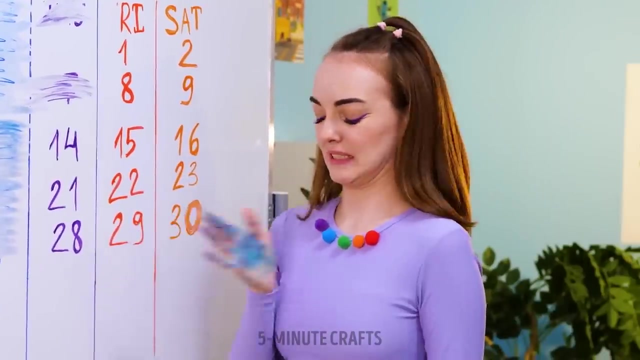 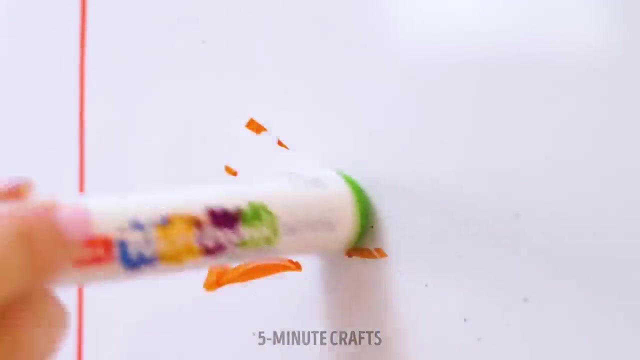 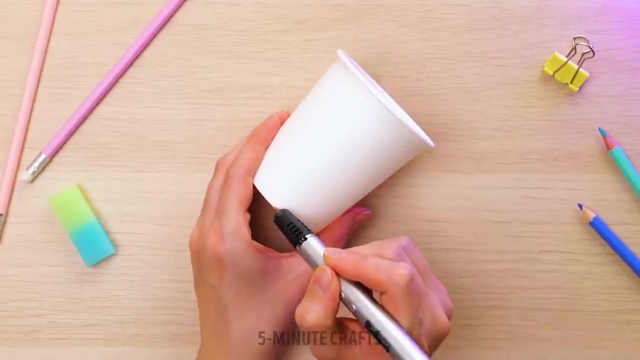 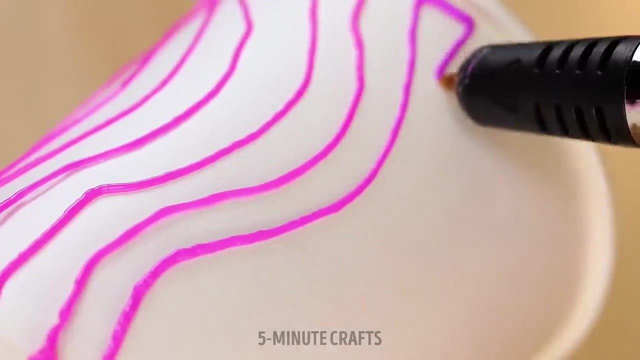 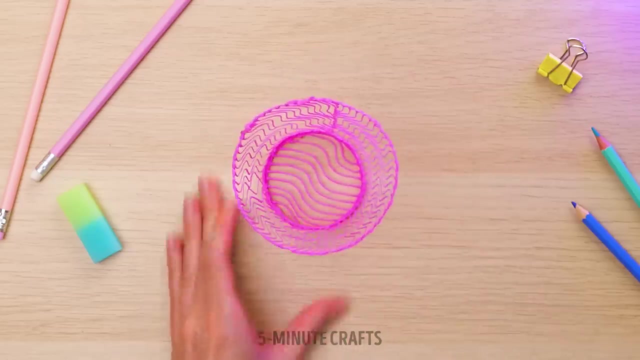 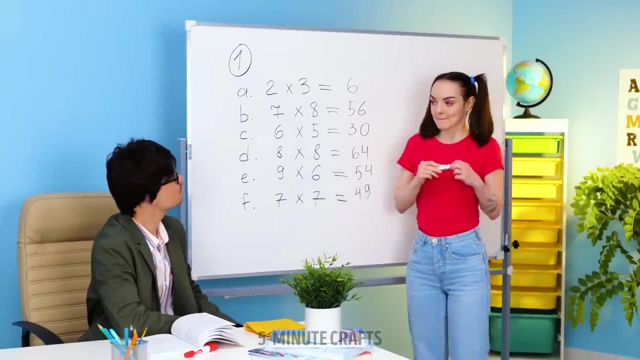 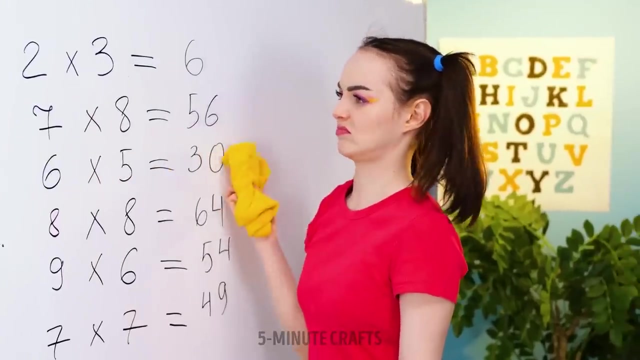 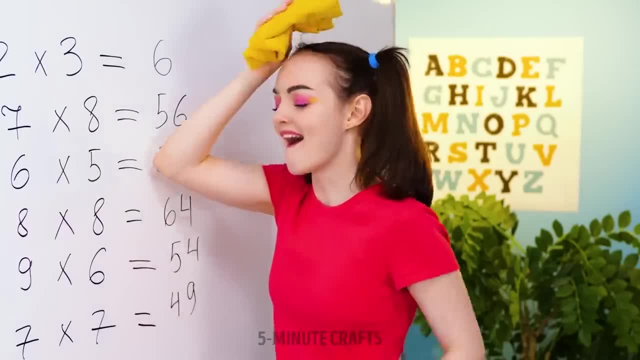 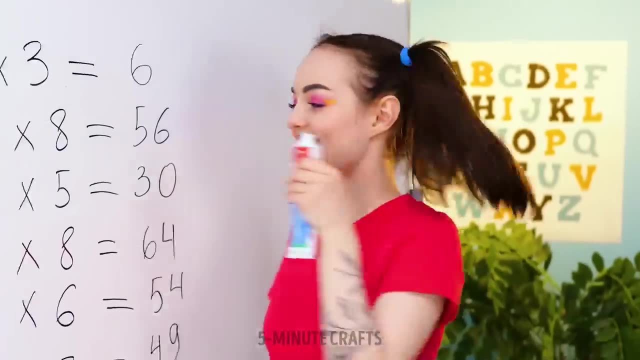 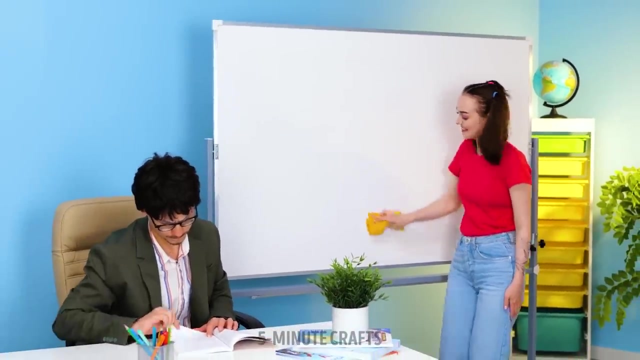 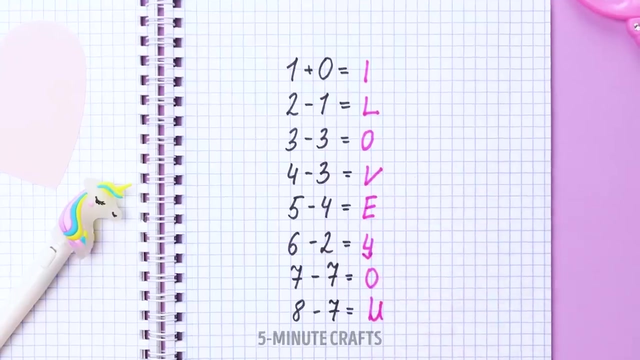 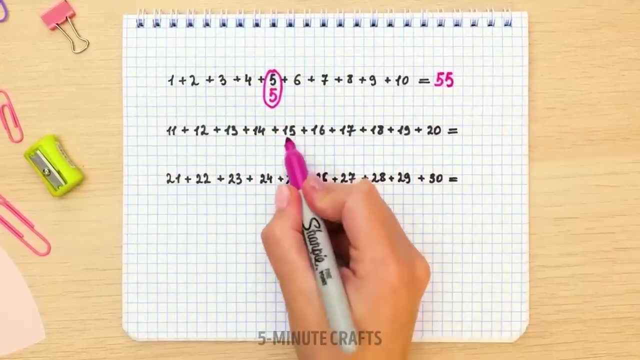 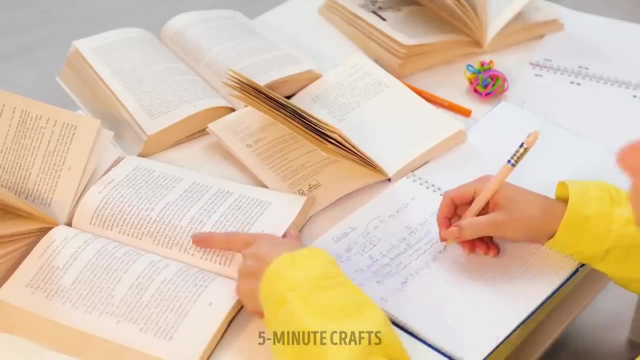 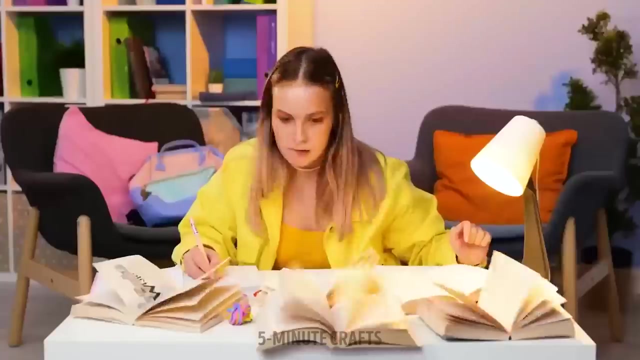 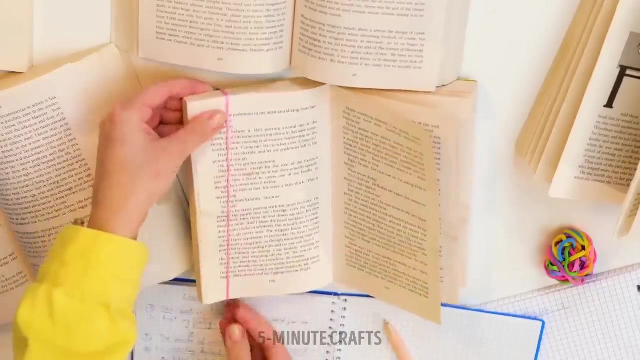 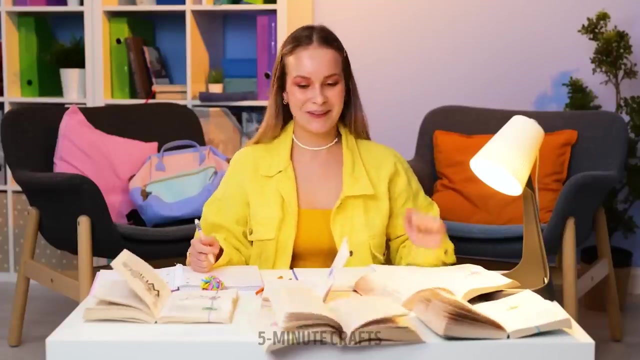 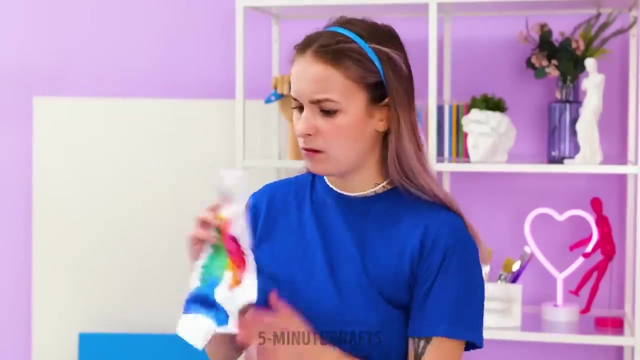 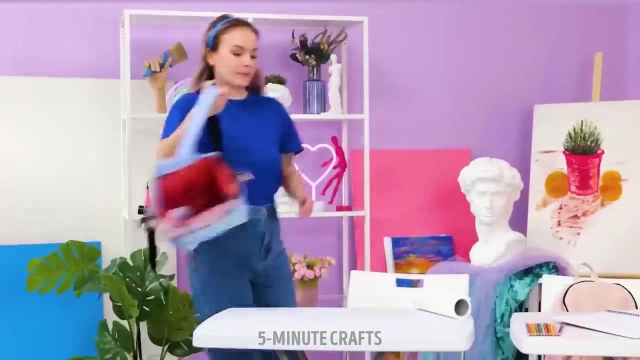 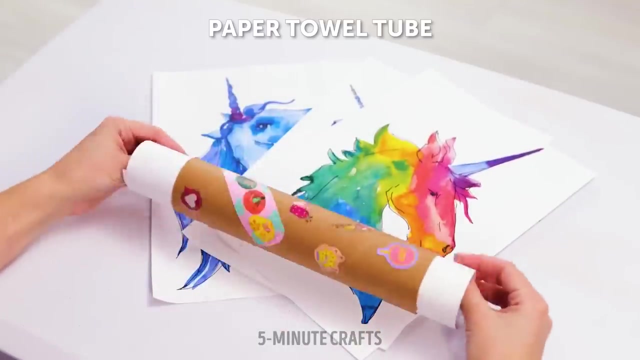 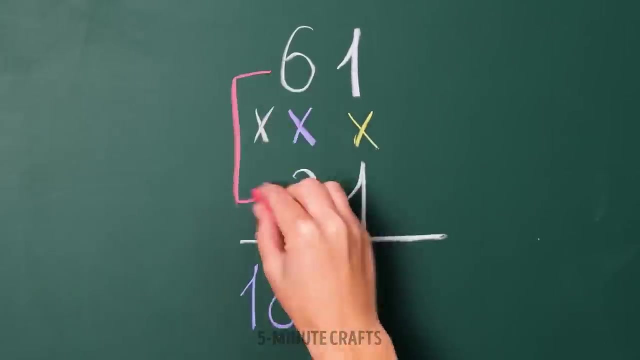 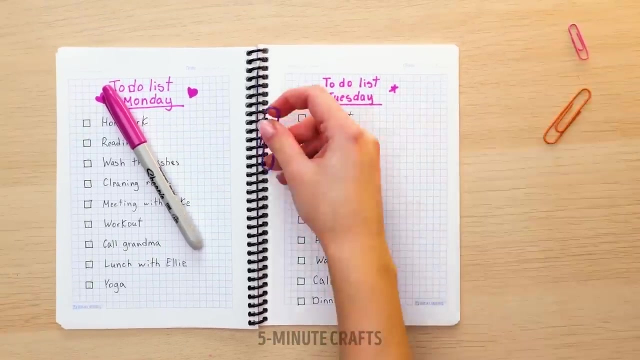 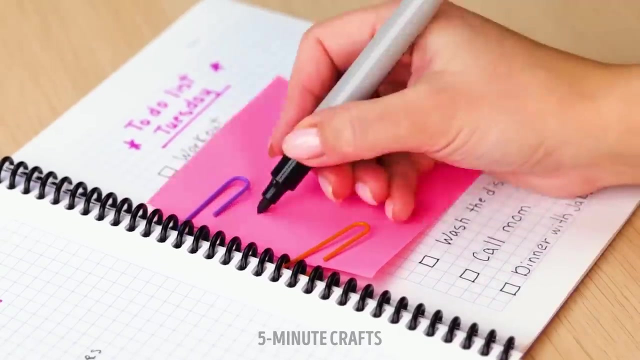 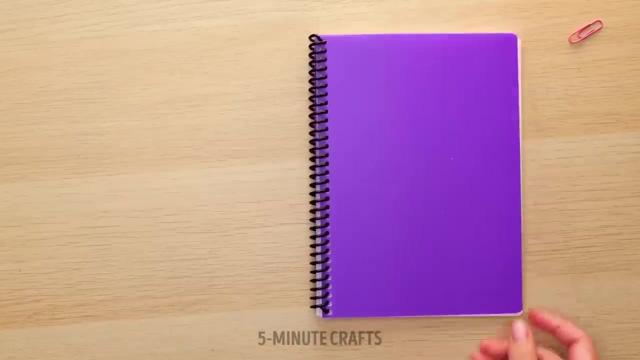 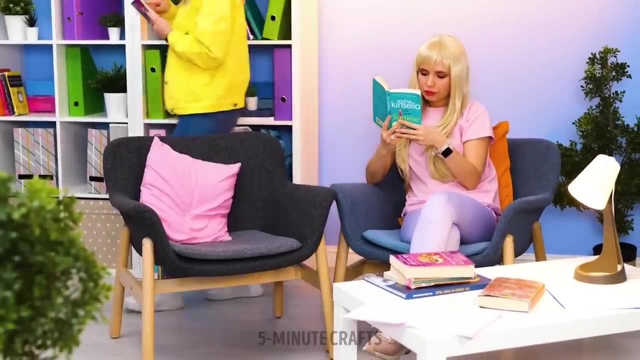 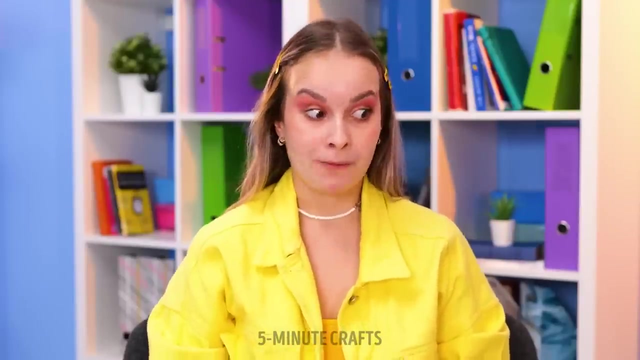 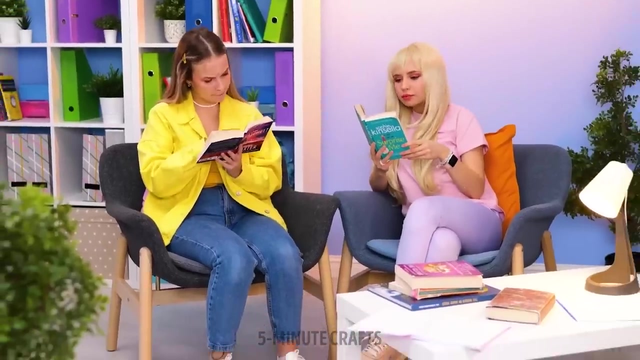 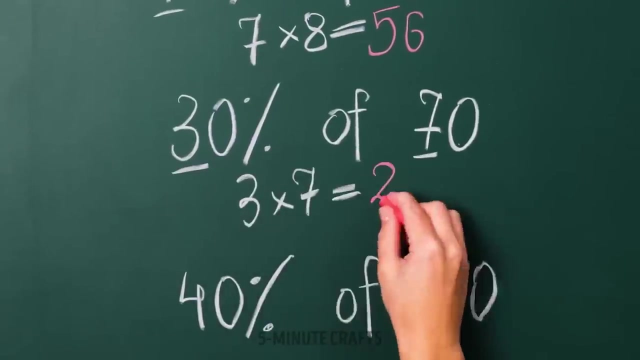 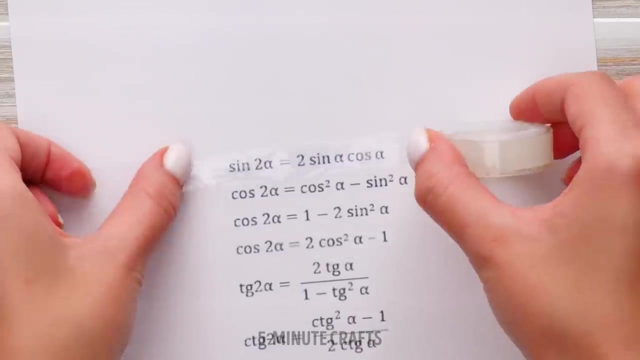 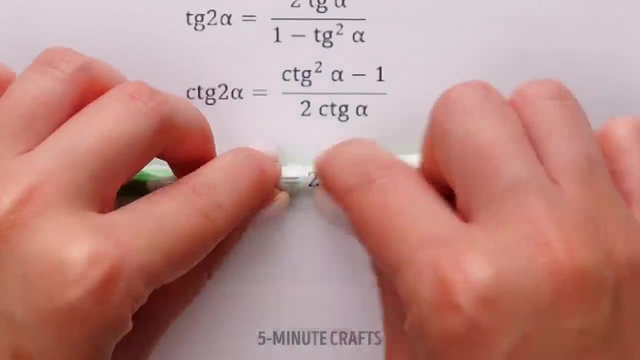 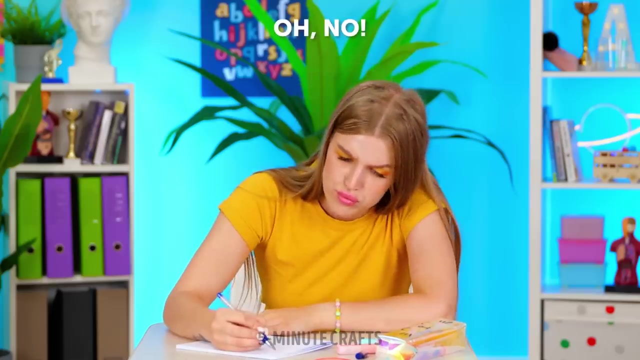 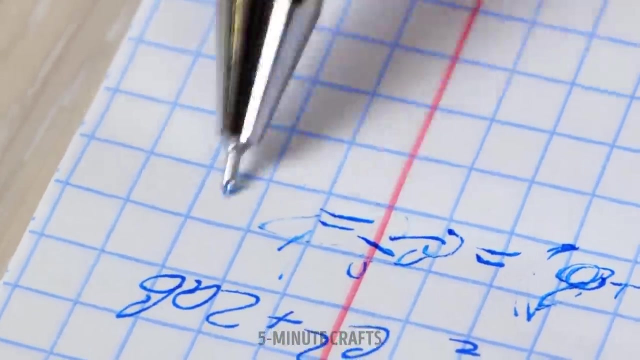 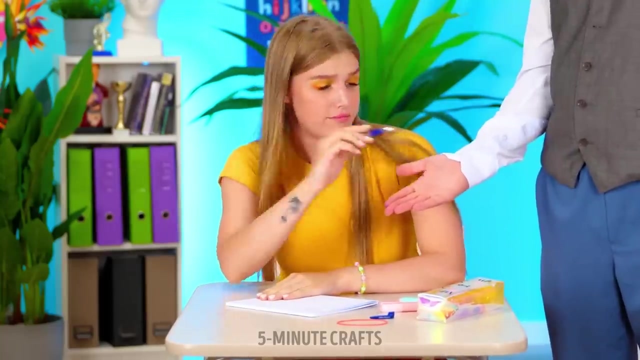 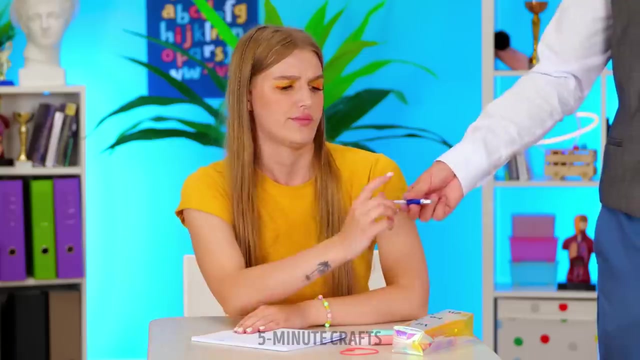 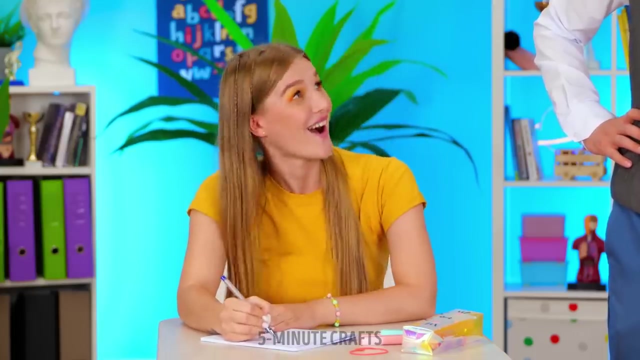 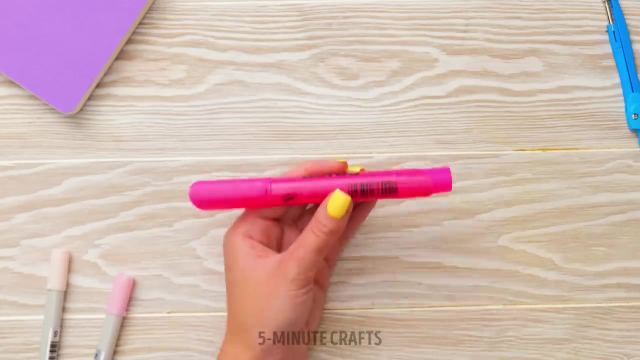 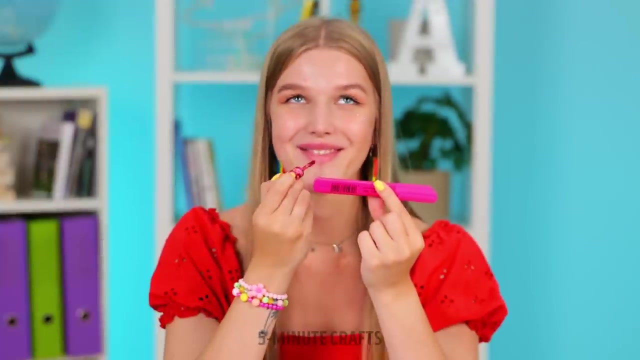 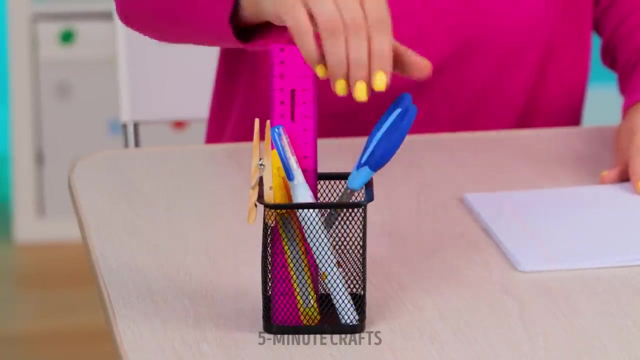 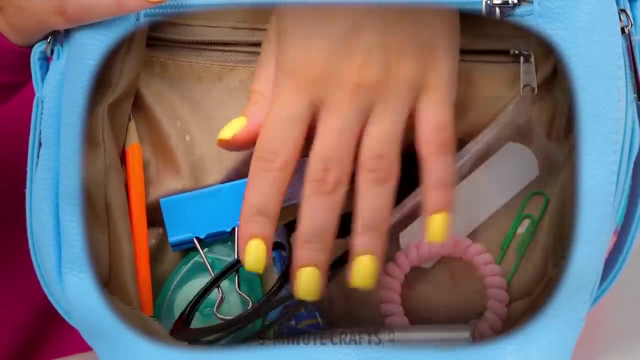 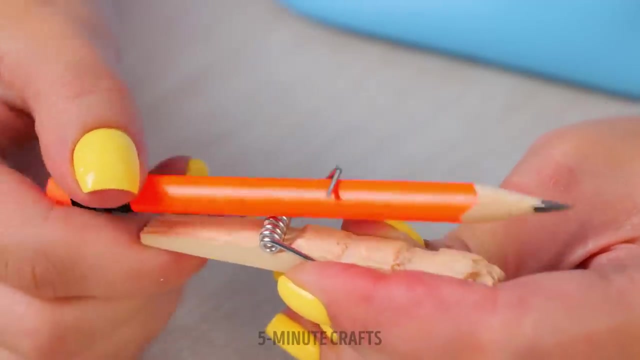 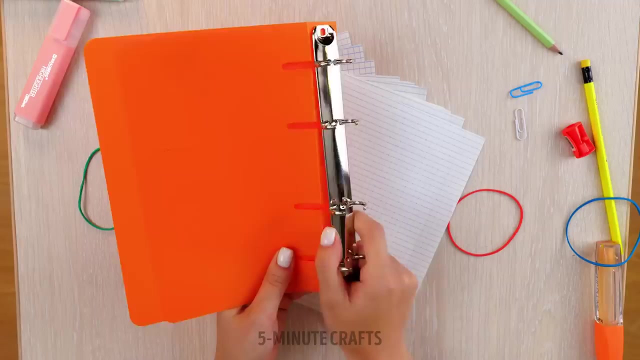 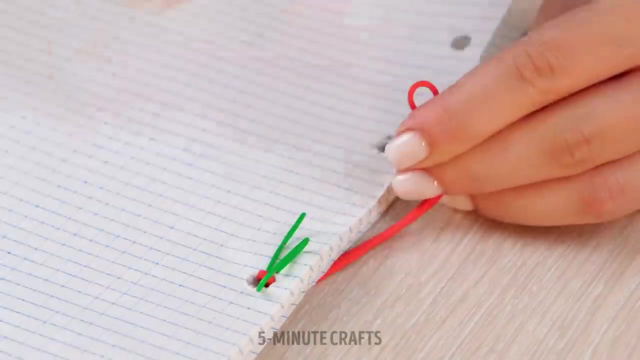 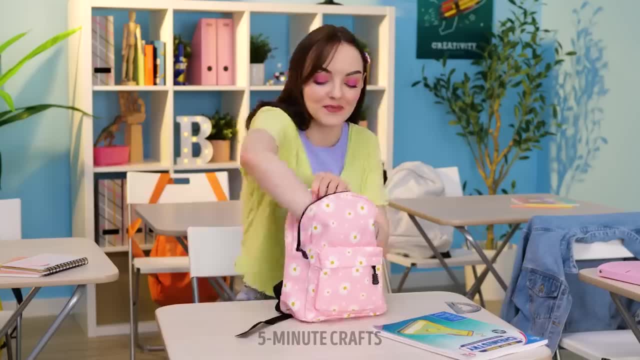 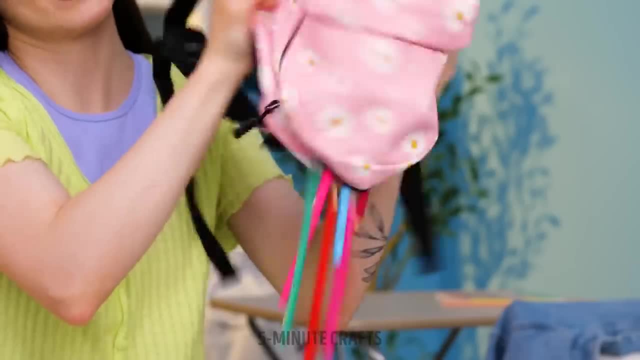 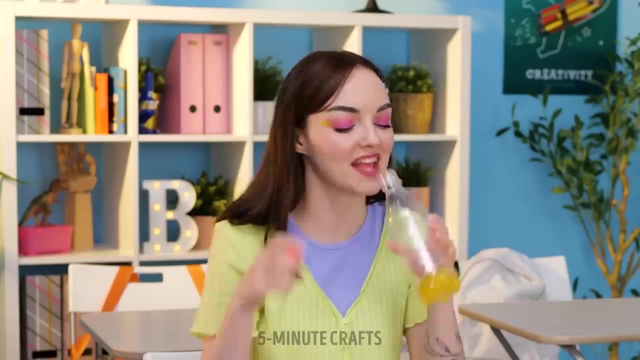 We gave it all. we gave it all Na-na-na-na-na-na, na-na-na-na-na. We say we love. we say we love Na-na-na-na-na-na, na-na-na-na-na. But we were just gonna stay until something better came along. 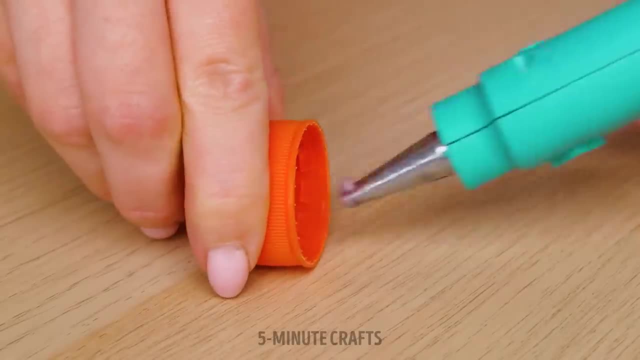 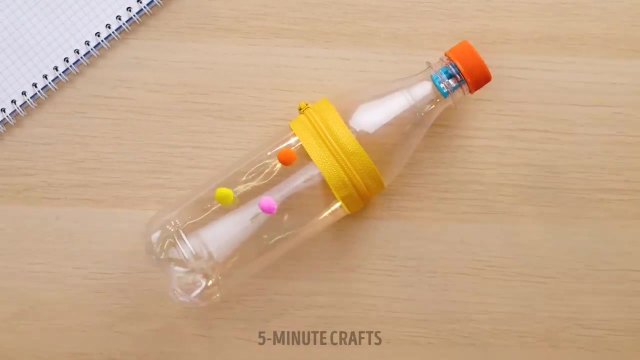 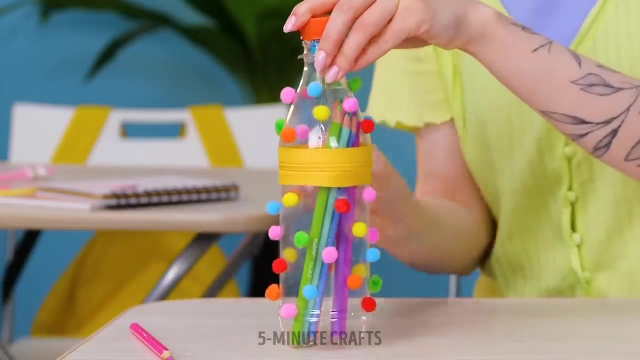 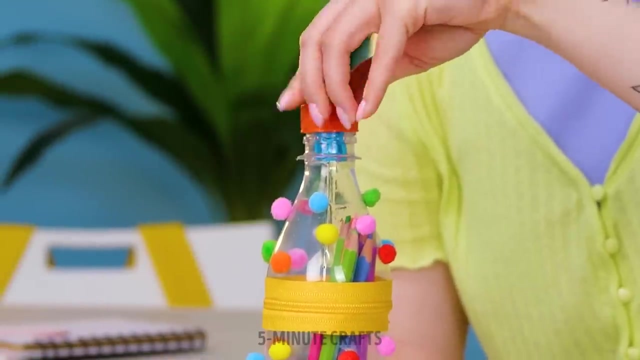 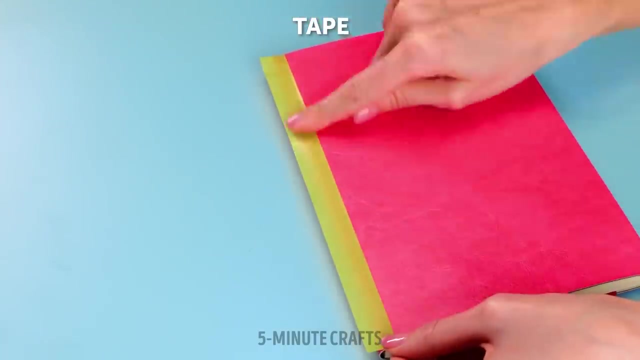 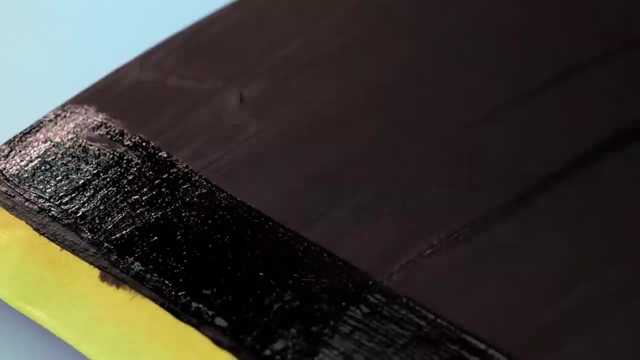 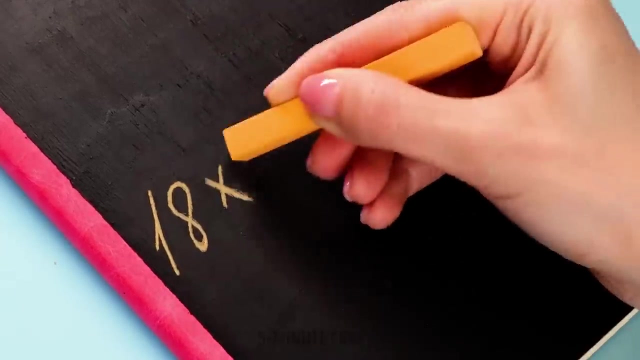 Na-na-na-na-na-na, na-na-na-na-na, Your body speaks my language and you read it like a book. This night means forever, and so does me and you. Na-na-na-na-na-na, na-na-na-na-na, We say we love. we say we love. 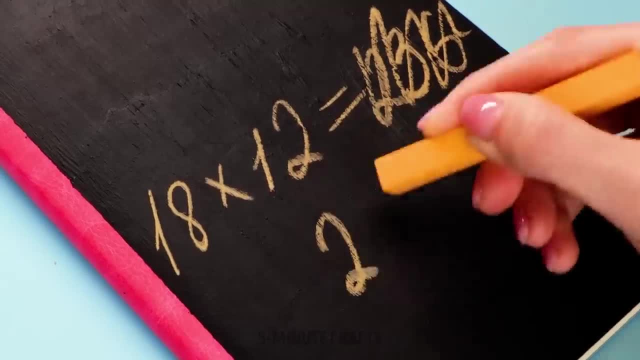 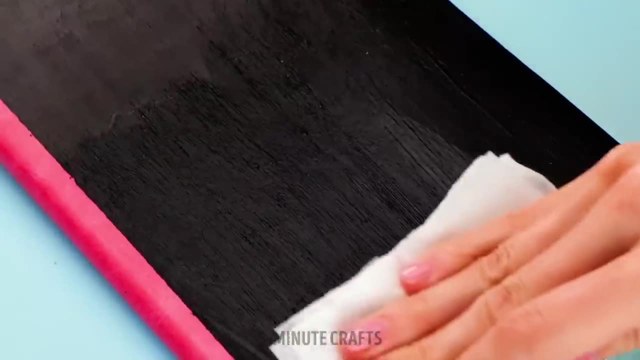 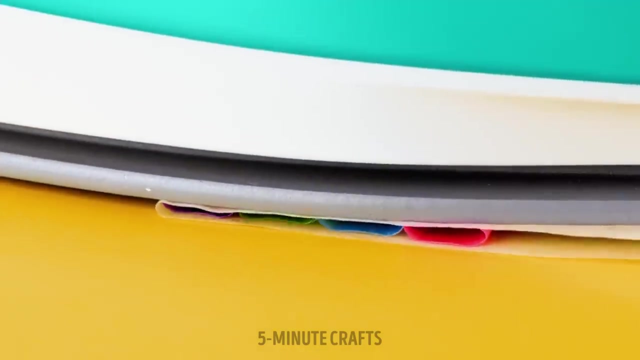 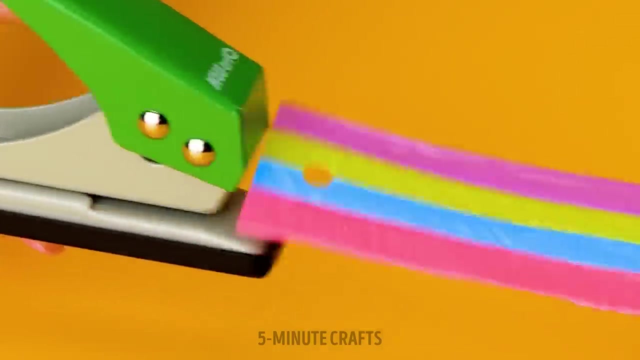 Na-na-na-na-na-na, na-na-na-na-na. We gave it all. we gave it all Na-na-na-na-na-na, na-na-na-na-na. We say: we love Na-na-na-na-na-na, na-na-na-na-na, But we were just gonna stay until something better came along. 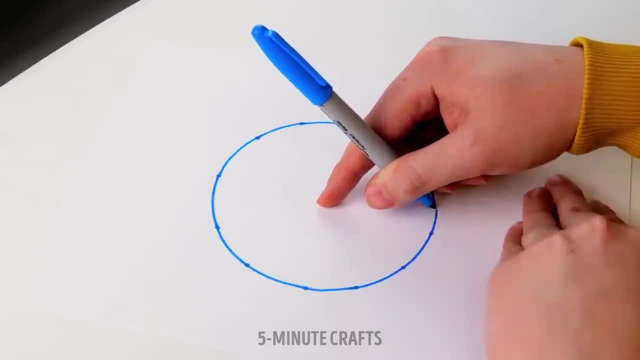 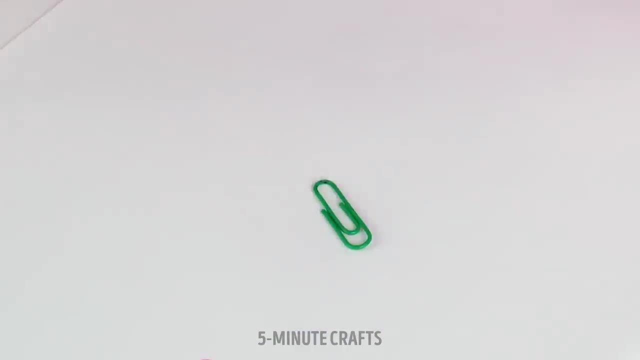 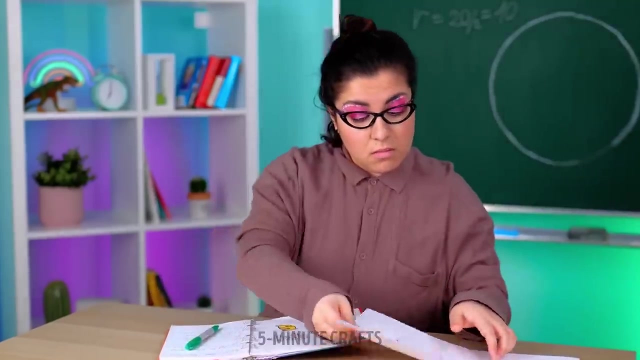 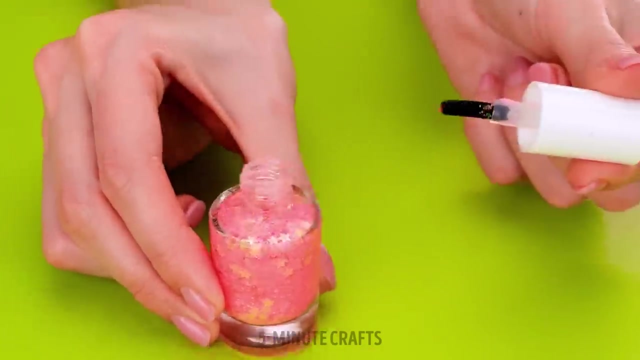 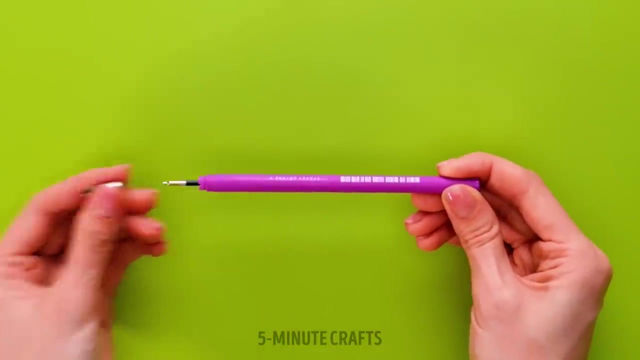 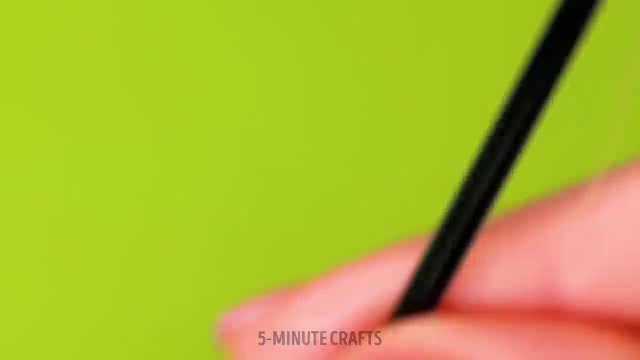 Na-na-na-na-na-na, na-na-na-na-na, Don't look back. My mama always used to say: You fucked me up And there's love. it's coming. I'll be sure of that, But it's so hard Cause it's you. it's you always on my mind. 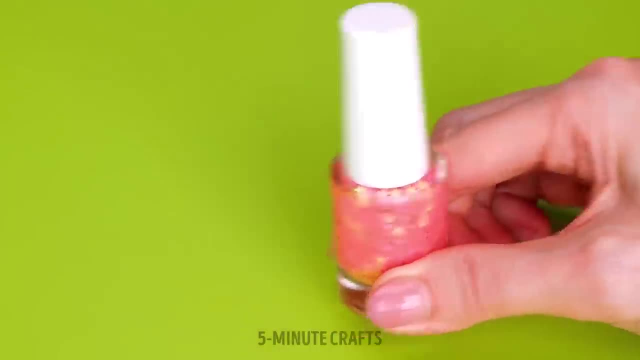 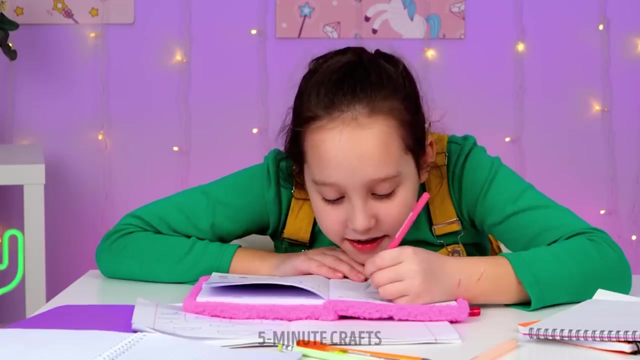 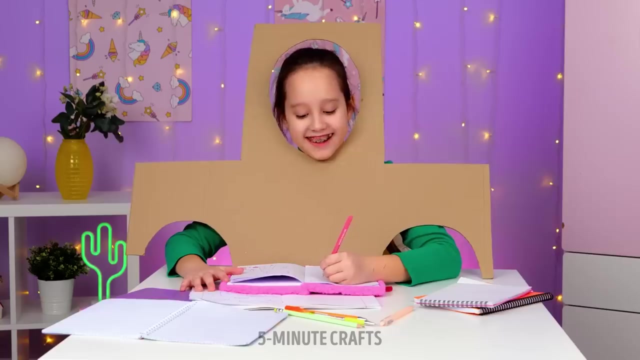 Yeah, it's you. it's you taking all my time. Let it sink in. haven't you been hurting enough? I give you all of my love, but you don't seem to care. But my heart's around you, but your heart isn't there. 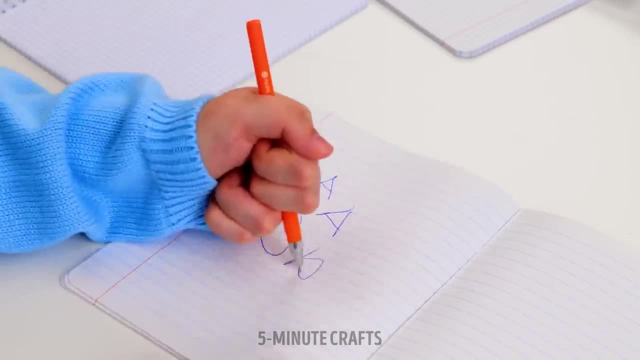 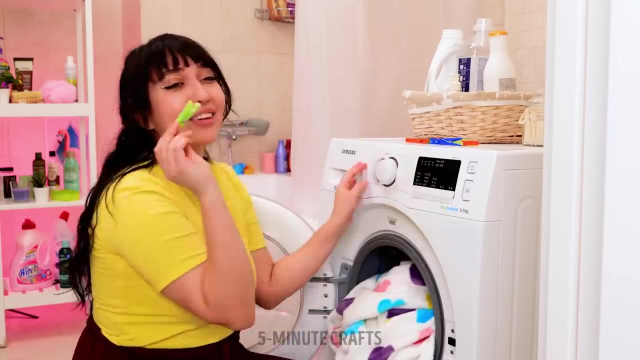 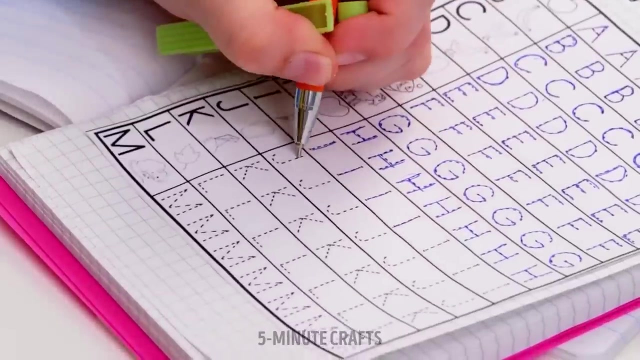 Don't tell me we're fine lying to yourself. It's so late to meet up, we are too far apart. It's so late, can't you see? I can't trust you no more. Gotta get over you, cause I'm more than the dark. 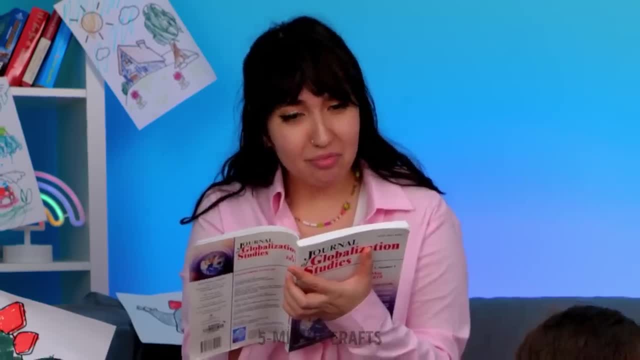 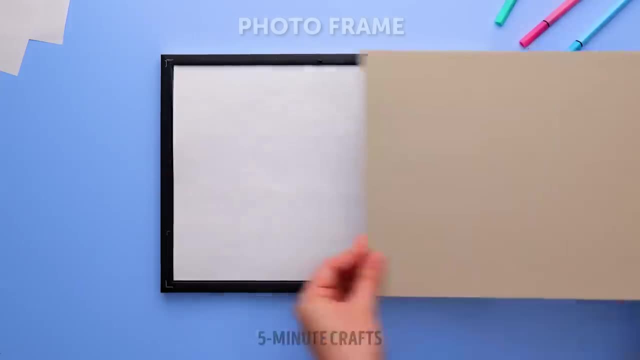 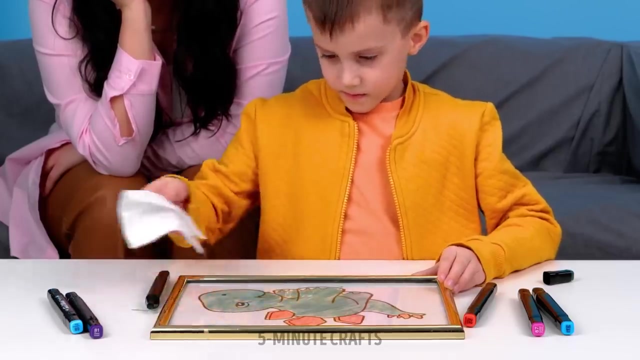 It's so late, can't you see? I can't trust you no more. It's so late, can't you see? I can't trust you no more. It's so late to meet up. Don't go there, cause you can't finish what you start. 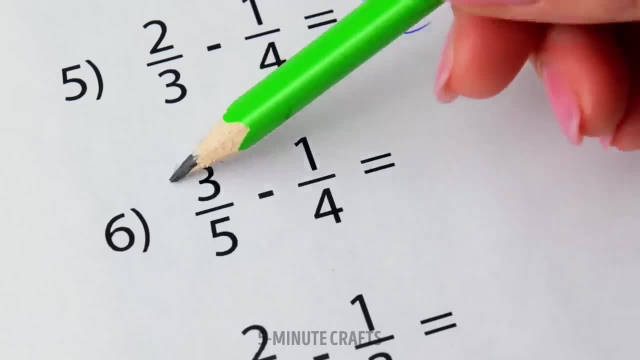 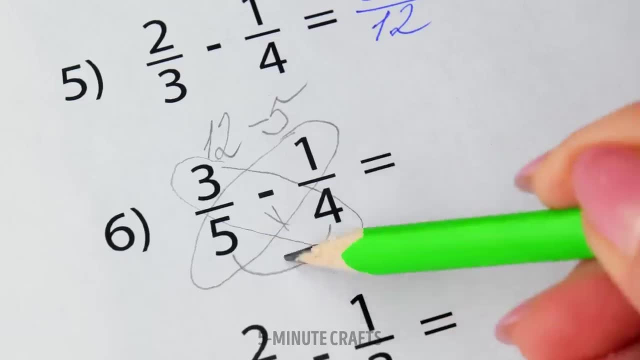 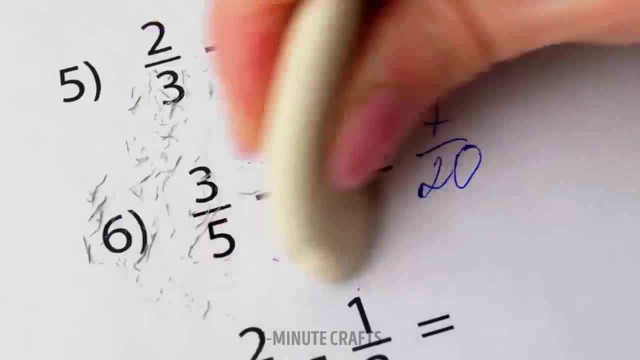 I can't keep up. Oh, then you're back, And then you're back. Don't let it go to far, just stay away, Cause it's you. it's you always on my mind. Yeah, it's you. it's you taking all my time. 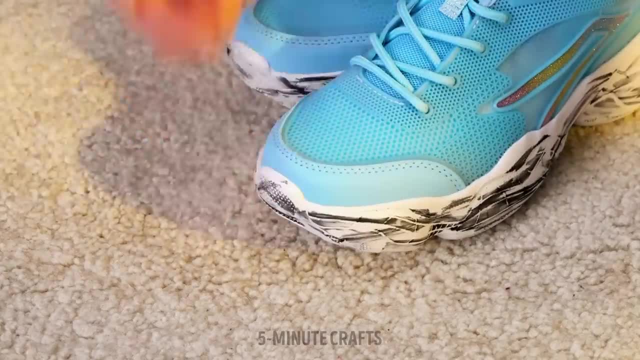 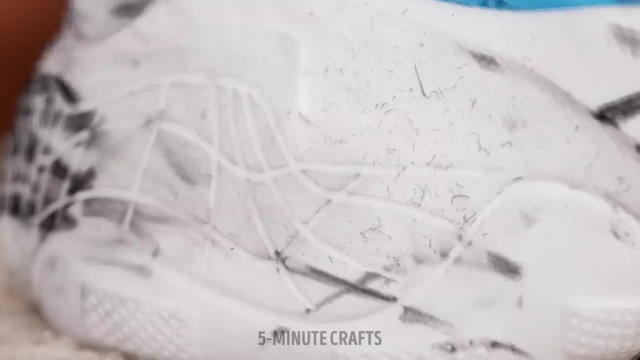 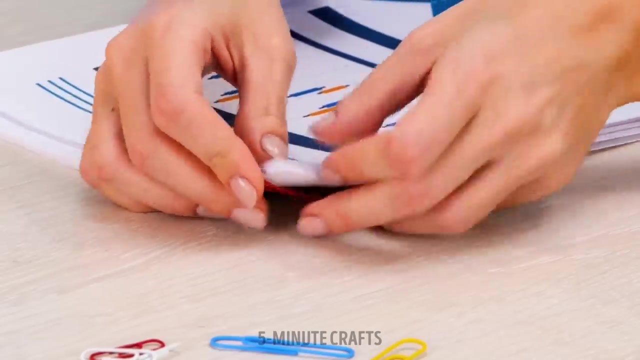 Let it sink in. haven't you been hurting enough? I give you all of my love, but you don't seem to care. But my heart's around you, but your heart isn't there. Don't tell me. we're fine Lying to yourself. 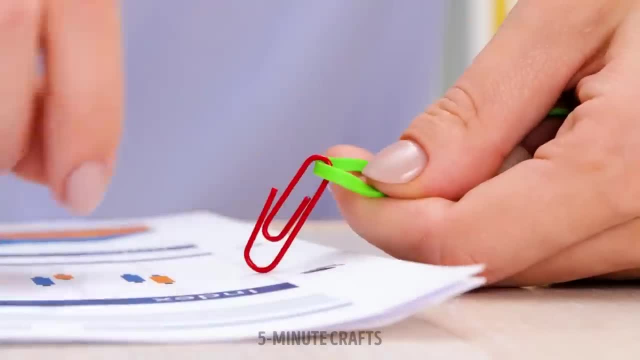 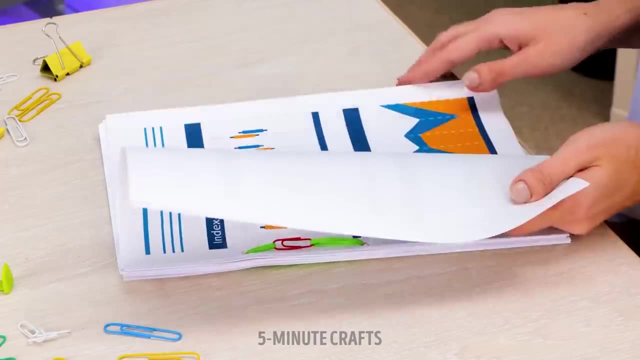 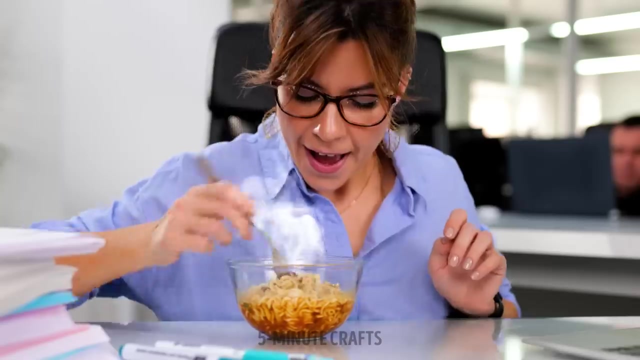 It's too late to meet up. we are too far apart. It's too late, can't you see? I can't trust you no more. Gotta get over you, cause I'm more than the dark. It's too late to meet up. Too late to meet up. 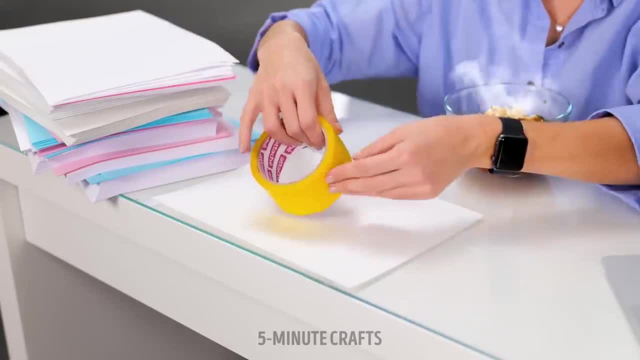 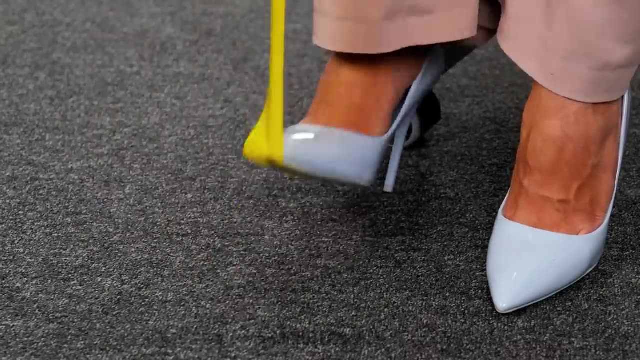 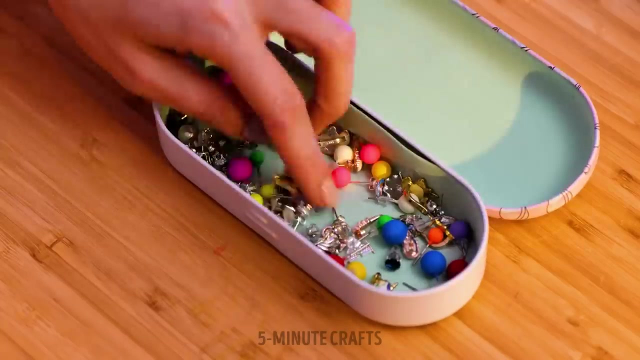 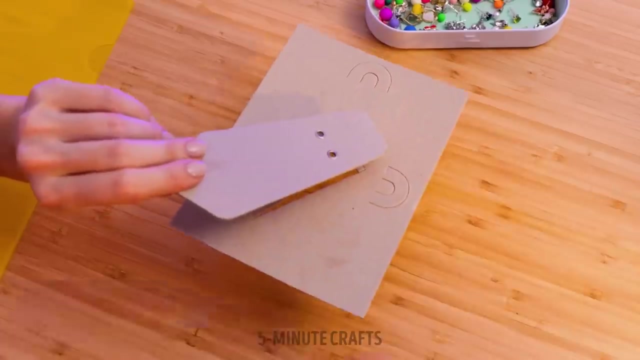 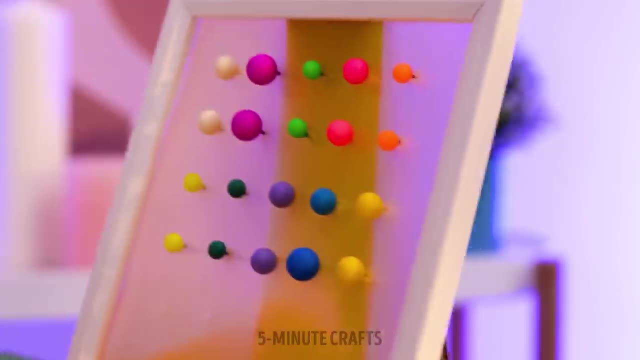 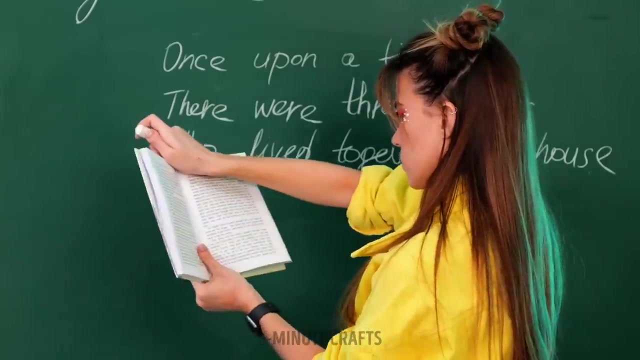 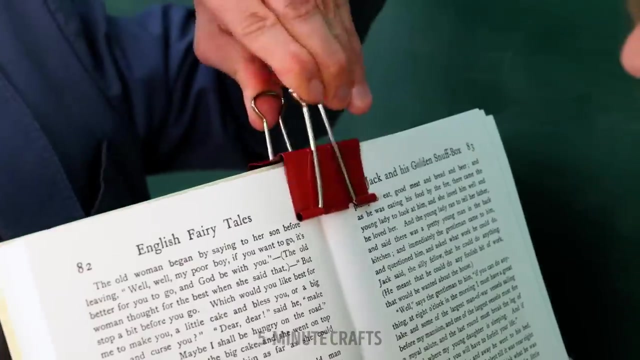 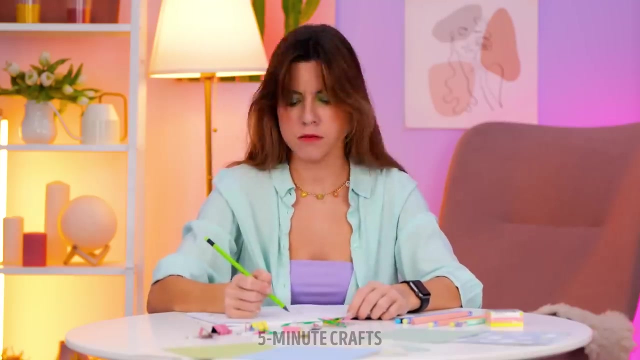 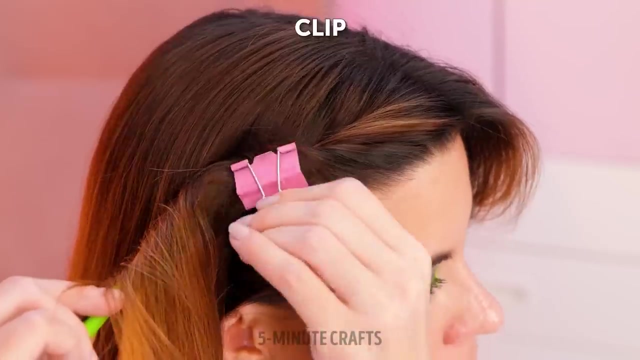 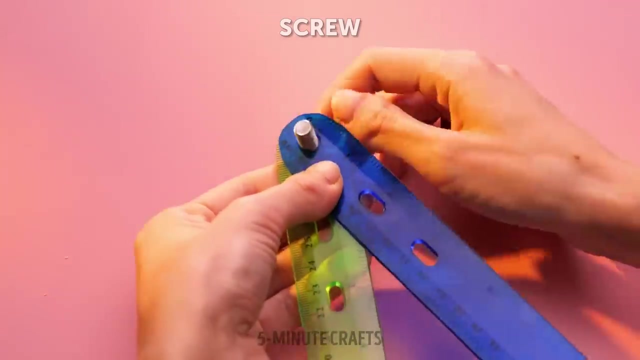 Too late to meet up? Too late to meet up. Too late to meet up. Woo, Work is almost over, summer's getting closer, No time to be sober. sunshine on my shoulders. I'm alive and breathing, living my best life, Lovin' my life, lovin' my life. 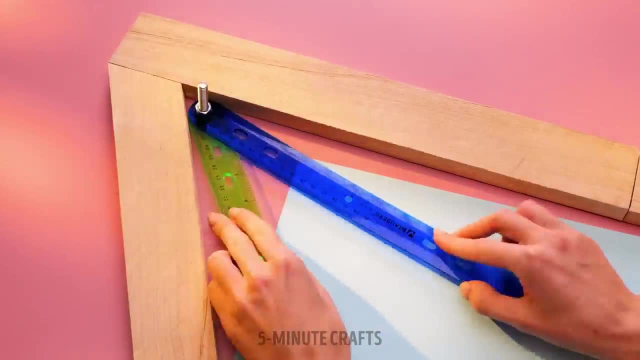 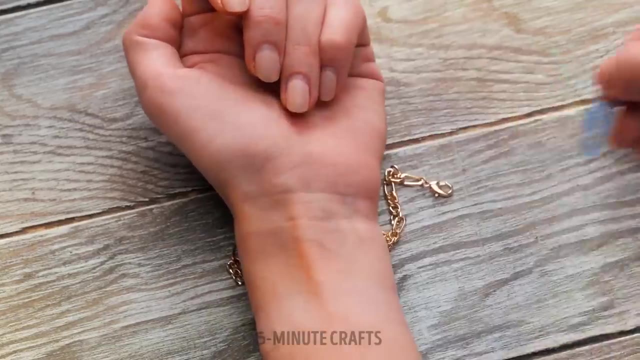 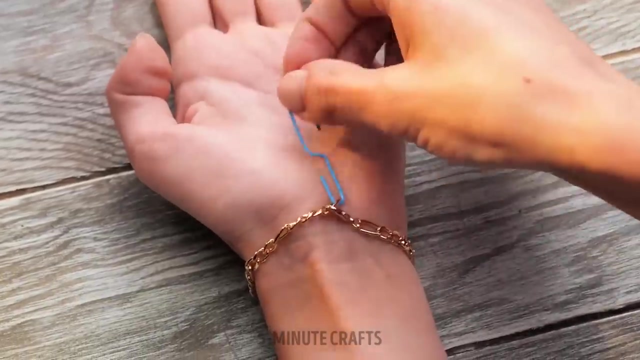 It's on my mind, it's taking me high. I'm staying in this moment, so it's hard sometimes, But I work it out every once in a while. I feel the love. I feel it growing every day. I feel the love. I feel the love. 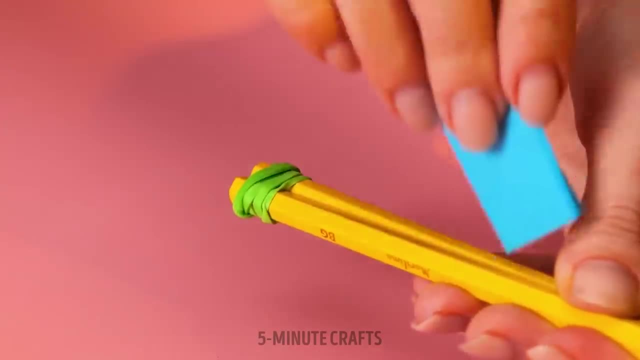 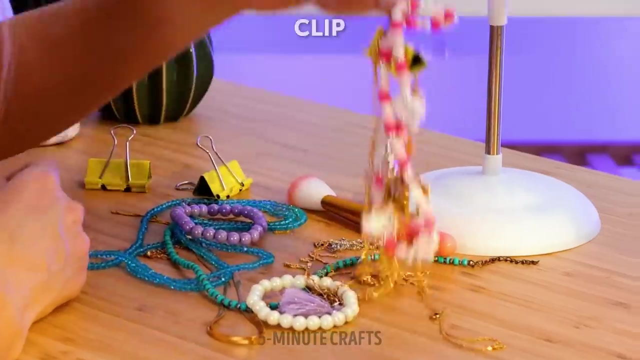 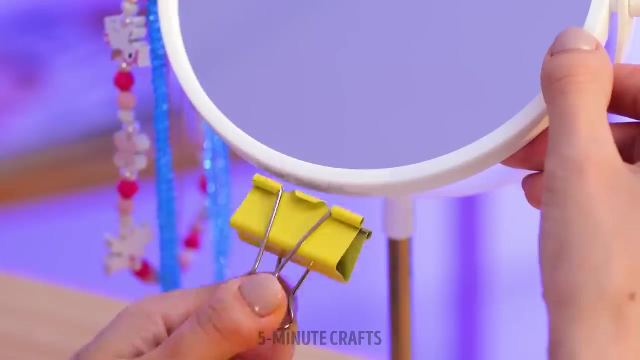 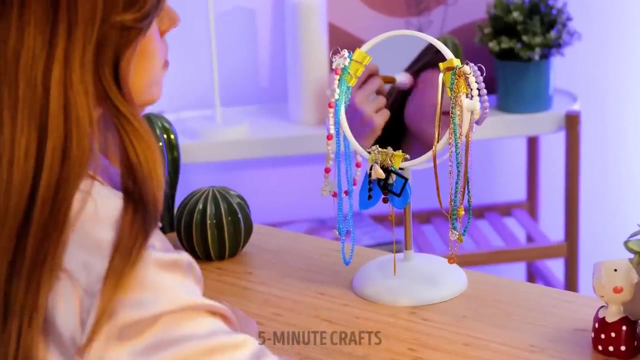 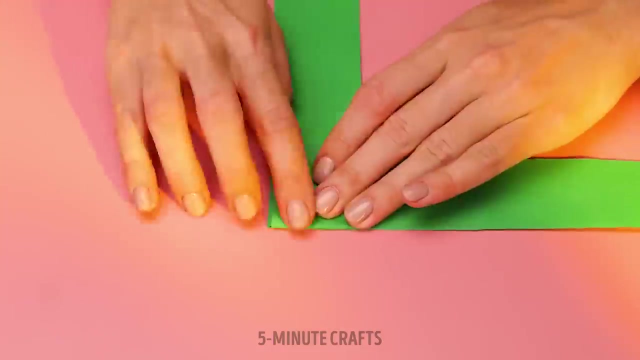 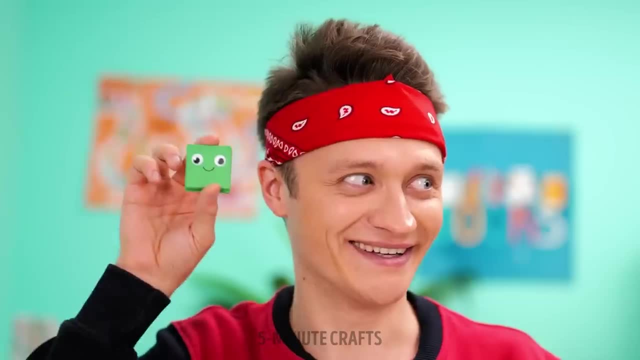 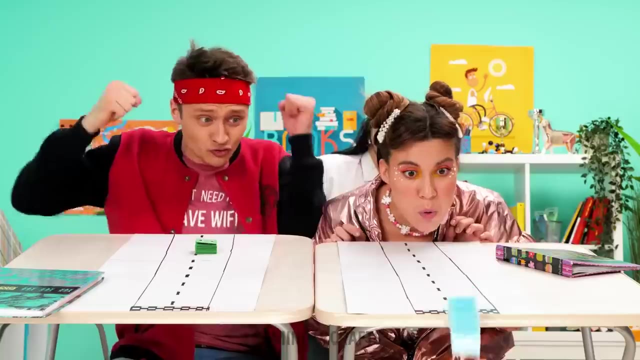 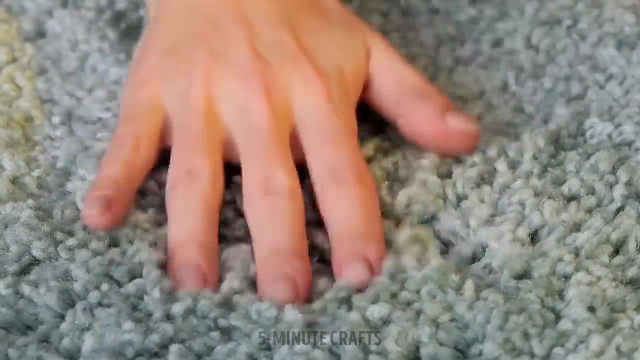 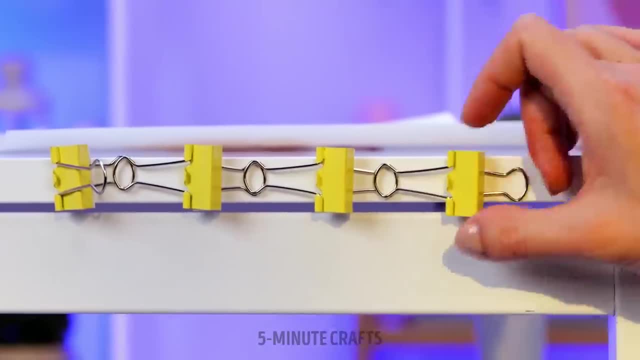 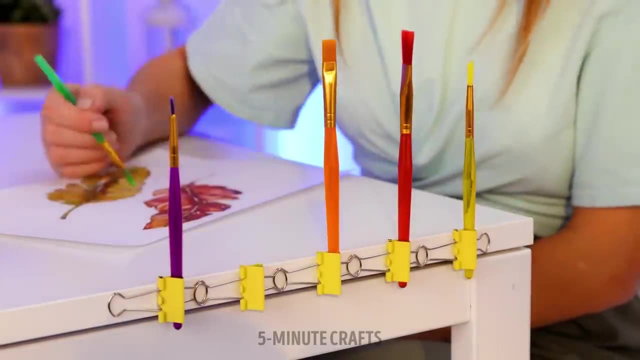 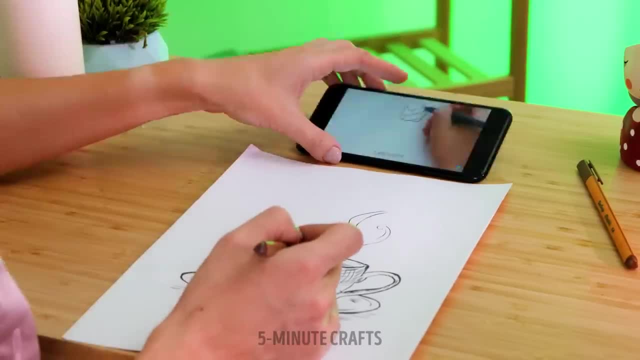 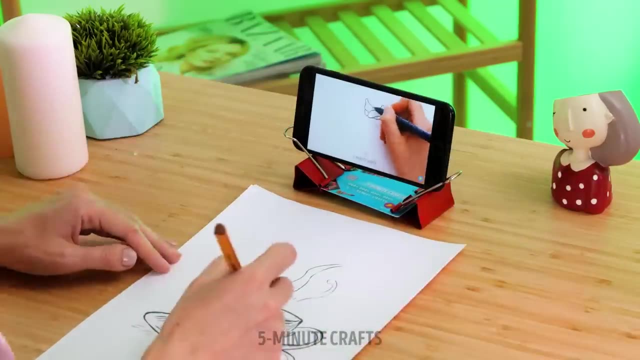 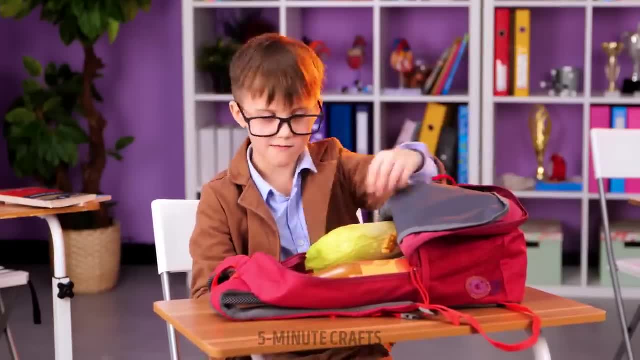 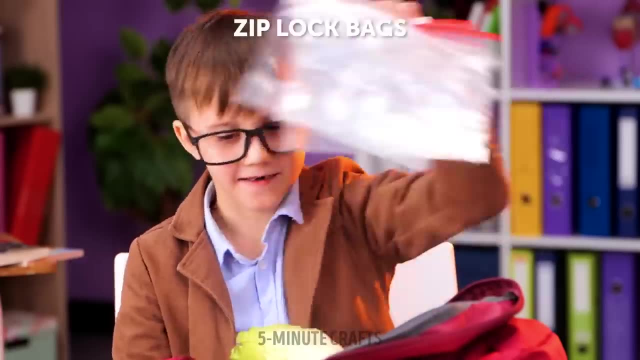 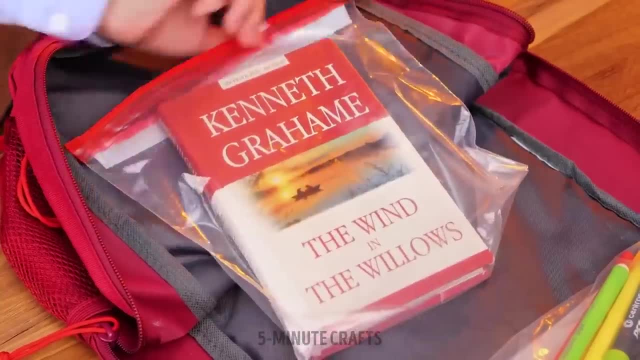 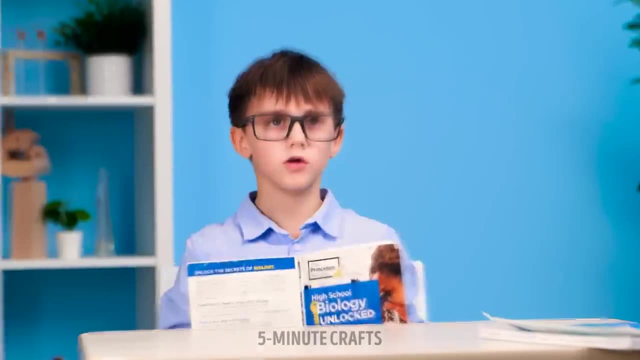 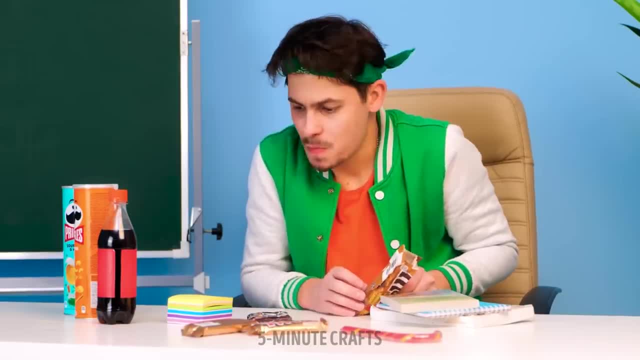 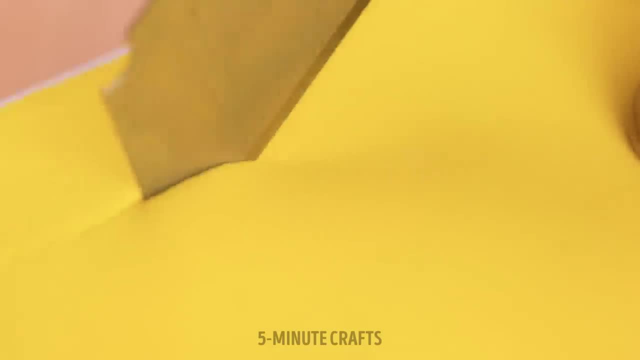 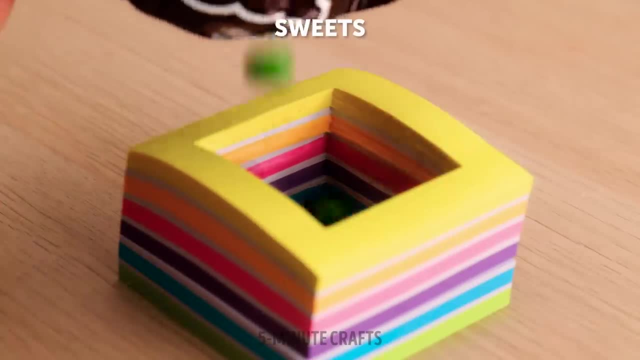 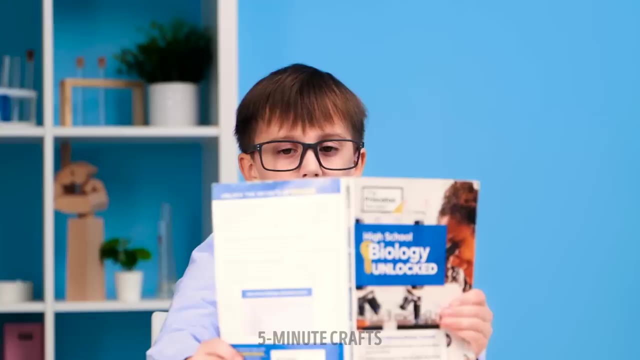 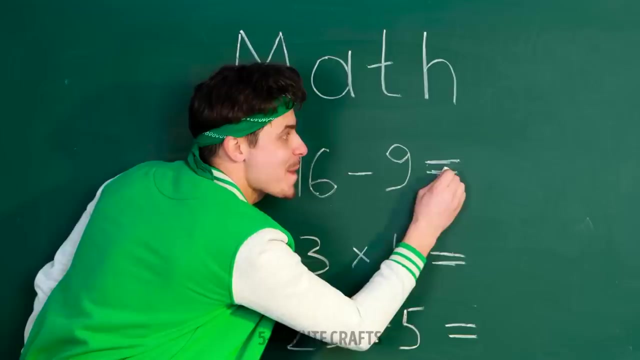 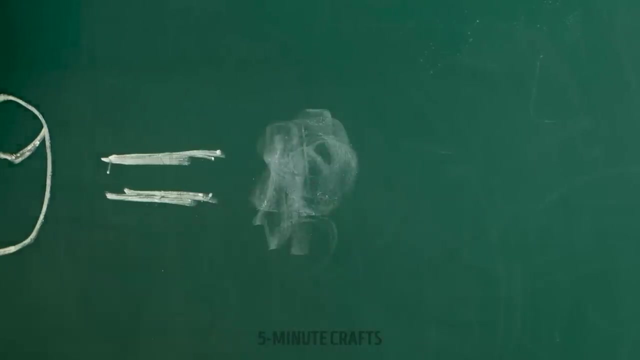 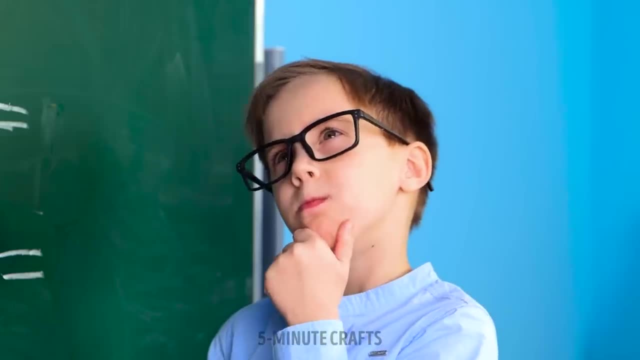 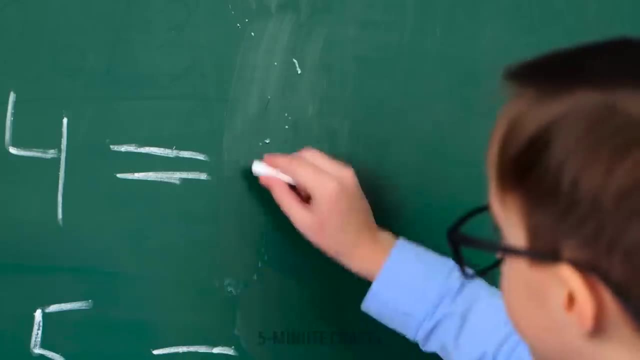 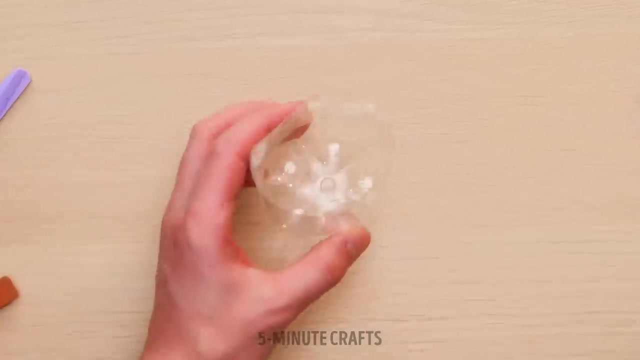 I'll call your friends. I'll let them know That I'm so done with the tragic boys. Tonight I'll get into my zone. I'll dance until the tears are gone. No time for bad love, bad love, bad love. I'm dancing all these tears away. 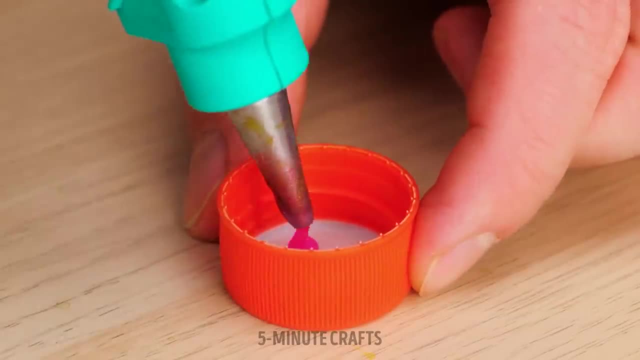 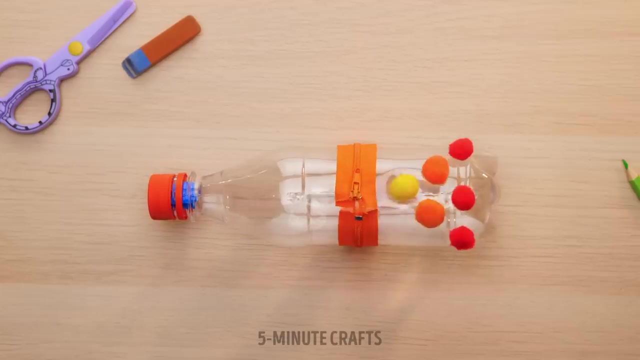 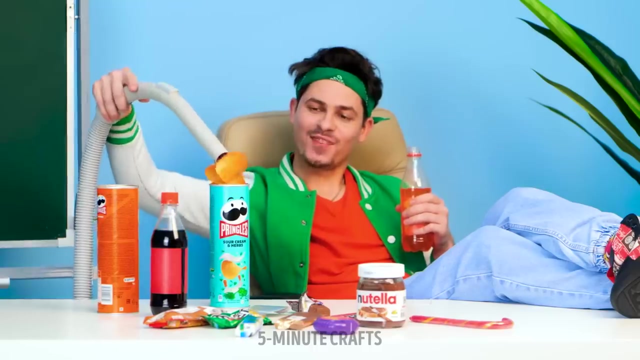 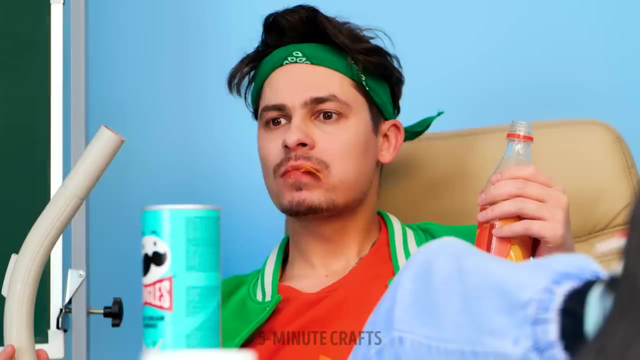 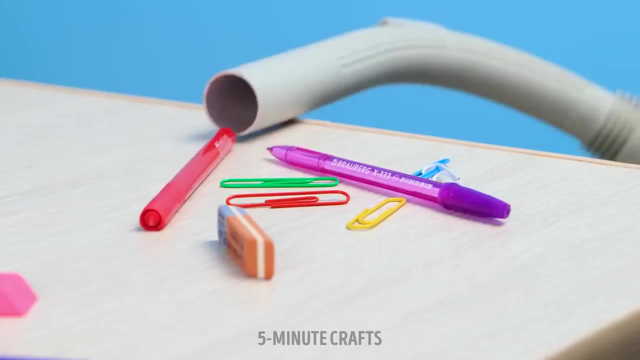 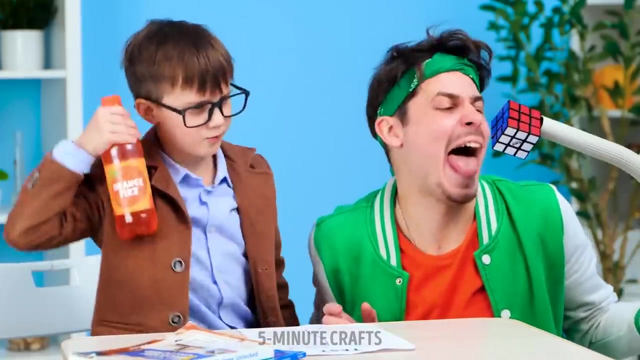 No time for bad love. bad love, bad love. I'm dancing all these tears away. Don't need ya, Don't need ya. Me and you just made me realize All the things I used to sacrifice Just to please you, just to call you mine. But look at me, now I have the time of my life. I'll call your friends. I'll let them know. I'll let them know I'm so done with your tragic boys Tonight. I'll get into my zone. I'll dance until the tears are gone. No time for bad love. bad love, bad love. I'm dancing all these tears away. 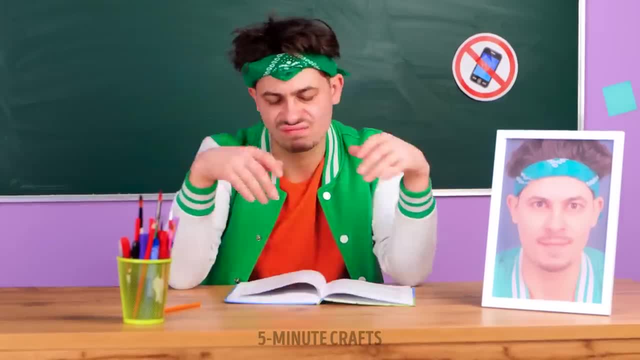 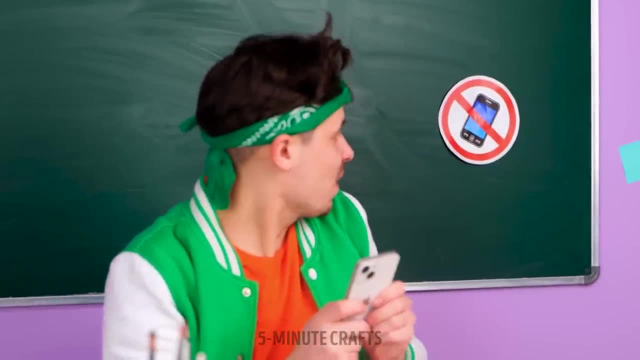 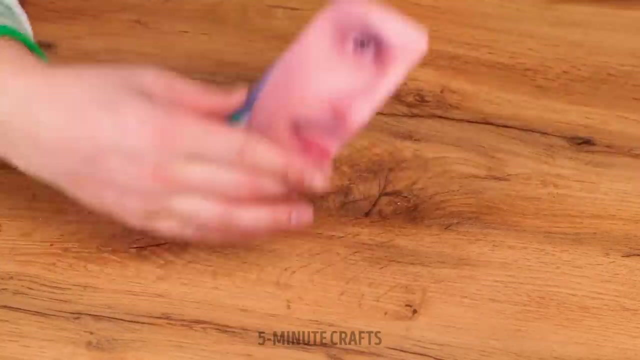 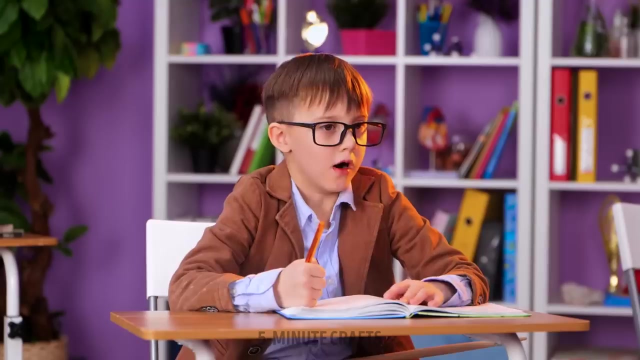 No time for bad love, bad love, bad love. I'm dancing all these tears away. Don't need ya, Don't need ya, don't need ya, no more, don't need ya, Don't need your, Don't need your, Don't need your Dancing all these days away. 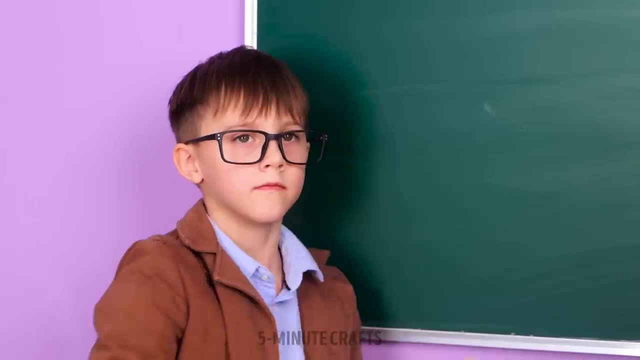 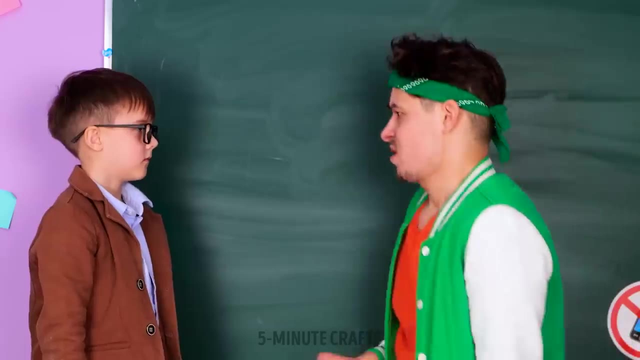 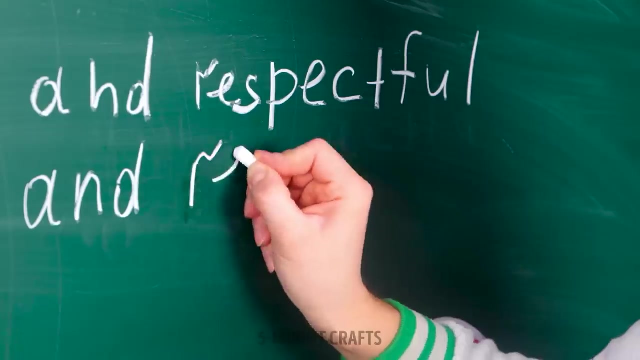 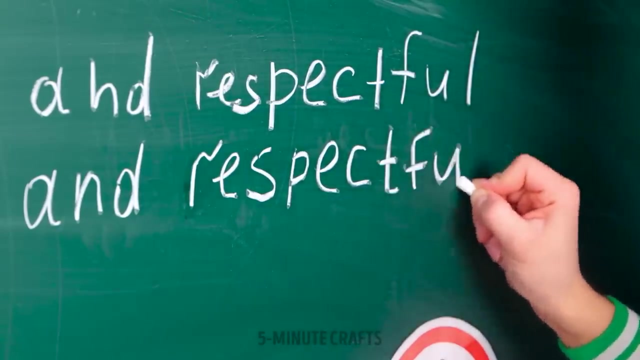 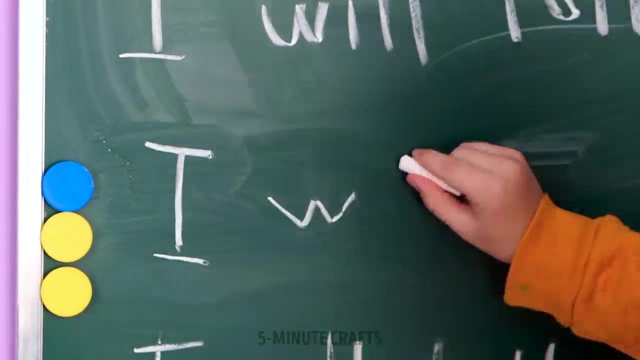 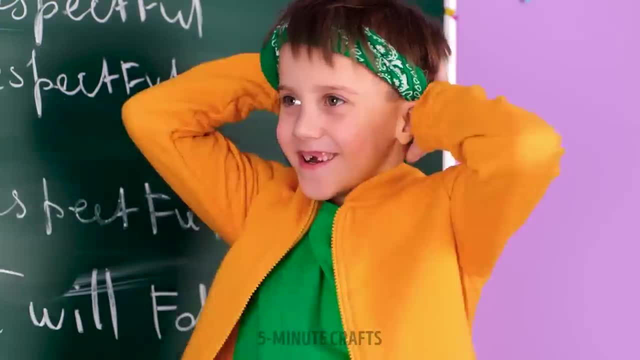 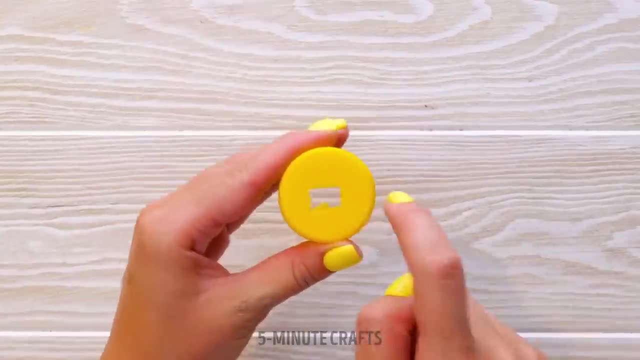 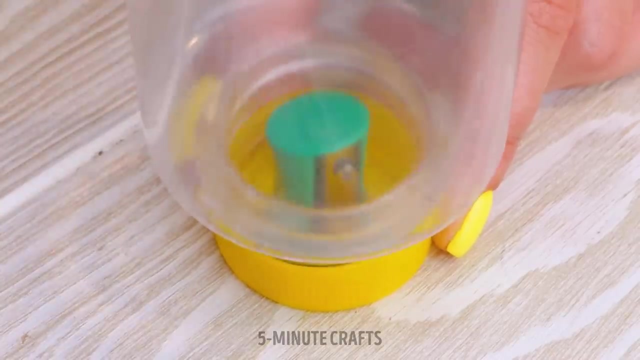 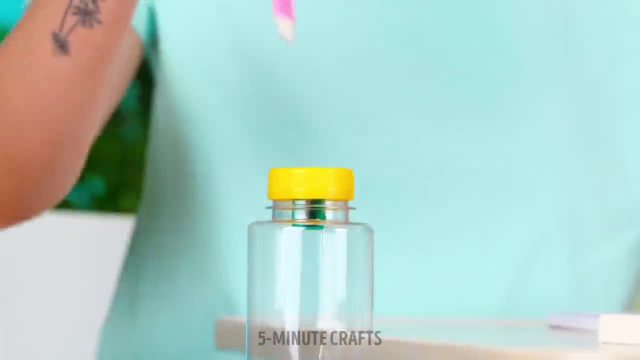 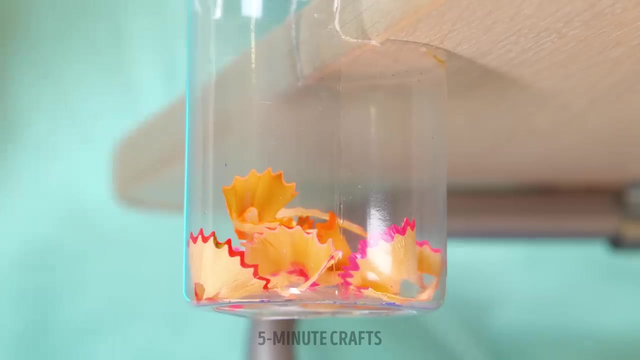 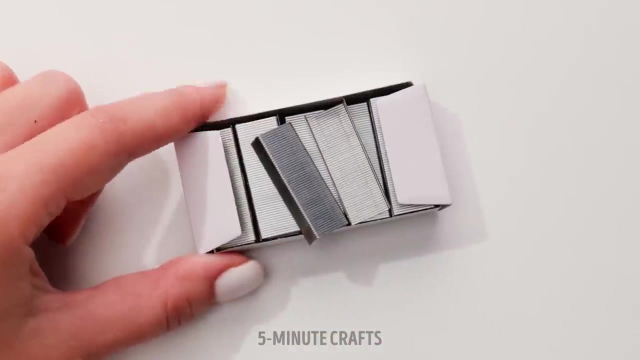 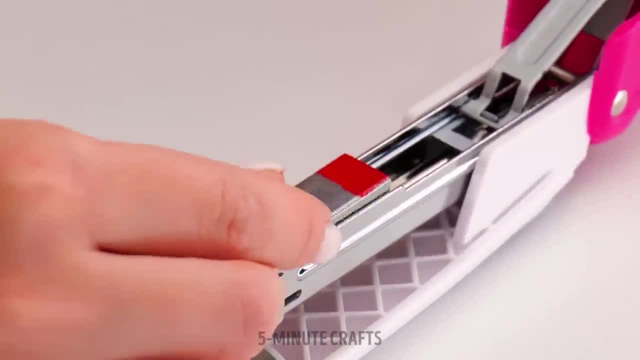 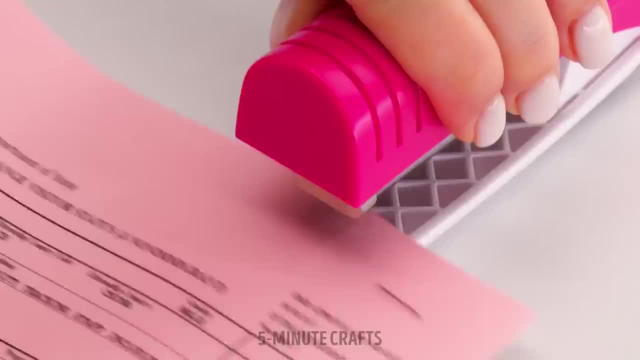 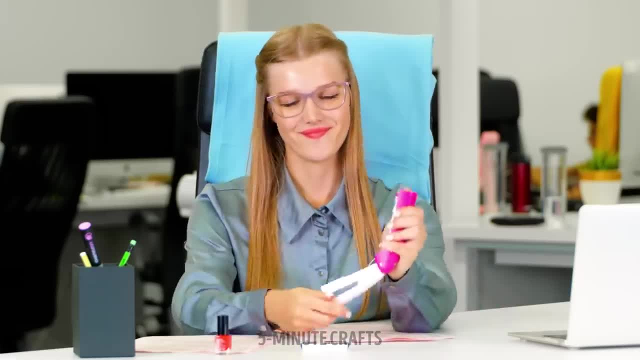 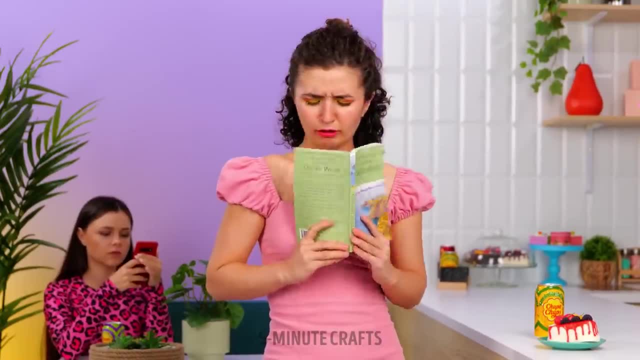 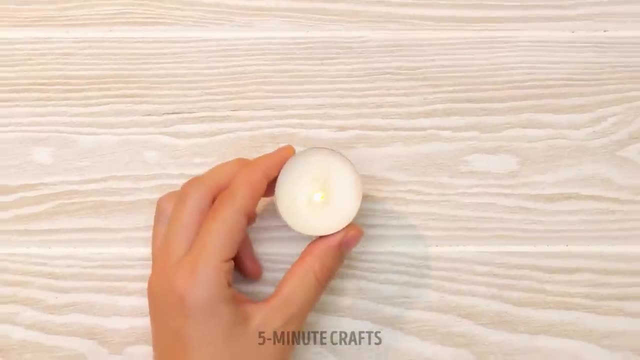 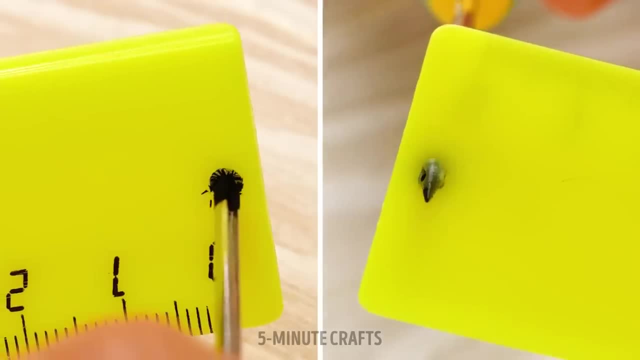 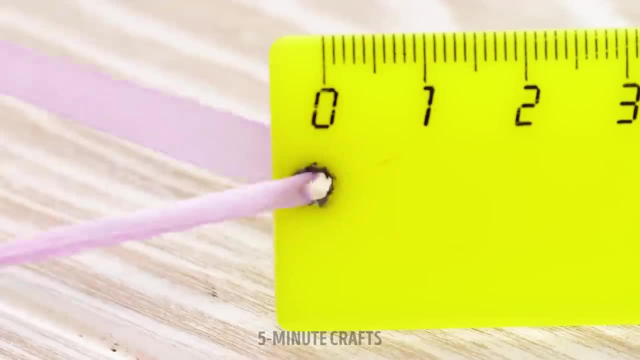 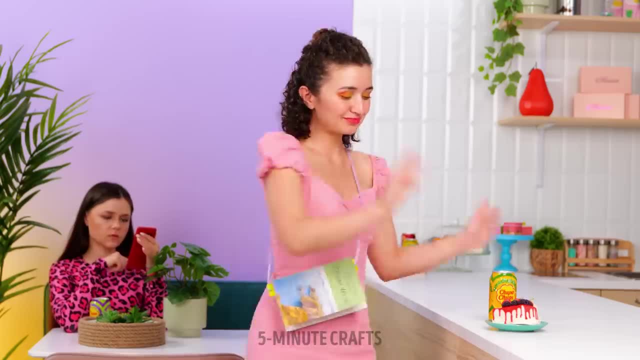 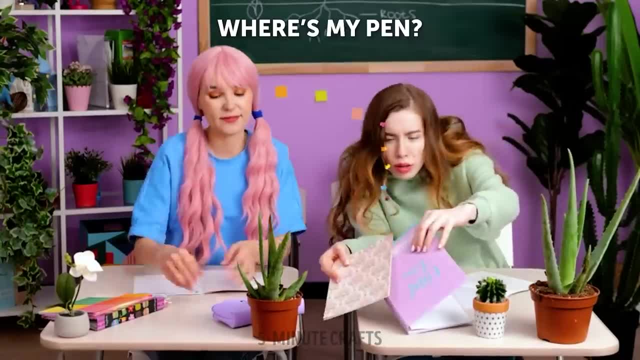 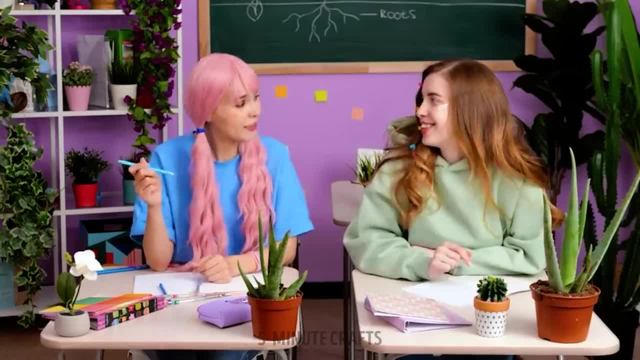 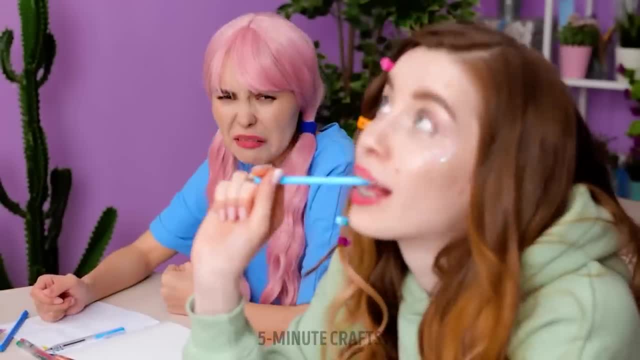 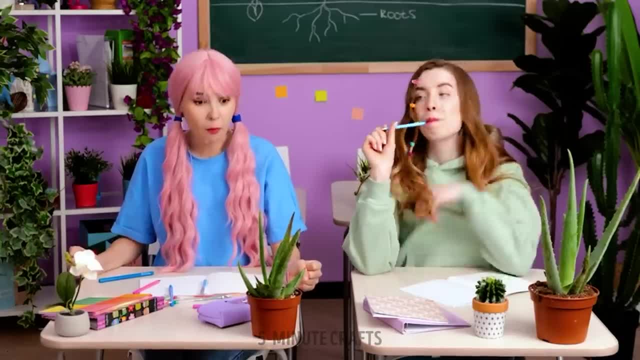 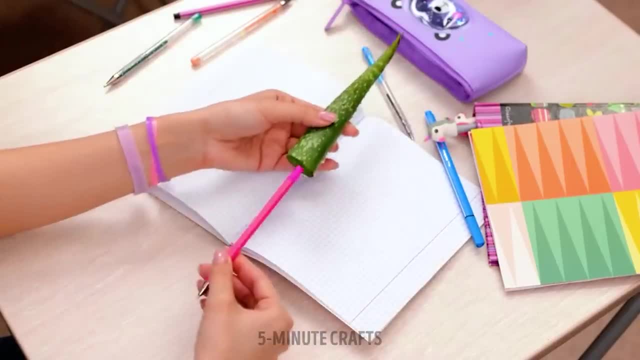 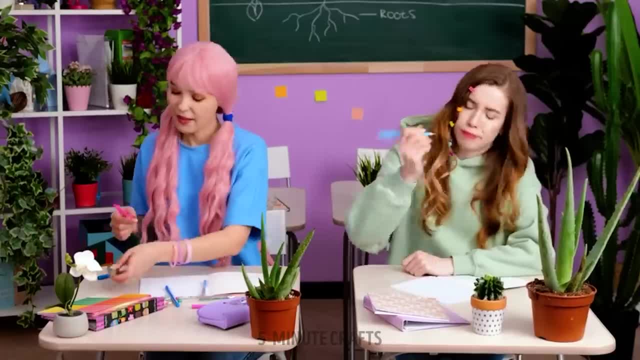 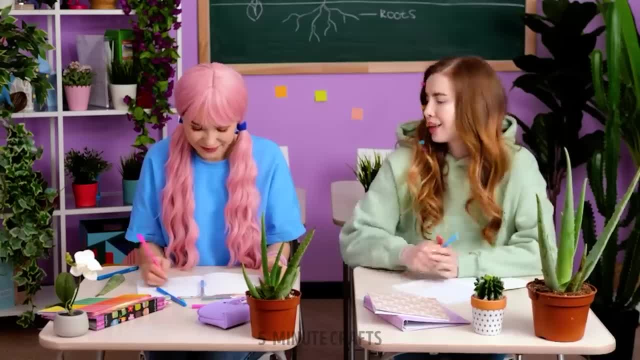 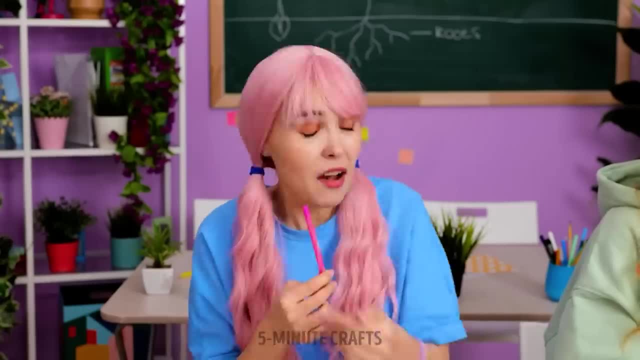 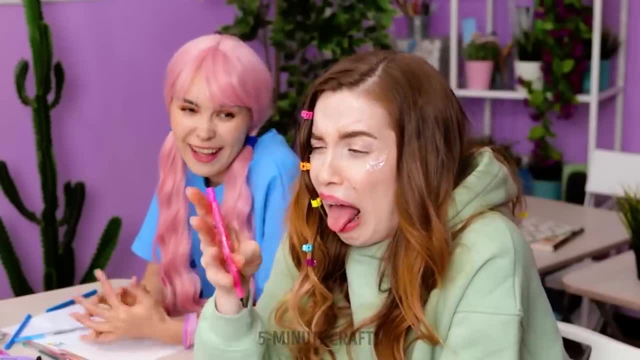 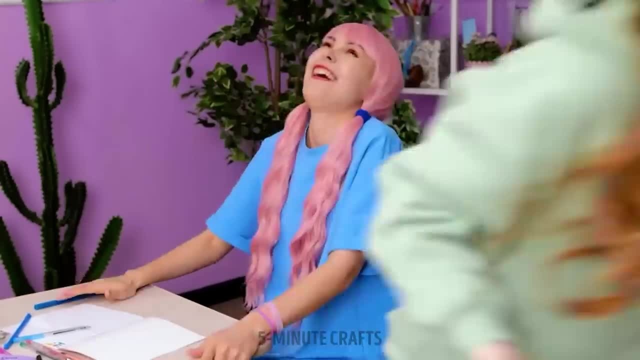 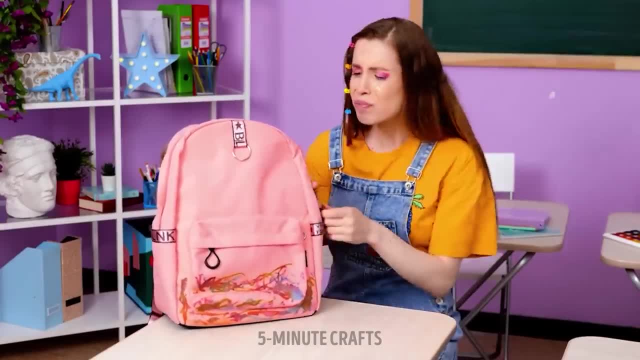 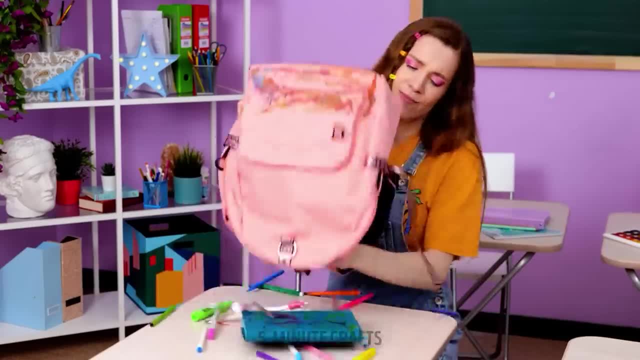 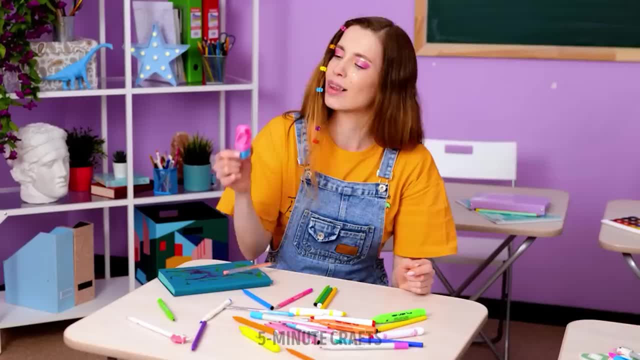 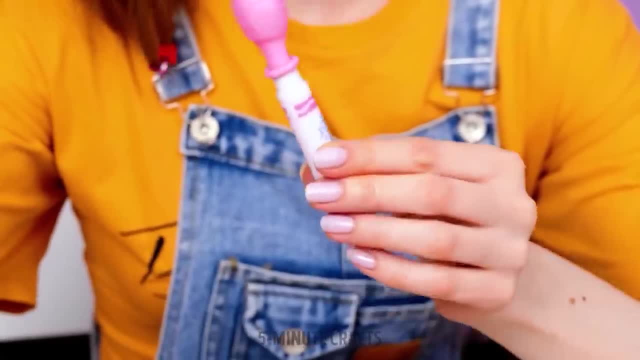 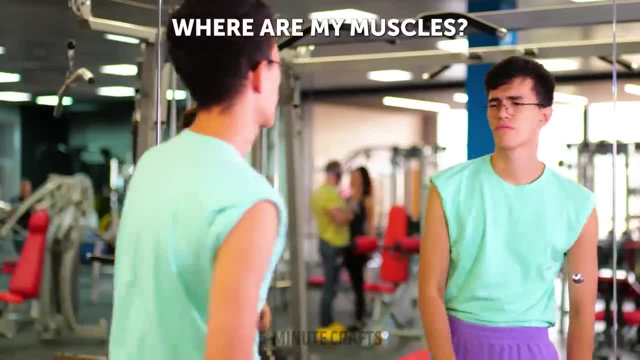 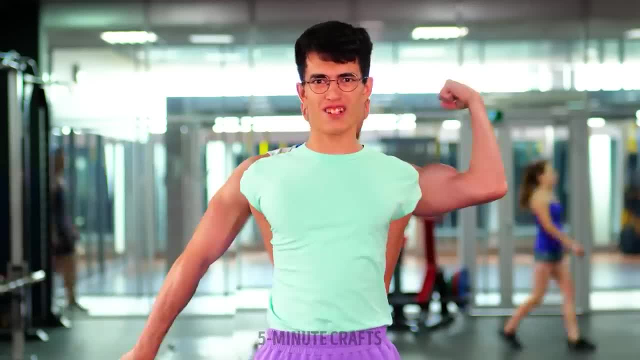 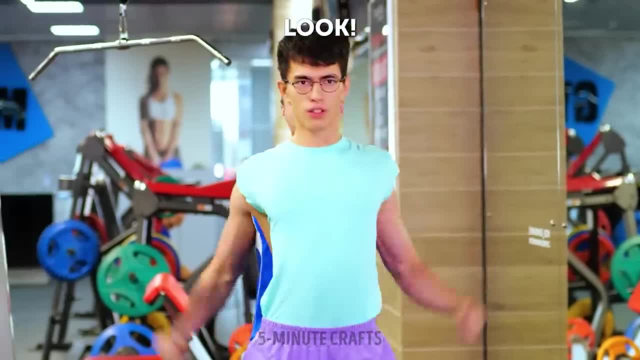 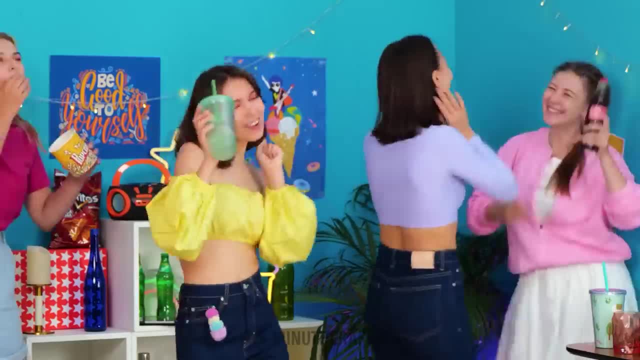 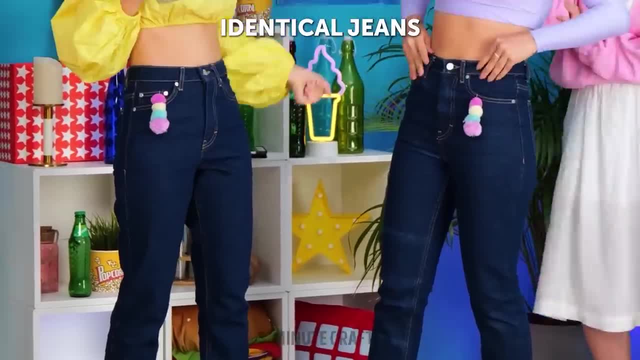 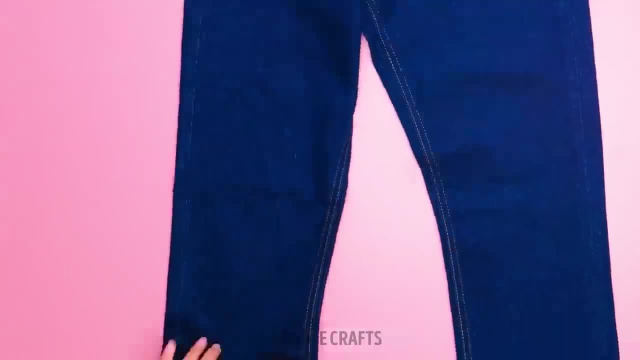 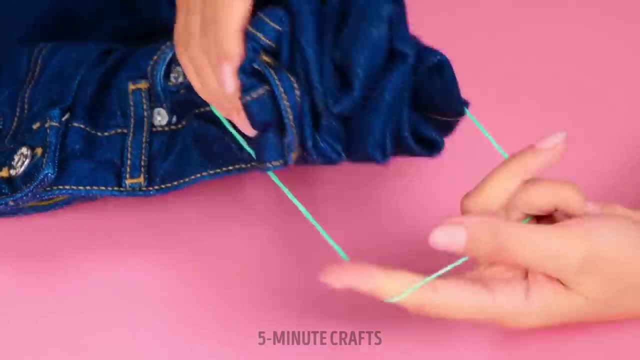 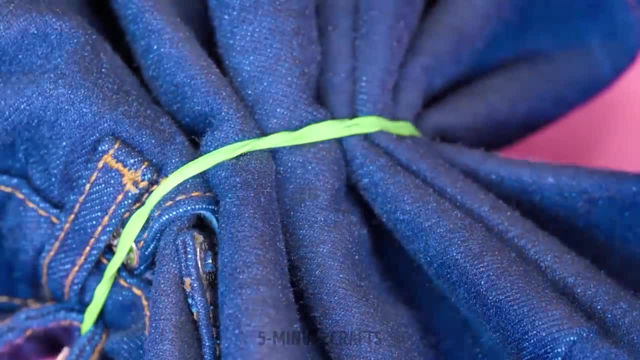 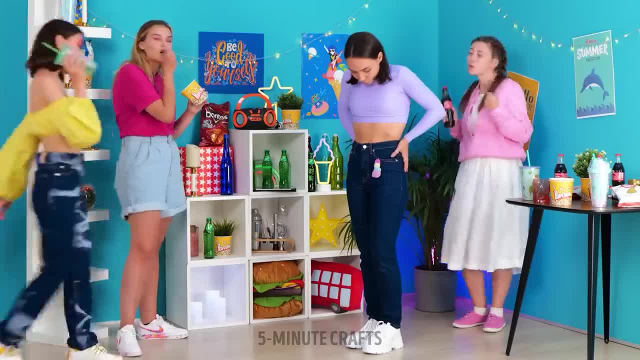 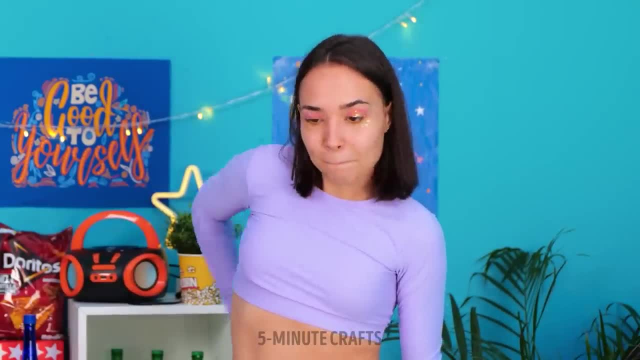 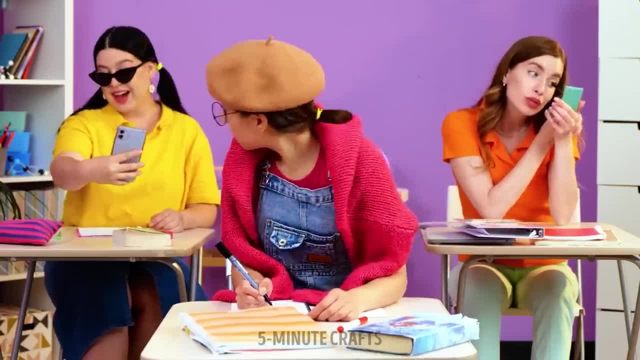 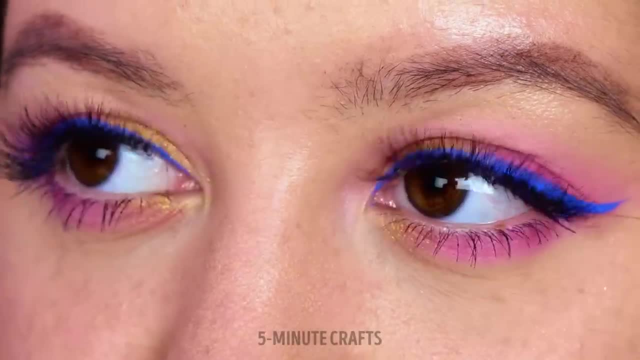 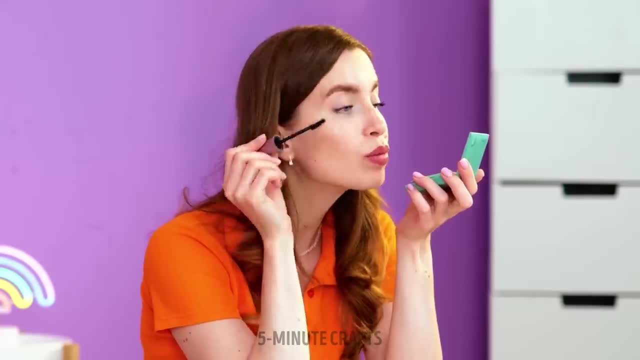 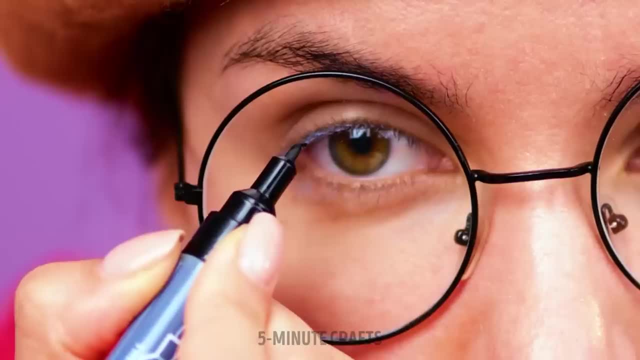 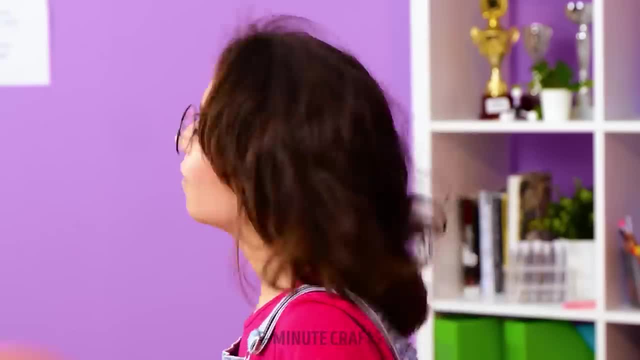 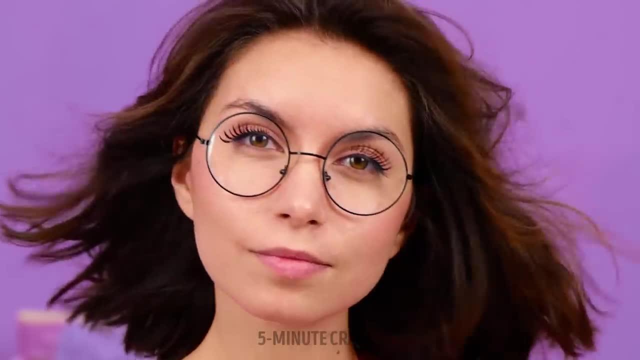 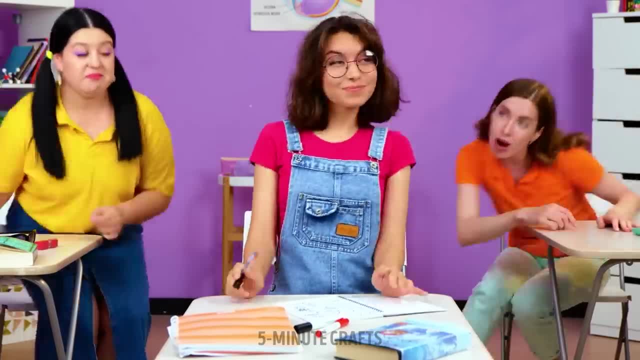 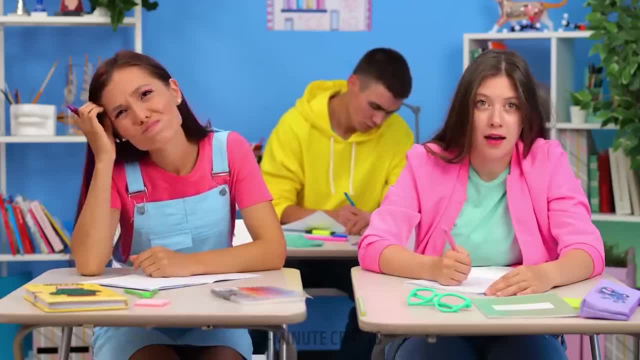 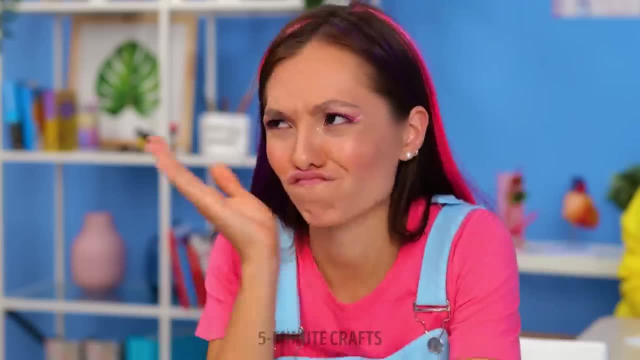 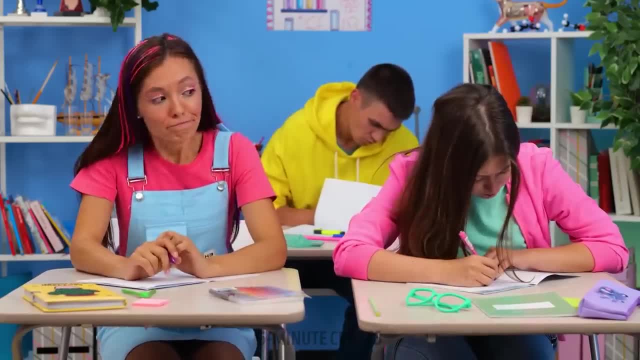 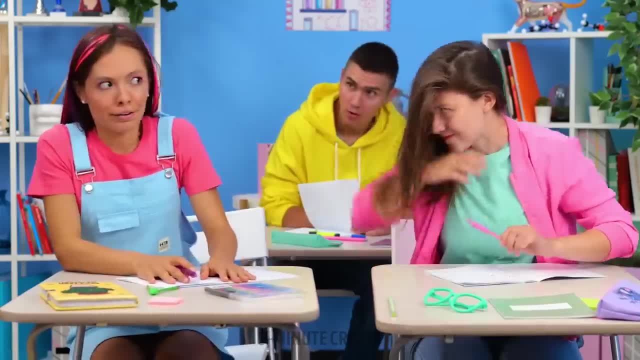 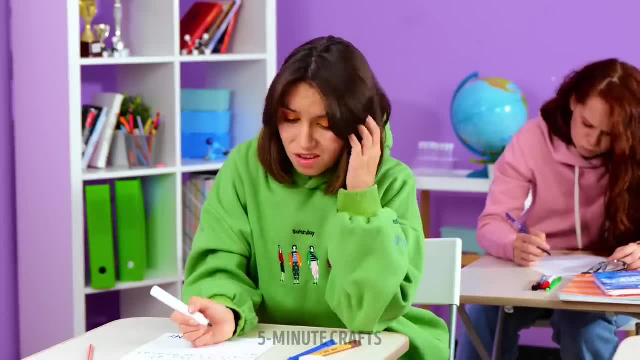 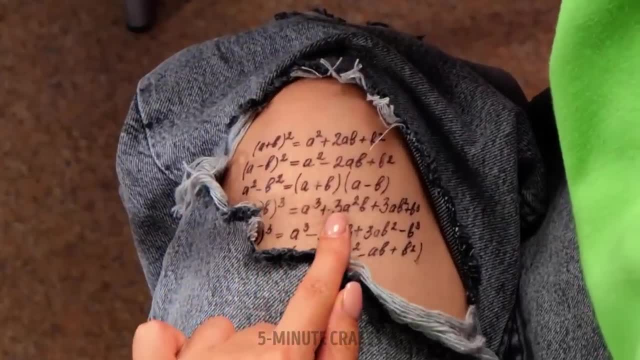 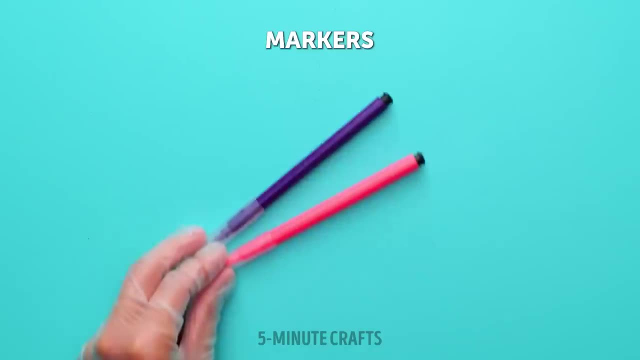 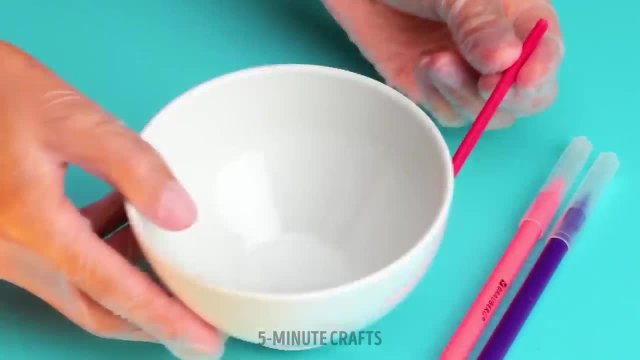 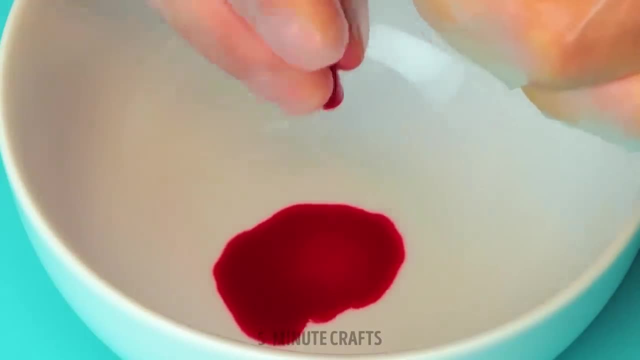 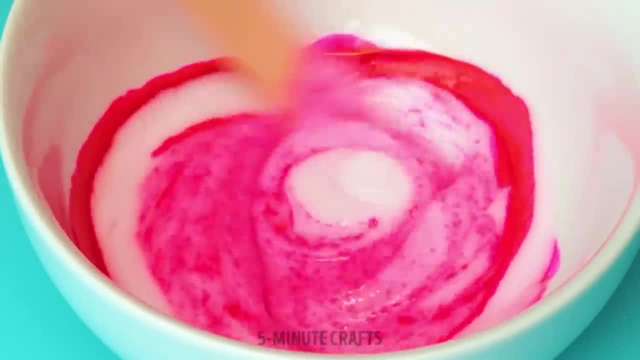 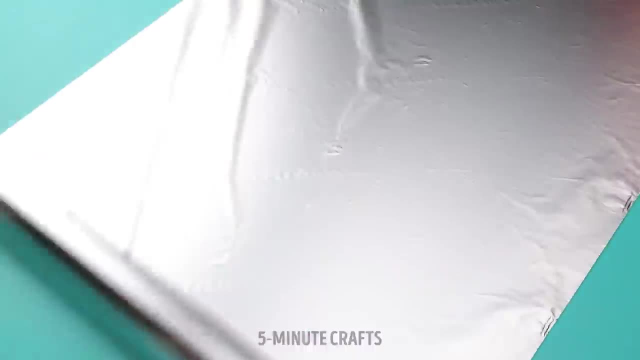 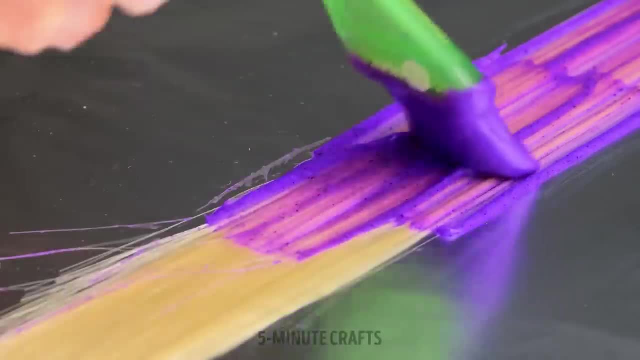 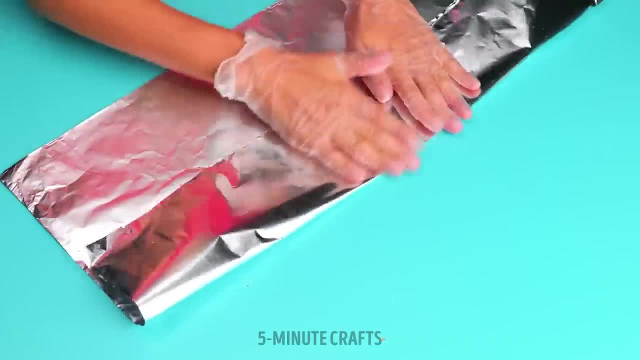 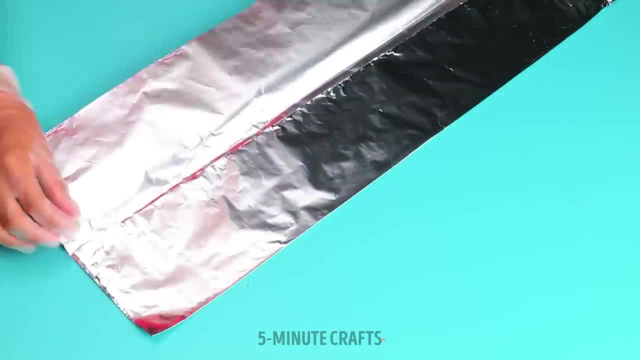 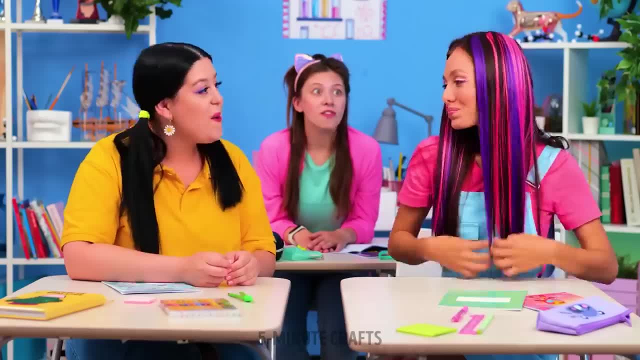 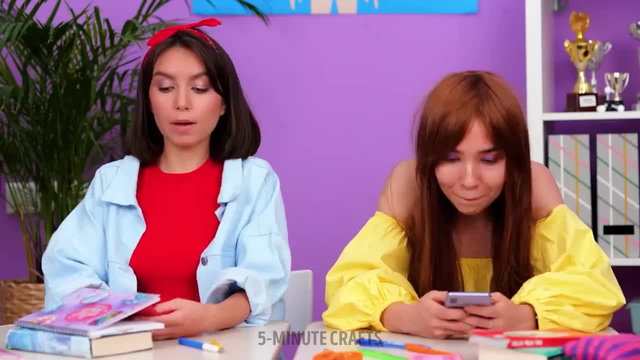 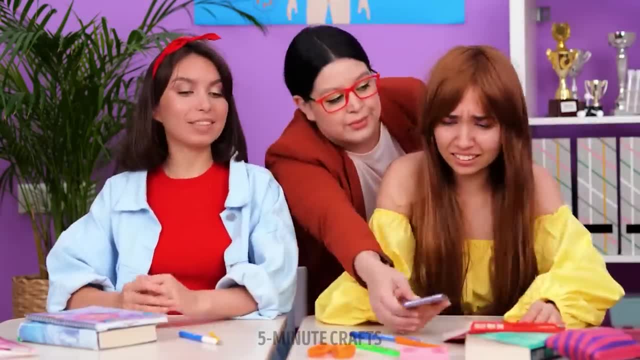 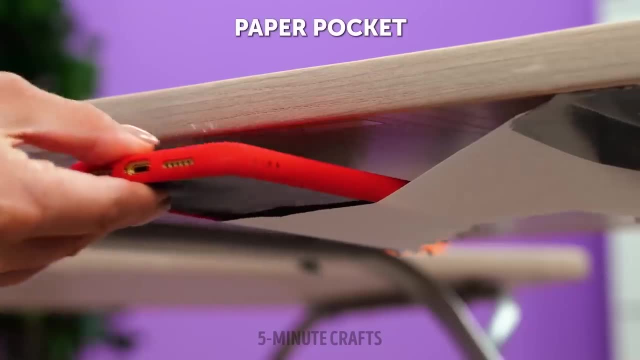 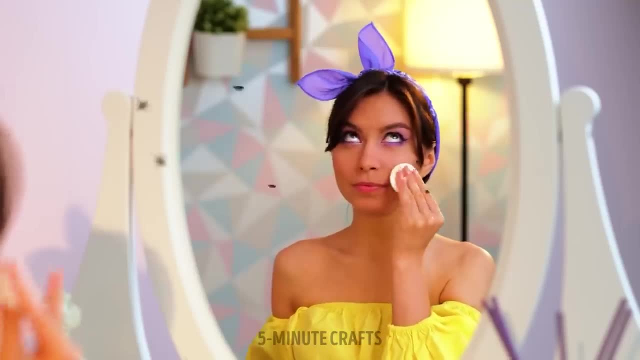 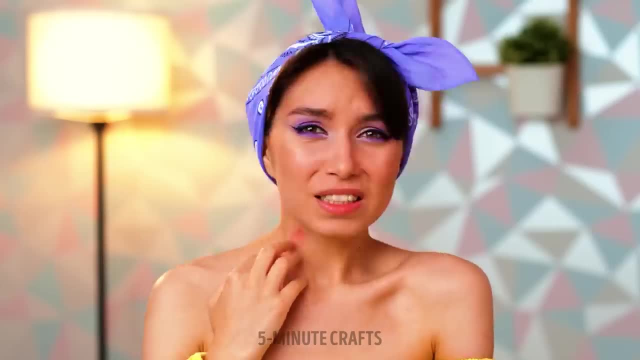 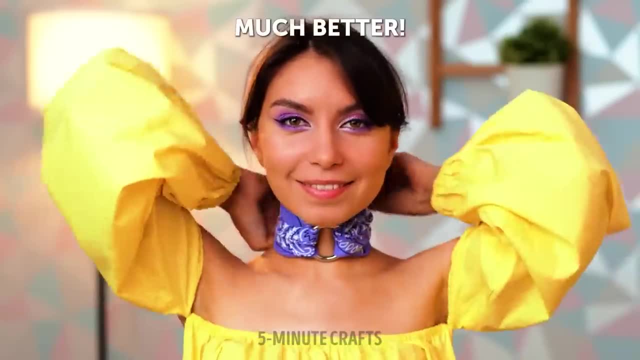 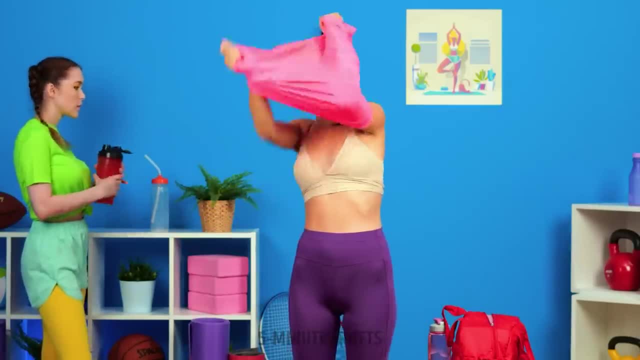 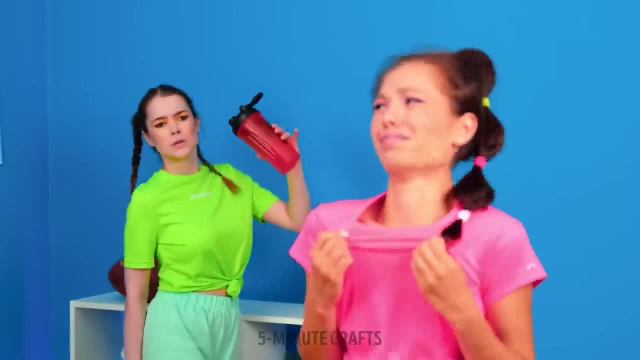 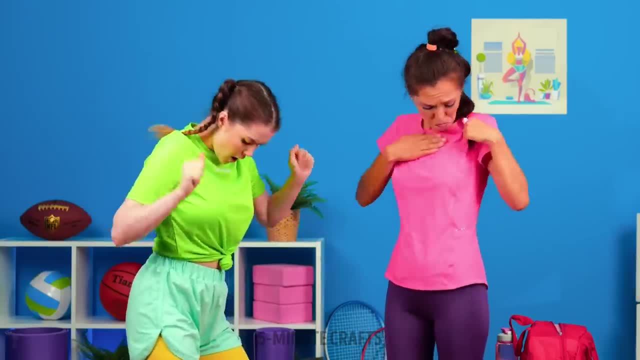 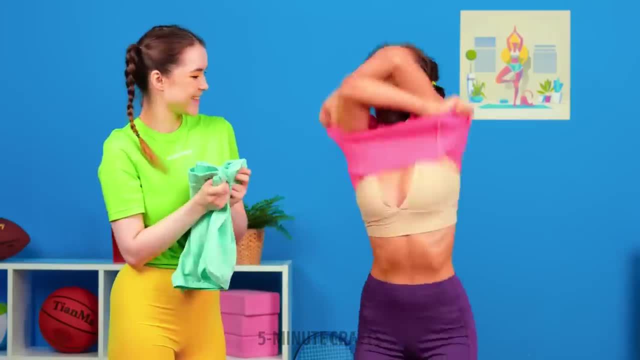 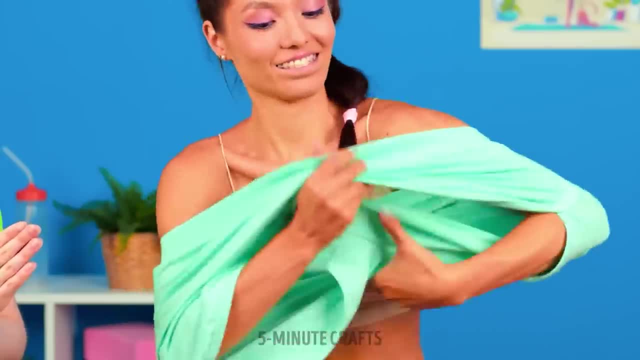 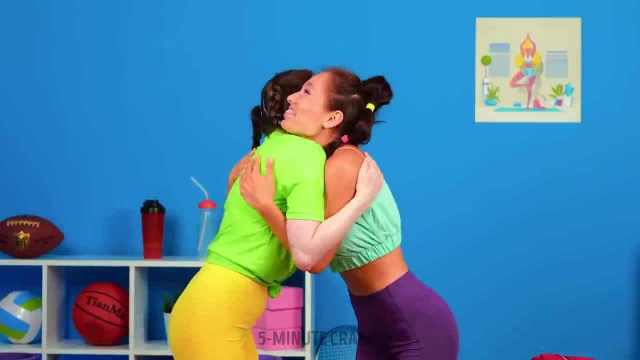 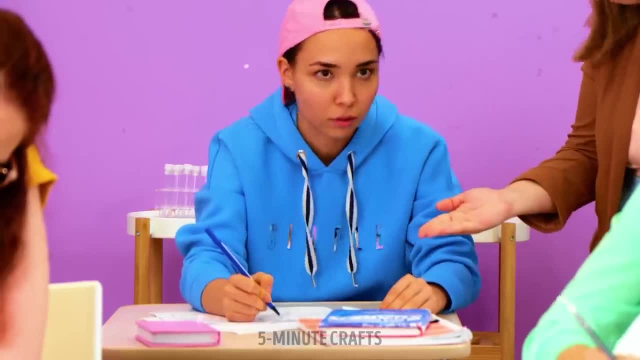 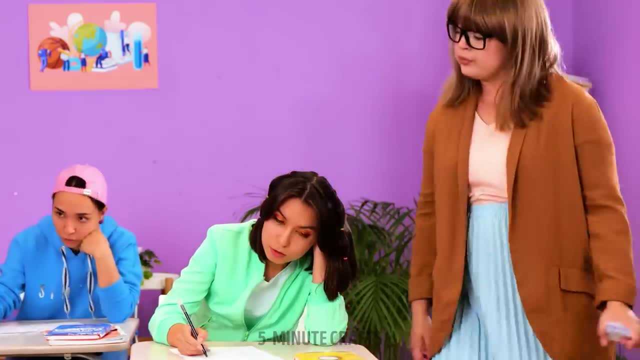 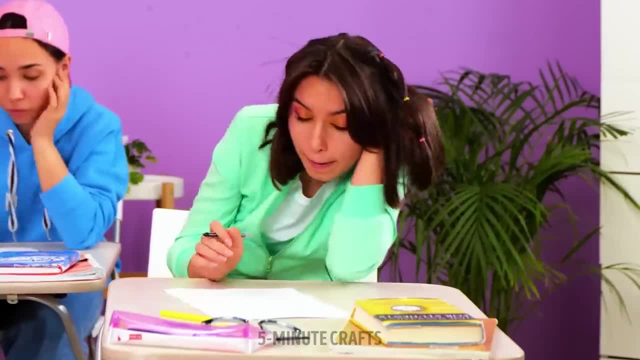 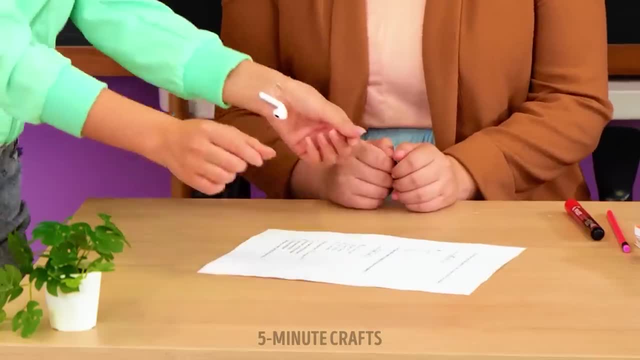 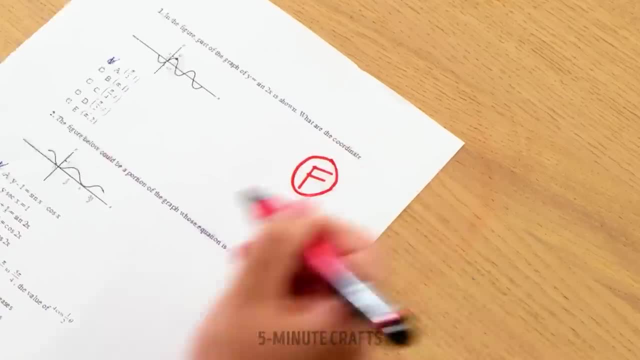